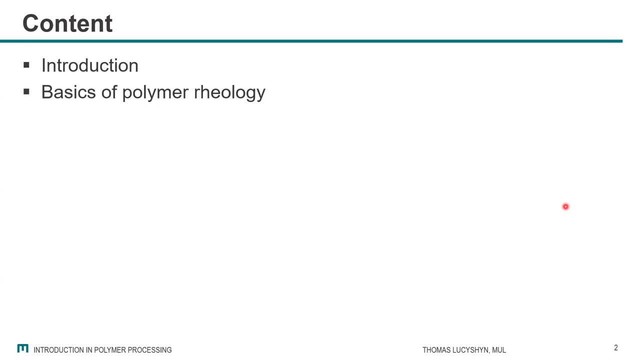 we're focusing more on the material, on the polymer, how it behaves in processing. Then it comes to the major part of this, really: principles of polymer processing, the different processing methods and the products that are produced by. that is starting from extrusion: pipe extrusion, film extrusion, then blow molding, thermal forming, injection molding. 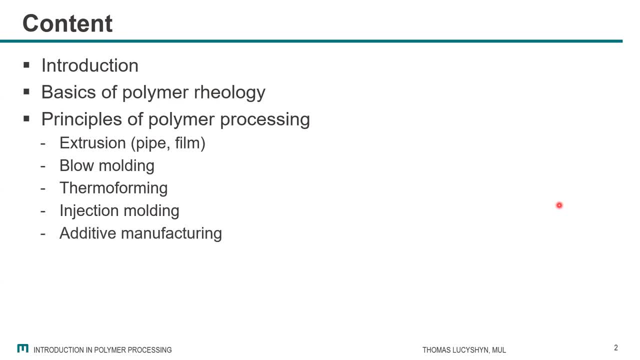 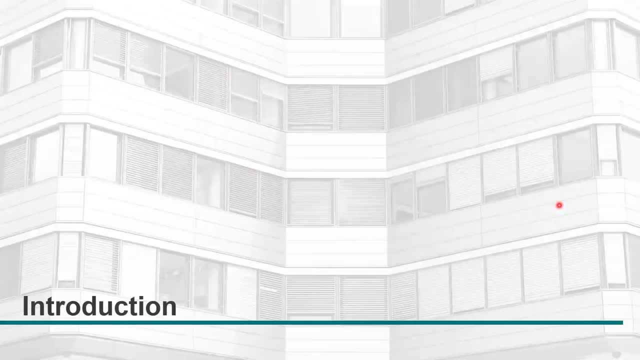 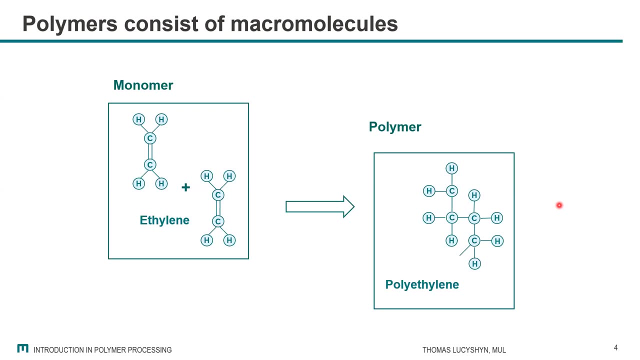 also, of course, recently very strong developments in additive manufacturing. At the end I will summarize and give some conclusions. Let's start with an introduction. We heard that already in the previous lecture, so I don't have to tell about this. We have polymers consisting of macromolecules which are built up of different 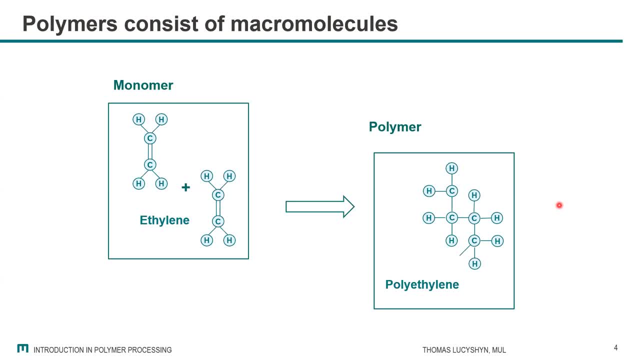 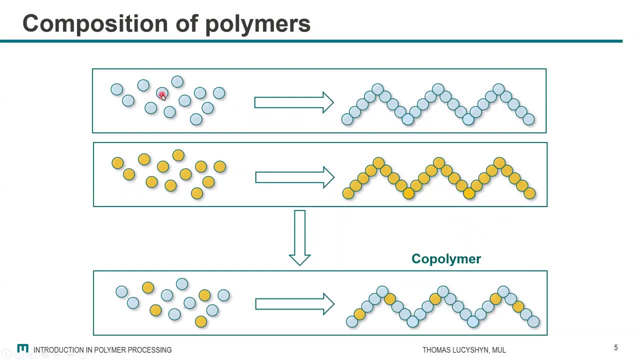 monomers and then creating those nice polymers. We have long, very long chains. This other picture demonstrating this: Depending on the Lego bricks, if we have different Lego bricks and based on how do we assemble them, we get different polymers with different properties and we have different 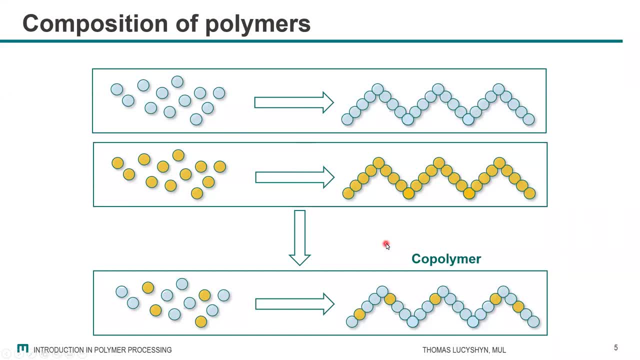 colors We get different properties and then we're using co-polymers mixed the properties. so There's a huge variety of polymers and property profiles which we have. That also has an influence on the processing conditions that we need. It's still important to know these long molecular chains have also some influence on the 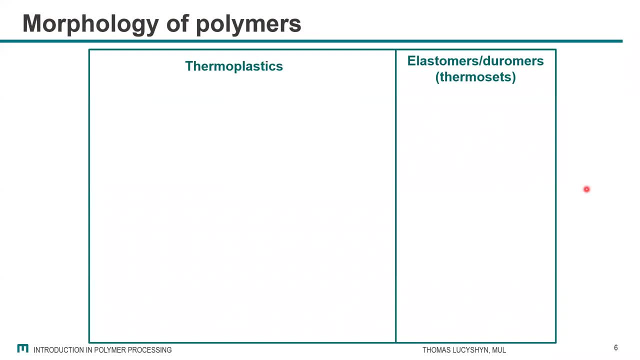 material flow behavior. Also, the morphology of polymer is relevant and necessary, also the also in terms of processing, from the processing point of view. So we had this already in the previous lecture. We have, on the one hand, we have thermoplastics. 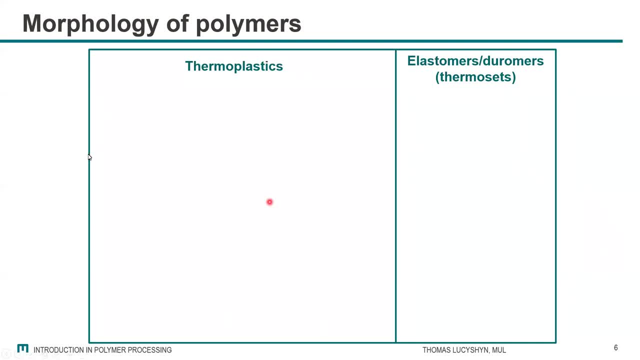 And on the other hand we have so-called thermosets, which are like elastomers and duramers. The thermoplastics can be further distinguished between amorphous materials which have this very unstructured state. So all those molecule chains are entangled but not cross-linked. 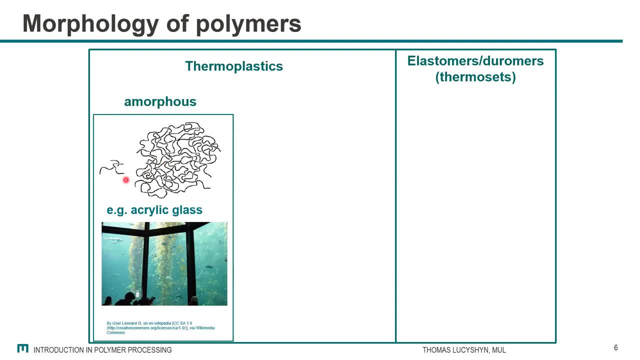 So that's important. So they are basically not chemically bound but just physically entangled, And one example of that is acrylic glass, for example. So amorphous materials are typically also can be transparent, Whereas semi-crystalline materials. 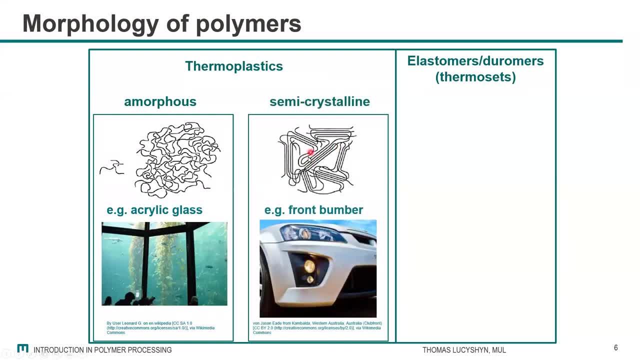 parts of the molecular chains are able to arrange themselves in crystalline structures, But not all of them. So you will not find a polymer with just perfectly crystalline, So therefore we call them semi-crystalline. You will always have some imperfections within. 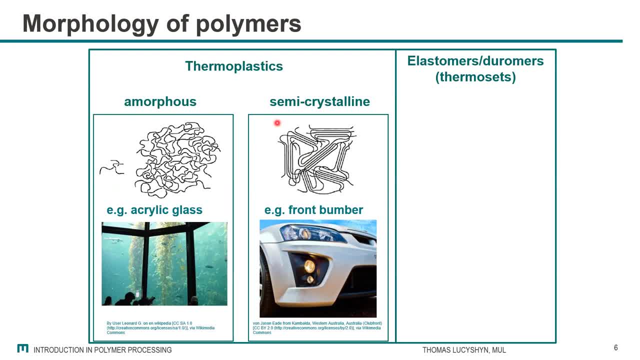 and that are those unstructured amorphous phases within those crystallines. One example: All these typical applications. the mechanical properties are typically better for or very good for semi-crystalline materials And typically they are not transparent. So that's the thermoplastics. 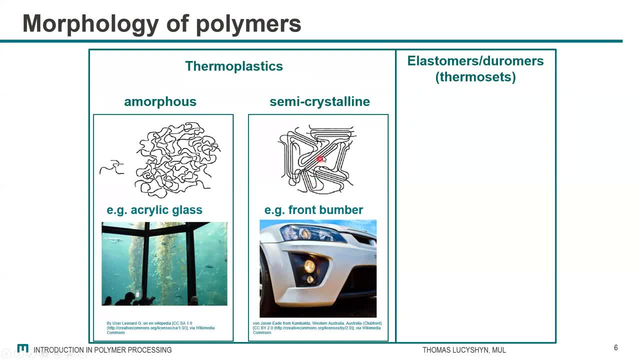 Once again, the main point is that they are not. the chains themselves are not linked to each other in a permanent link, Whereas for the duramers, or elastomers, or thermosets, as they are called, we have cross-links, chemical bonds between the molecular chains. 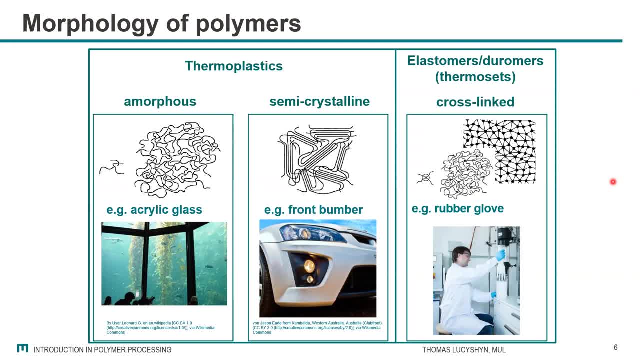 And depending on the number and density of those bondings we get different properties. So if we have very few connecting points, then it's quite an elastic material behavior And we have rubber basically. So it's like this rubber glove. 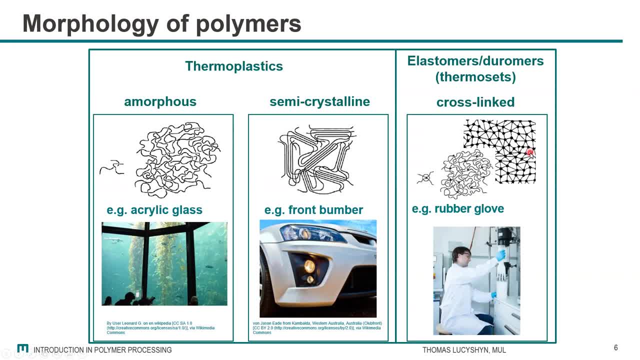 And, on the other hand, if we have very tight network of connecting points, then it becomes increasingly rigid, And we have really those very hard and rigid materials which are also quite temperature resistant, And these different morphologies have also an influence on the processing. 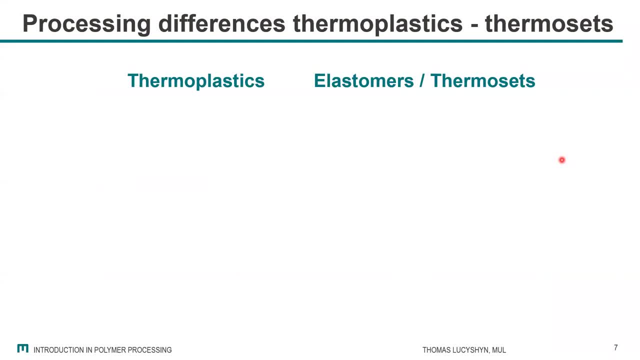 and also, furthermore, on recycling. So, having a look at the different processing paths of thermonucleotides, we have thermoplastics and elastomers. We have, on the one hand, the thermoplastics, typically starting from pellets or powder, sometimes. 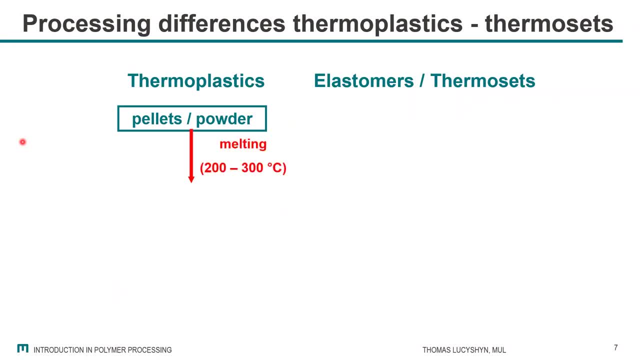 The point is that thermoplastics, as the name says, we have to heat them to melt them. Then they become plastically deformable, So we have to melt them. A typical processing range is in the range of 200 to 300 degrees C for most of the polymers. 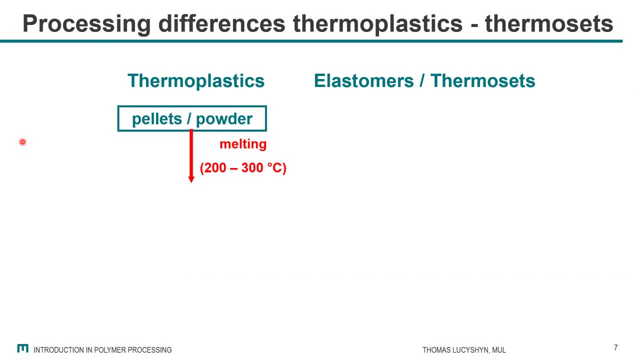 There are, of course, some at lower temperature and also goes up to 450 degrees for some specialties, But still the majority of polymers will be processed in this range In the melt state. we can then shape the material into the desired shape. 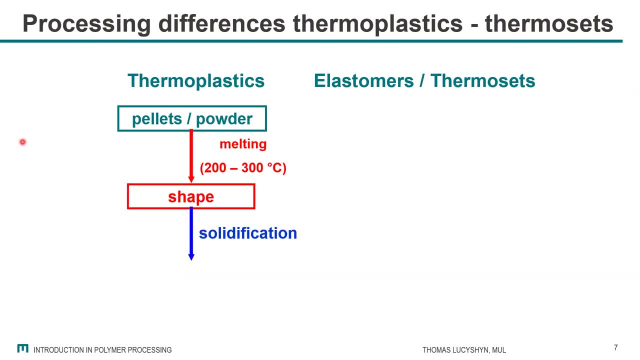 And then finally, we have to cool it down. We have the solidification of the melt and we end up in a product. The very, really nice thing about thermoplastics is that this process is reversible, So we can remelt, reshape and create a product. 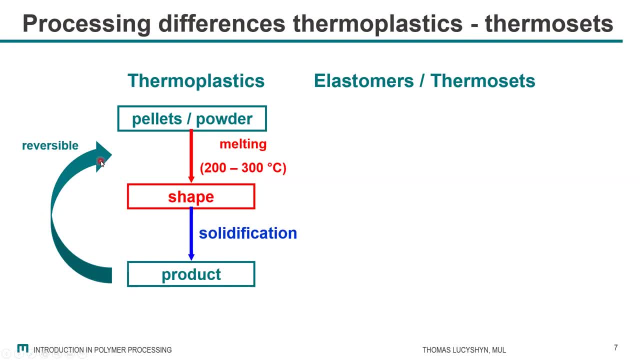 Of course we are losing properties. So each time we are doing this there is some damage done to the material, because the relationship between heat and polymers and heat is an ambiguous one. We need the heat to shape it, But on the other hand, heat causes some damage to the material. 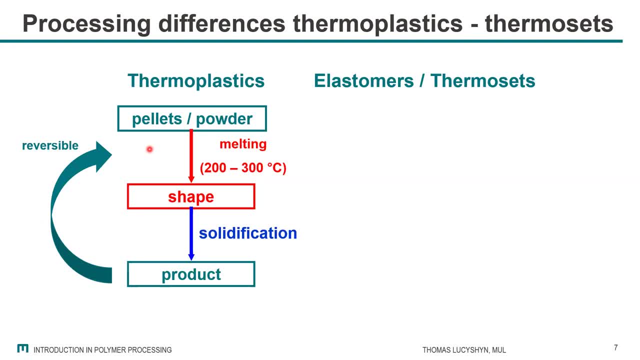 So we have to find a compromise of not too much damage but still getting nice processing conditions. On the other hand we have elastomers or those thermosets. We start with the rubber or liquid state and typically the shaping happens in the cold stage. 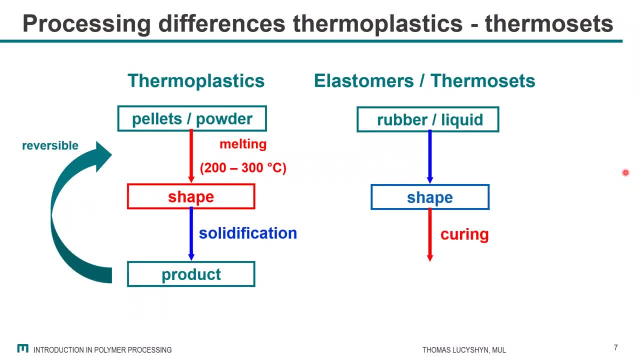 So we were still cold, and then heat is introduced to trigger the chemical reaction of the curing. So this cross-linking, this chemical reactions of cross-linking, It's happening by introducing heat and then the product is finalized. And here the problem is that is typically not reversible. 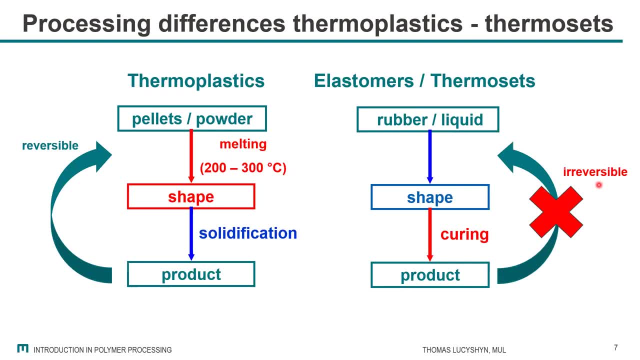 So it's irreversible. So once you have your product which is cured, you cannot just kind of remelt it as you can do with thermoplastics, which is very important to know regarding recycling opportunities, especially mechanical recycling. So typical thermosets are not the champions for mechanical recycling. 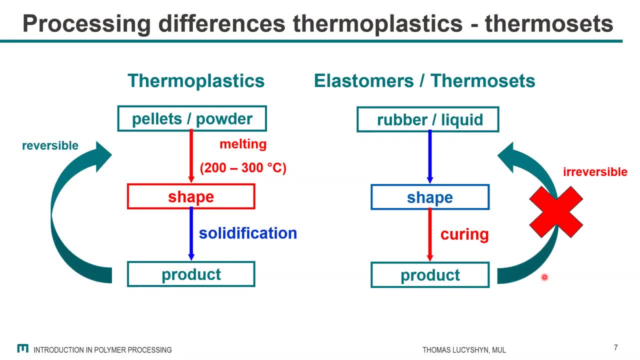 So you will not be able to use it for mechanical recycling. There are some developments, Although for like Vitramers which are kind of deformable one more time, but still the majority of the thermosets cannot be really mechanically recycled. It's important to understand. 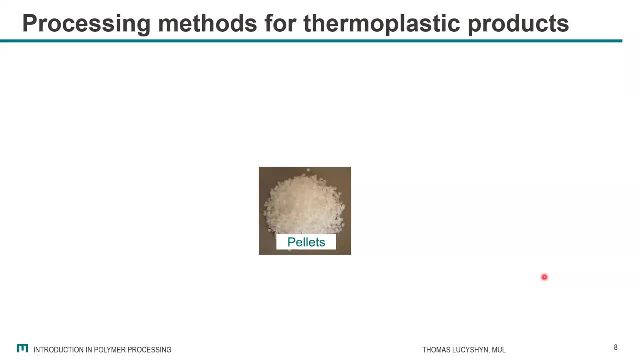 What can we do? So I'm in my presentation. I'm basically focusing mainly on thermoplastics, So not on the elastomer side and the rubber side. So we are typically starting from a pile of pellets and based on the different processing methods. 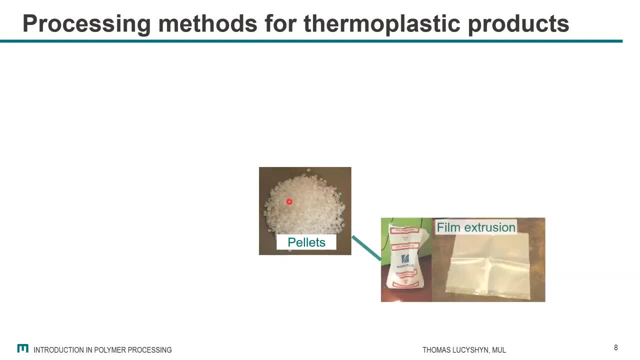 we can produce different products from these Pile of pellets. So it could be film extrusion on the one hand, like bags or some standard sheets. On the other hand there is profiles or pipes or window profiles, pipes for sewage, whatever. thermoforming is another method where you would typically produce packaging goods. 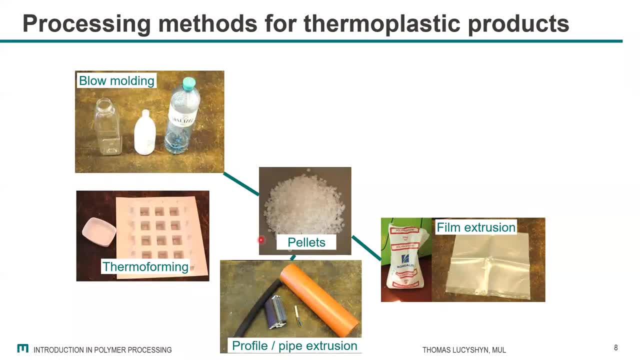 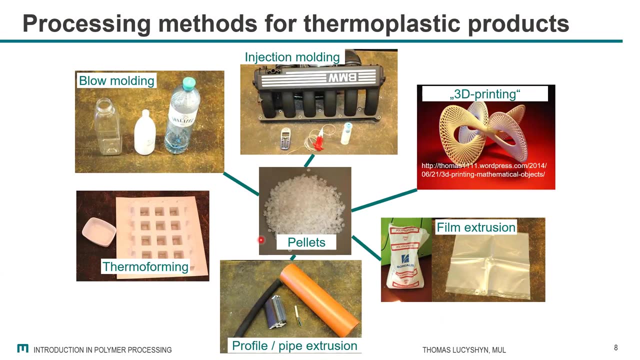 Then we have all those hollow bodies produced by blow molding and injection molding is for mass production of complex single part. So so, not continuous Products like pipes, but single parts. and then recently, of course, for crazy, weird geometries, We can also use 3D printing, which cannot be achieved by the other conventional methods. 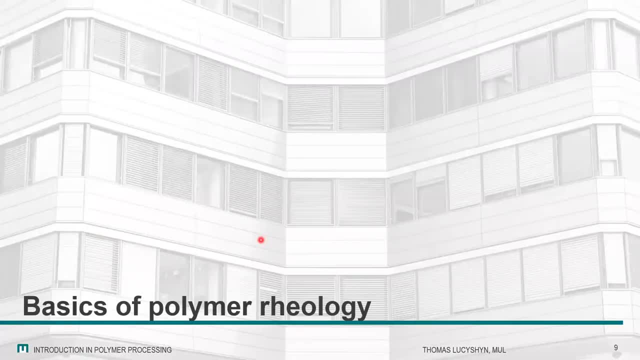 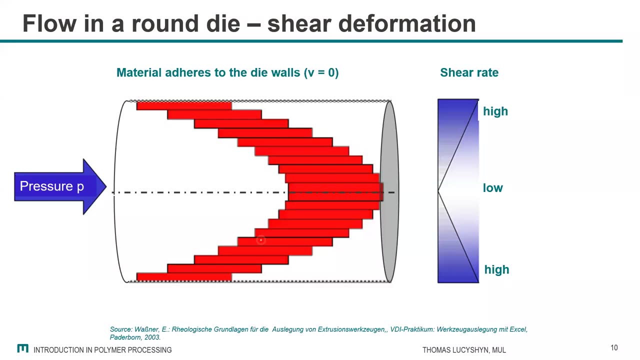 Before I go into the processing methods, I would really like to talk a little bit about basics of polymereology, And for that purpose I would like to first introduce a little bit of an understanding of what how polymer is flowing in a processing machine. 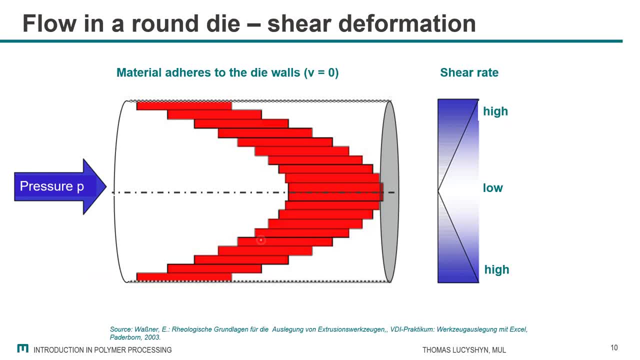 So we are assuming we have a a polymer melt and we are trying to pump this polymer melt through a channel. Now we are looking here currently at a cylindrical channel like a pipe, And then we typically have this flow pattern so that typically polymers are adhering to the wall. 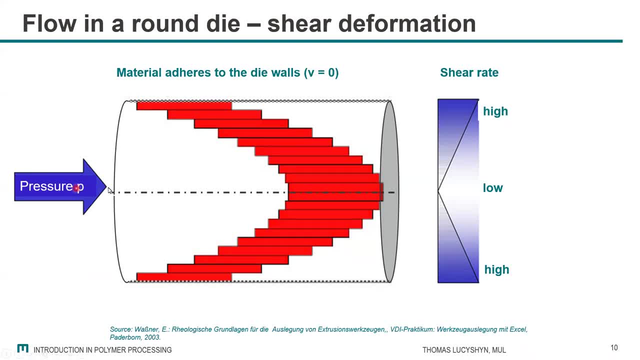 That means they're, they're sticking to the wall basically, And material, if we apply some pressure goes there with the maximum speed in the center. So we typically have this parabolic velocity profile of the maximum speed of the melt flowing in the center and then zero velocity on the. 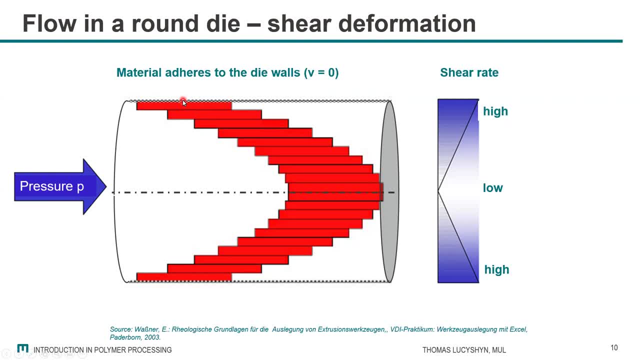 on the surface And this different velocities within this channel result in a in a shearing between single layers. So if you have, if you imagine this, this whole material split up into single layers of material, just for a model, then you can see that, for example, in the center line 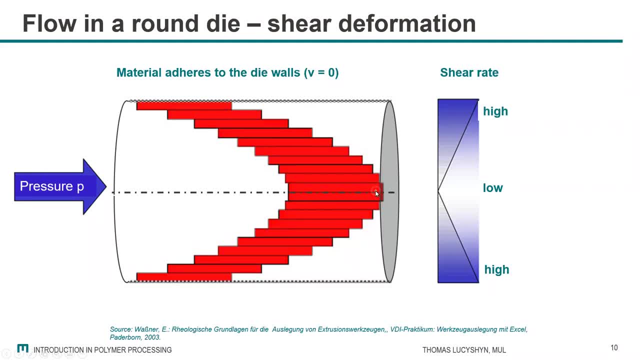 due to the symmetry, those two layers to two neighboring layers move at the same speed. So this, this bars represent the speed, So they have the same speed. So that means between them there is no shearing because they move at the same speed. 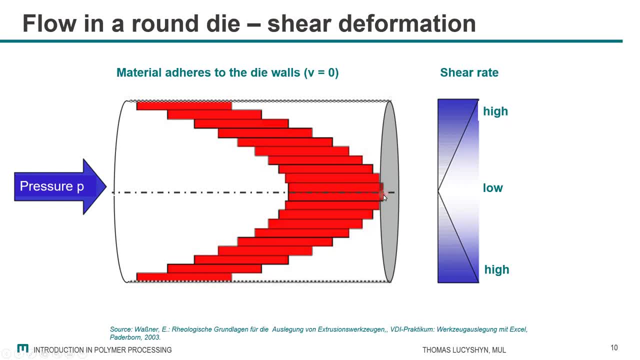 There is not a different speed And that means in this stage our macromolecules are staying in this quite unstructured state, in this entangled state, because the molecules are not oriented And, as you can imagine, just a plate of spaghetti If you try to pull out single threads out of this pile of spaghetti. 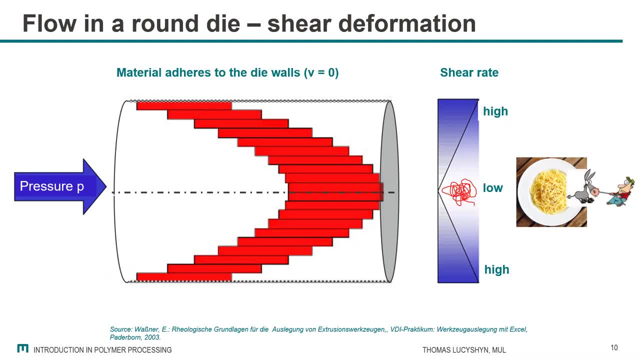 which are quite entangled, it's very hard to get them out. So here the flow ability of the material is quite bad. It's quite a high resistance against flow Because they are quite entangled. What is happening If we are moving towards the surface here? 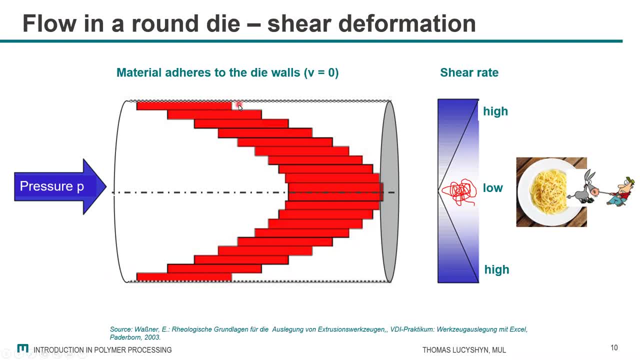 we have a big difference in velocities between two neighboring layers. So that means that this layer is the surface- is a zero speed and this head is higher speed. So that means in between we have kind of can imagine- like friction If two bodies are moving at different speeds and touching each other. 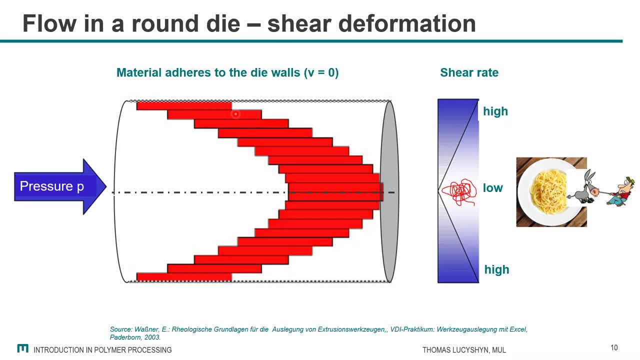 we get some friction in between them And with this friction we call shearing in the melt state. And what is happening in this, in this, in this area, is what? imagine: you have a polymer molecule which is oriented in this way: 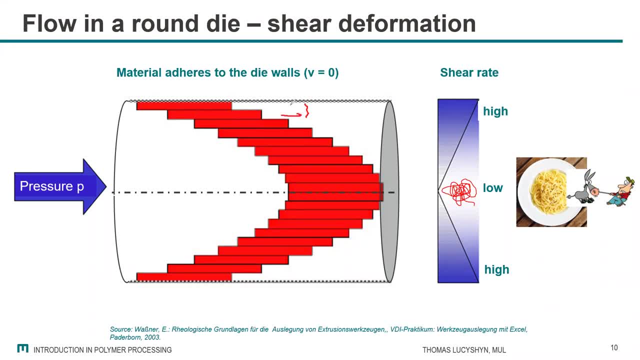 And now in this layer the speed is higher than in this layer. So that means that this part with the higher speed is orienting the molecule in this direction, because here it's moved faster. So in the end the molecule gets oriented in the flow direction. 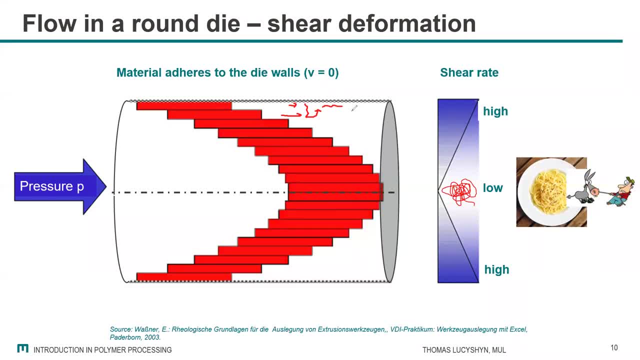 So that means in general in those layers close to the surface the molecules are getting oriented and also a little bit disentangled. So in the end you end up in in layers where the molecules are more aligned to each other, which means also it's much easier to pull out or to move them along each other. 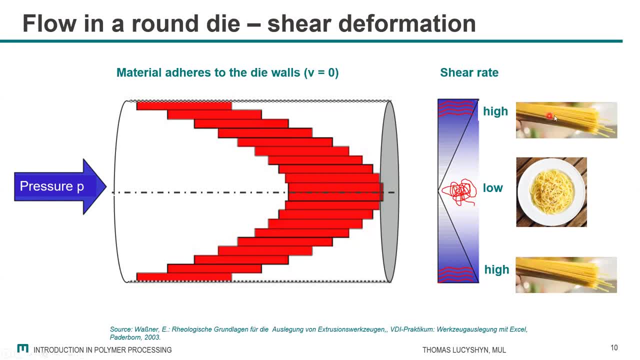 It's like now, the spaghetti in the package. they're not entangled there. You can easily pull it out. So it's in the layers to the surface. It's quite easy to pull them out And this whole phenomenon we are describing is so-called shear thinning behavior. 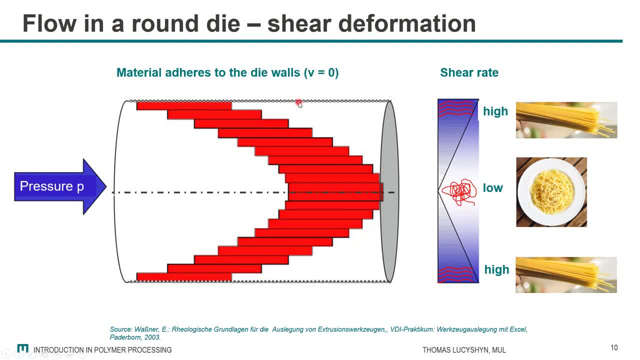 So with increasing shear which are applying, the material gets thinner. It means basically the flow resistance becomes lower. It's easier flowing. I will come to that in later slides as well, I would look. I would like to share a few equations. 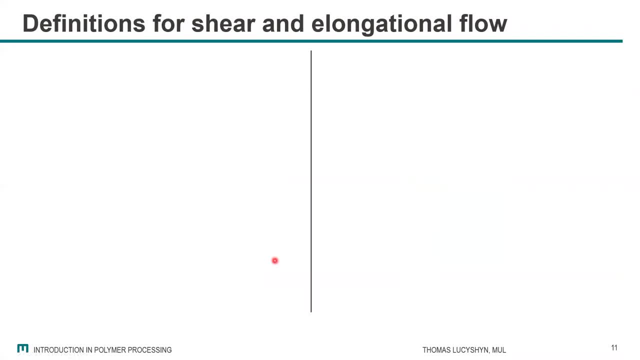 So I promise this is the only slide with a few equations, So I won't confront you with our beloved conservation equations. So this is really, I think, accessible to anyone. So let's have a look. also, distinguish between shear flow and elongational flow. 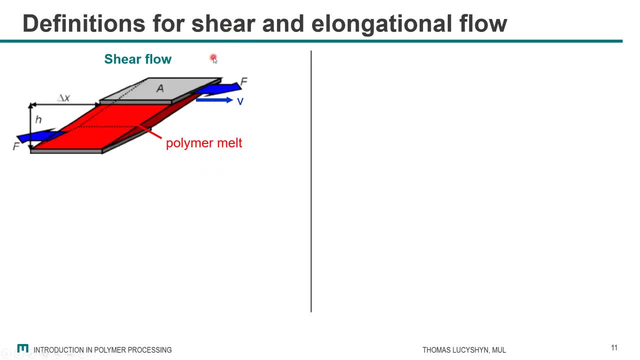 Shear flow is basically happening in like in extrusion or in injection molding, whereas elongational flow is a topic for a blow molding or other process where you, where you stretch the material. So let's have a look at shear flow. 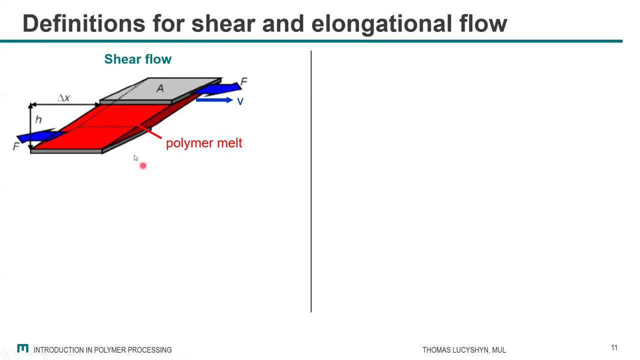 Have a look at a very simple experiment. So we are starting with the two plates- The gray ones are two plates- And then in between these two plates we have a polymer melt, which is this red one. The starting point would be that we start with a straight cube. 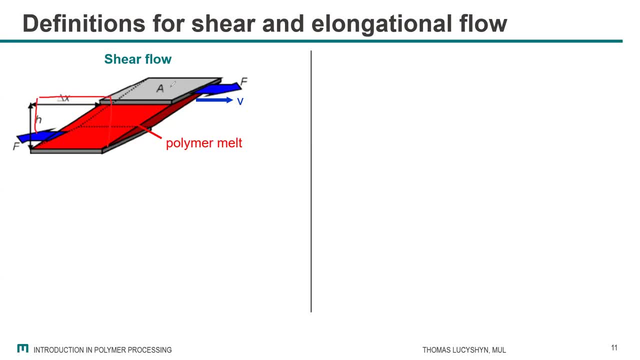 So we start with a straight cube of cube of material And then we are starting to pull those plates with a certain force, F, and a certain velocity V. So we pull the for the plates And the result of this pulling is that the polymer melt gets deformed. 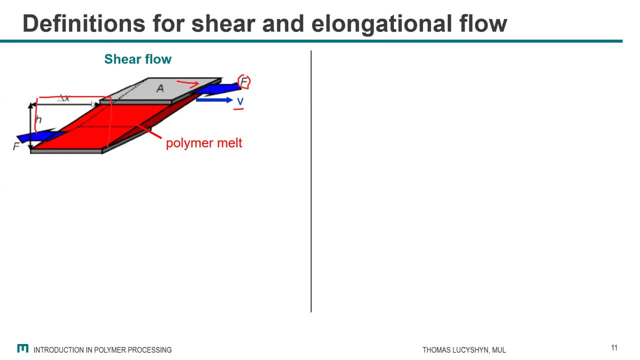 And this deformation is expressed by this Delta X. So this is the amount of deformation that is happening relative to the gap. height is the distance between the two plates, And then we can define certain terms and values which are frequently used If you're talking about polymer pressing, processing, 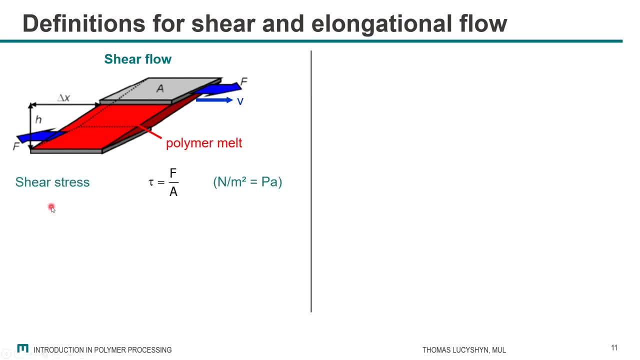 you will come across those terms- That's, on the one hand, the shear stress acting on the fluid. So that's basically, we have to transfer this flow force into the fluid, into to the deformation of the fluid, And this is happening with the shear stress, with the Greek letter. 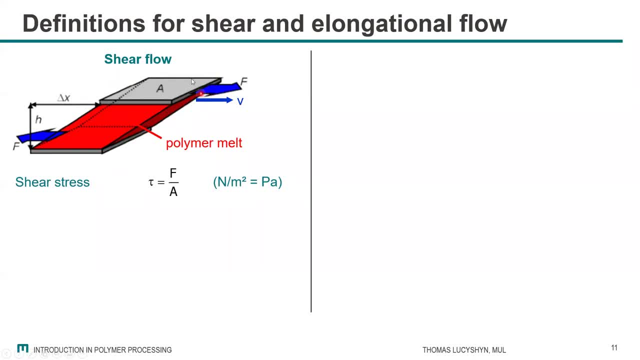 Tau is equal to the force which is applied in this interface area between the plate and the melt And that's the ratio of the force applied on this area. That's the shear stress acting against the force of the of the external force. So we are pulling with the force and the material tries to work against it, with the shear stress acting in this interface. 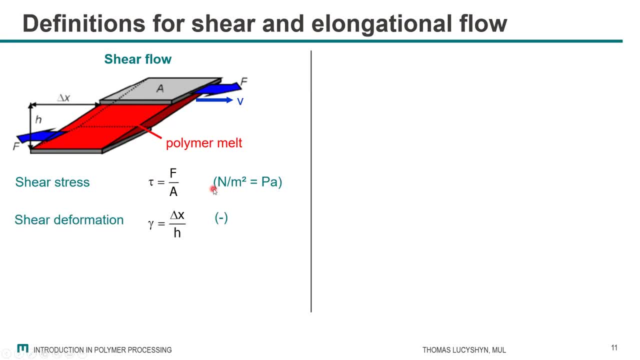 The unit is Newton per square meter or Pascal. Then we can define the so-called shear deformation gamma, which is basically the amount of deformation, Delta X, which is happening relative to the gap height. This is important If you have a very big cube. 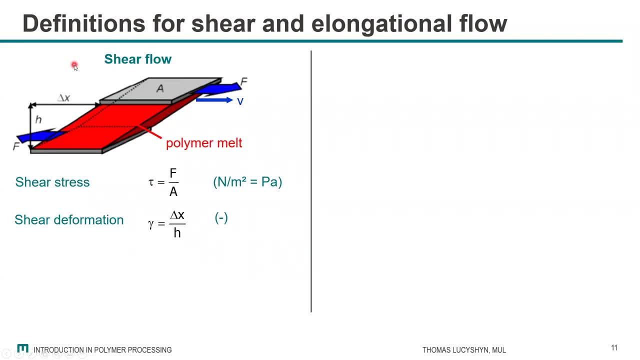 a very big height and a very small Delta X, then the whole deformation is quite small. So just to show it: if you have a very big cube and you deform it by a small Delta X, then the whole cube will just deform like that. 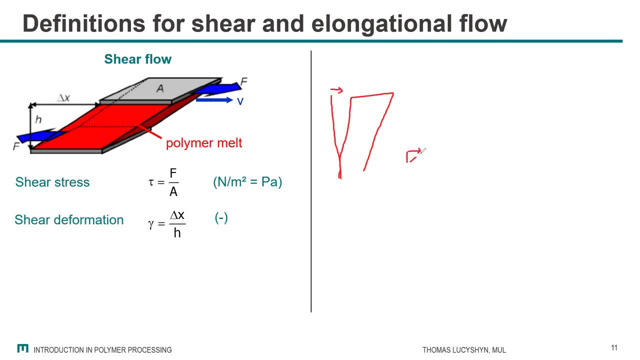 If you have a very small gap and you deform it in the same way, then the deformation is much bigger of the cube. So that's really makes a difference how big the height is compared to the deformation which is happening Next. the shear deformation is one thing. 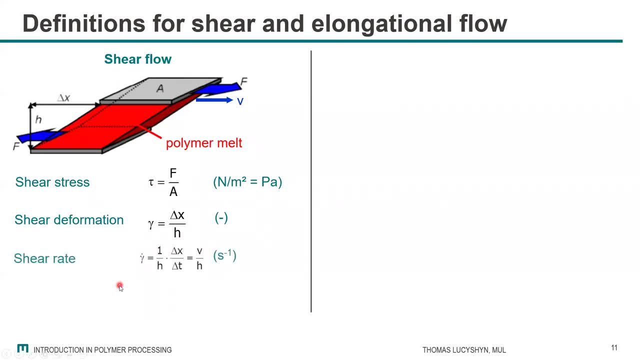 It has no unit because it's meter by meter. And then the next important thing, next important term, is the so-called shear rate. Shear rate is just meaning how fast is the shear deformation happening? The dot, the gamma dot, just indicates is a change. 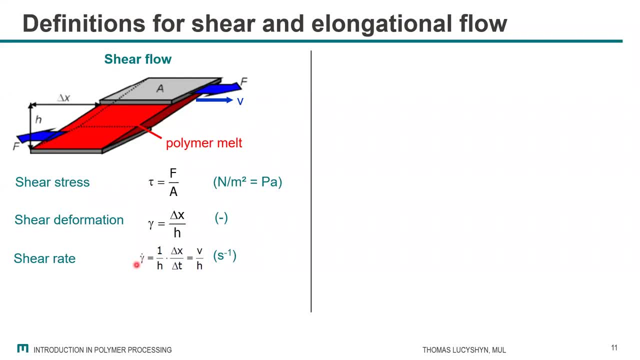 a change of deformation with time. So dot indicates a change with time. So deformation happening within a certain time step, Delta T. So what we write here is Delta X by H is the deformation divided by certain time steps. So how much deformation is happening during a certain time? 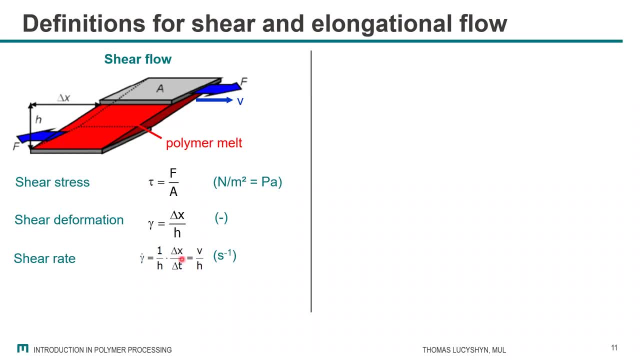 And we can rewrite this by Delta X. but Delta T is just distance per time, is meter per second, is the velocity. So in fact the shear rate can be defined as the velocity, the speed of the flow divided by the gap height. Here, 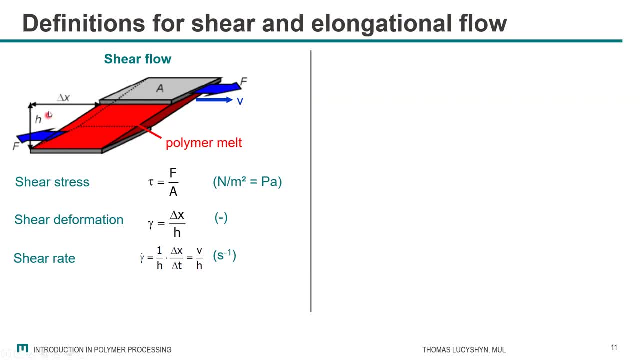 the same. if we have a very wide gap, a very high gap, there will not be too much shearing at a certain speed. If we have a very small gap, then there will happen a lot of shearing inside material which also causes some heat introduction. 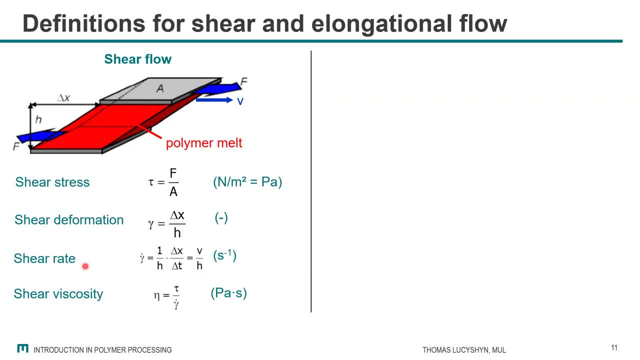 And finally, we have a combination or a relation between the shear stress and the shear rate and that is the shear viscosity. So that's the shear stress divided by the shear rate, And we are typically in processing, we are using SI units for the shear viscosity: Pascal seconds. 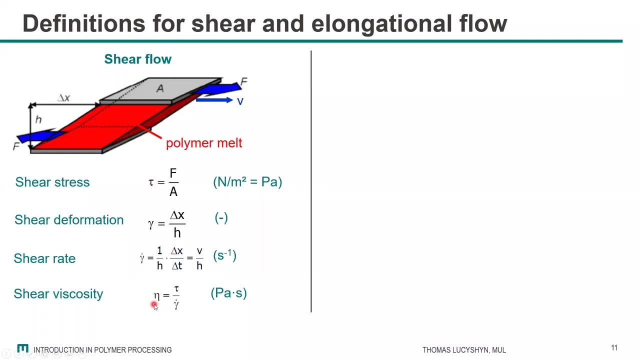 And the viscosity is basically the resistance against flow. A similar thing we can do for elongation flow. Now we have a different situation. Now the force is acting perpendicular to the surface and stretching the material, So not deforming the material sideways. 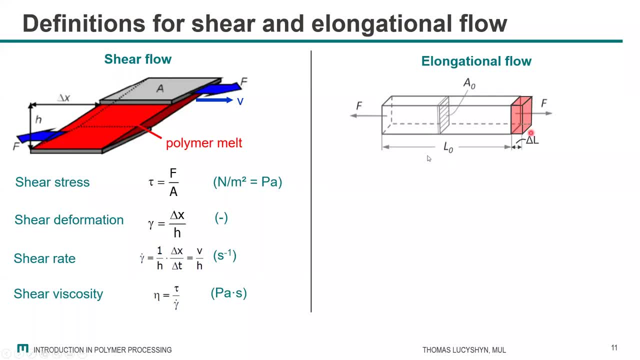 but in the length direction, if you want. We have a initial length at zero and then a deformation of Delta L, so an elongation and then a cross-section, a zero again and the force acting onto this material. Then we can define a normal stress. 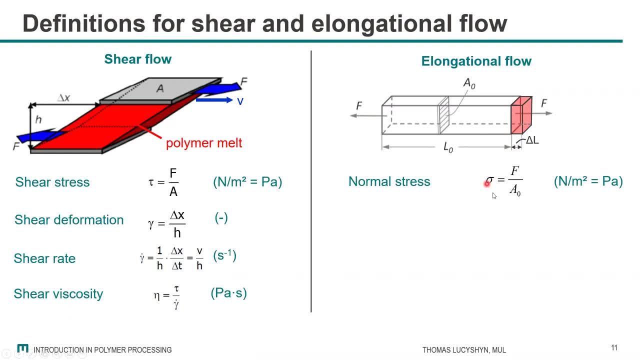 So, contrary to the shear stress now, the same equation, basically, but a different symbol. Typically, we use Sigma for a normal stress perpendicular to the surface, And it's once again the force divided by the surface. same unit, same meaning. 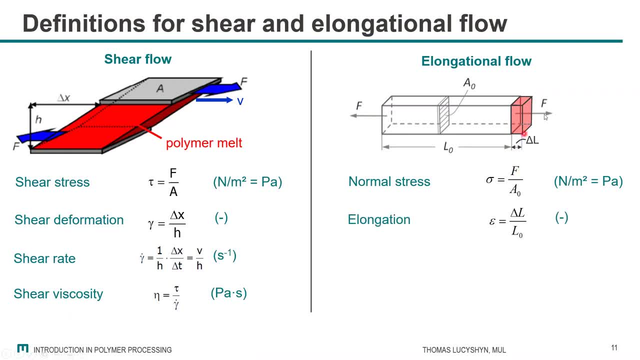 Then we can define also some kind of deformation. but now we have an elongation and not a shear deformation, And this typically the Greek letter Epsilon is used for that, And that's just the Delta L. So how much elongation is happening relative to the initial length? as zero, 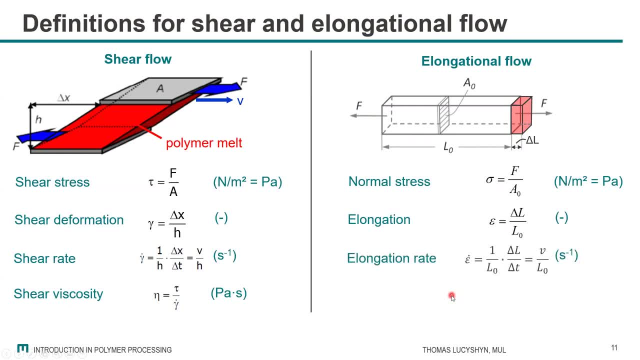 And here again we can define an elongation rate. So how fast is this elongation happening? indicated with this dot E dot is elongation per time. So once again, Delta L by L zero is the elongation per time. step Delta T. 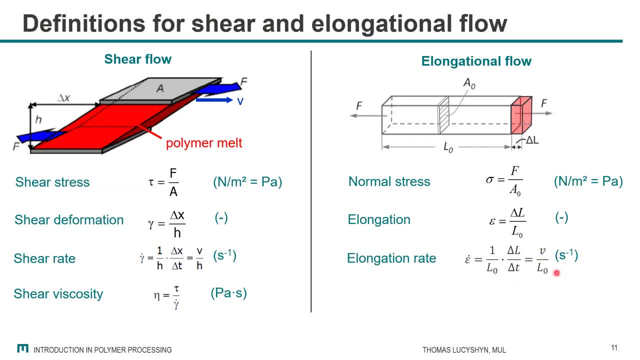 That's once again the speed of pulling divided by the initial length. The unit, by the way I forgot before- also it's second to the power of minus one, which means one by second, So reciprocal seconds, And also we can define here a viscosity. 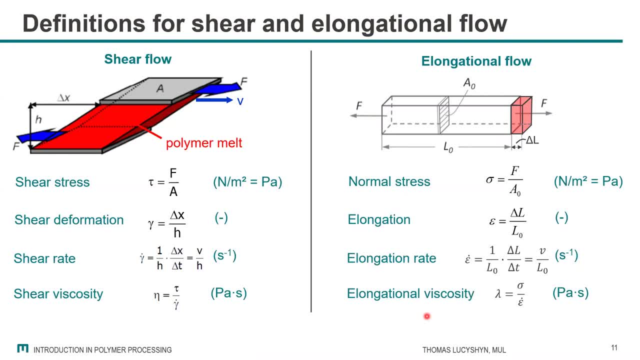 a resistance against this deformation. It's the elongation of viscosity Lambda with Sigma divided by epsilon dot. It's quite analogous to the shear deformation Remaining. focusing now on shear flow, because that's the predominant flow also in most of the processing methods. 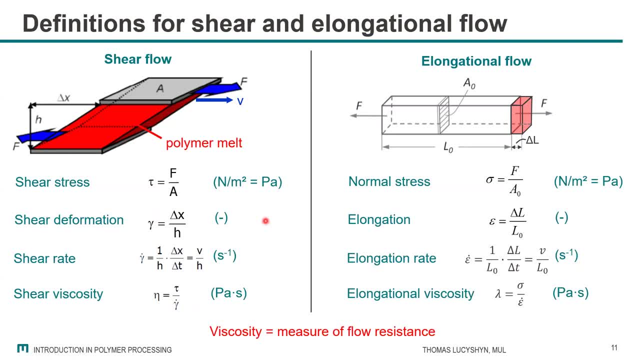 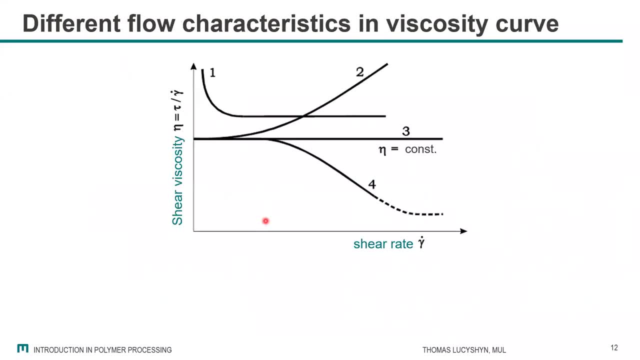 And once again, the viscosity is a measure of the flow resistance. If the viscosity is high, then there's a higher resistance against flow, And if the viscosity is low, then it's a low resistance. Not all materials are behaving the same way. 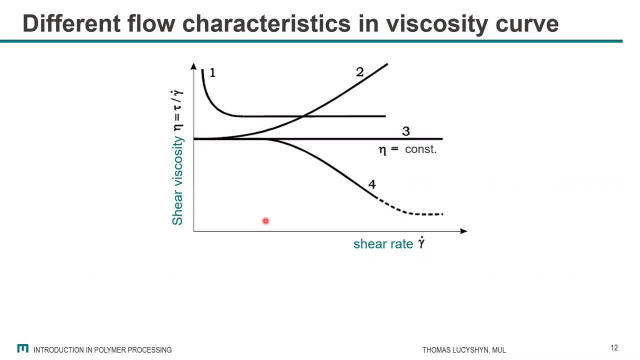 There's kind of different general characteristics of flow behavior. What you see here is the shear viscosity drawn against the shear rate. So that means the faster you are shearing, the maybe there is some change in the flow behavior, in the flow resistance. Starting with number one is the so-called Bingham behavior. 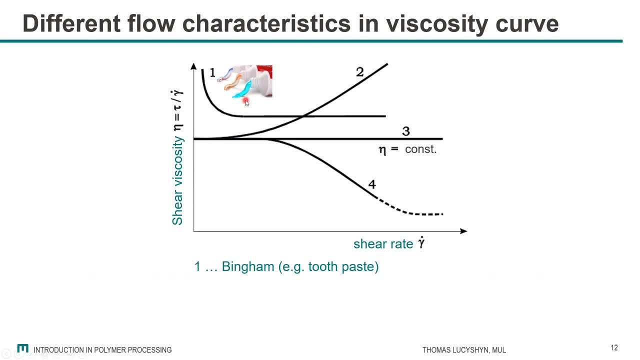 which you can find, for example, in toothpaste. That means at very low shear rates. So if there is not much movement, there's a high resistance against flow. It's really behaving like a solid body mollusk. So you need to apply a certain minimum force and nothing is happening. 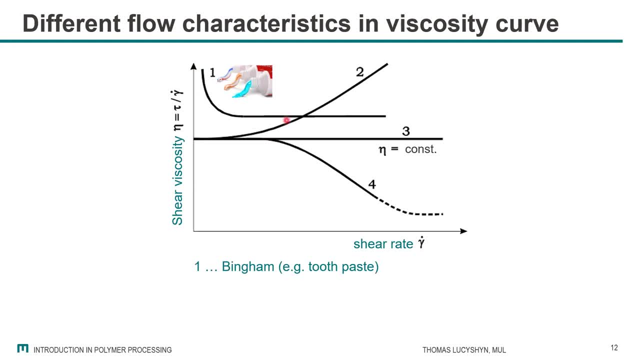 And then suddenly, once the material starts to move, then viscosity goes down and then you can really have a liquid behavior And then it starts to move. So if you press on your toothpaste container, nothing happens at the beginning and suddenly it starts to flow. 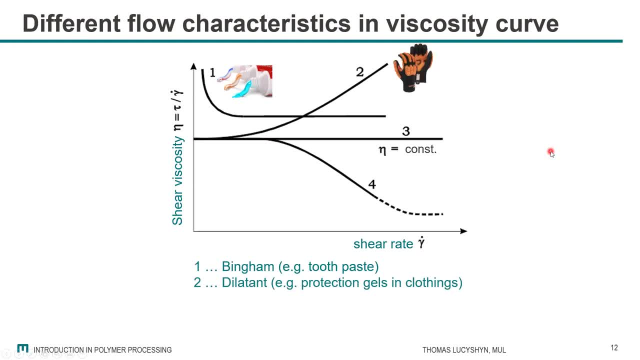 Another characteristic flow behavior is the so-called dilatant behavior, which means that with increasing shear rate the resistance against flow increases. So if you're moving faster, then there is a higher resistance against the flow. This is one example that can be used for protection. 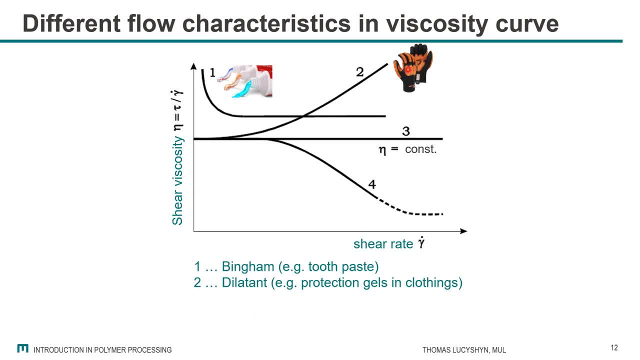 Gels. in clothings like here, for example, these protection pads are filled with some dilatant gel. That means at low speed. if you're moving your fingers, that's a low movement, then the resistance is very low, So it's flexible. 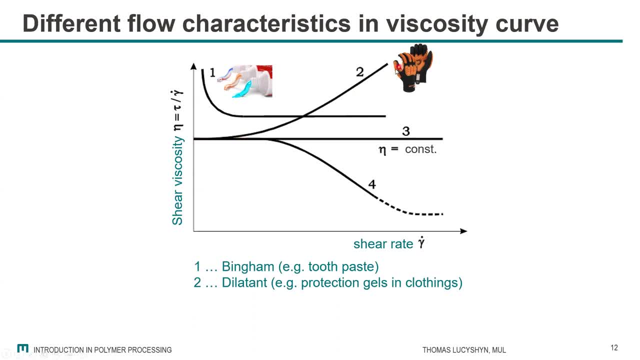 You can move it, But on an impact- for example, if you smash your hammer onto it- then it's a very fast deformation rate And therefore it react, it stiffens and therefore it has some protection effect- Then we have a very prominent characteristic flow behavior. 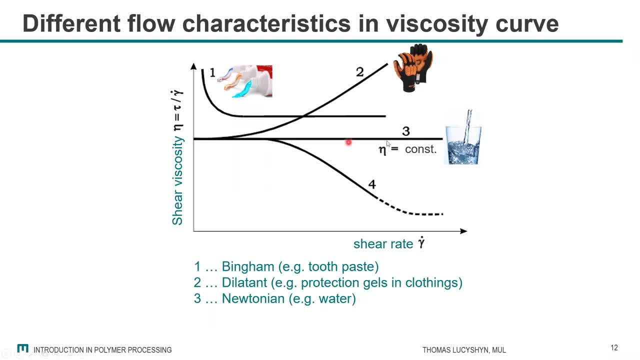 It's Newtonian flow behavior, Which means basically does not depend on the shear rate. So no matter how fast you're moving the fluid, it will always have the same flow resistance, And a typical representative of that is water. And then finally, 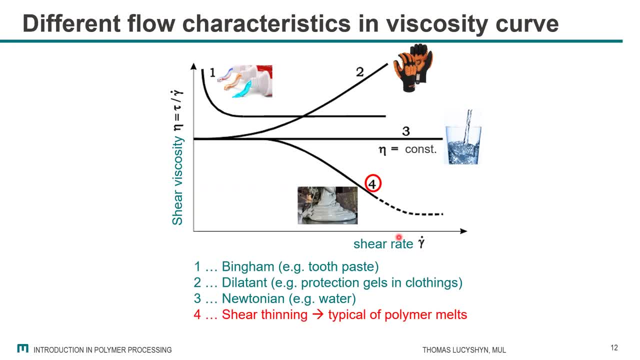 we come to. what we're dealing with most of the time is the so-called shear thinning behavior of typical of polymer melts. That means at lower movement. if we're moving not too fast, we have quite high viscosity. So it's this Newtonian plateau. 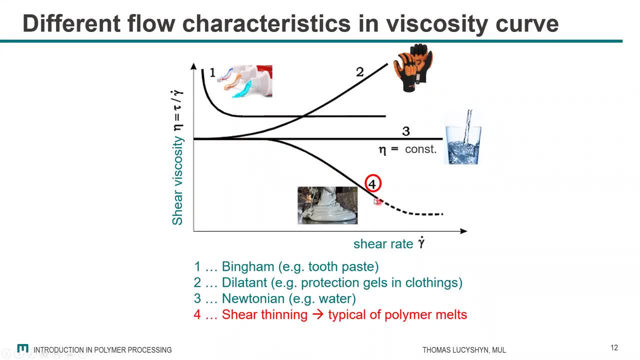 And then, typically at higher shear rates, the viscosity goes down. This is due to this disentangling of the molecular chains. They're aligning to each other, slipping easier. Then we have this decreasing of the viscosity, And this is a very nice property because this enables us basically to do injection loading. 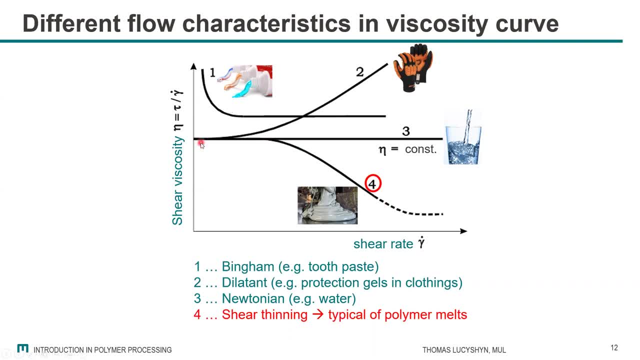 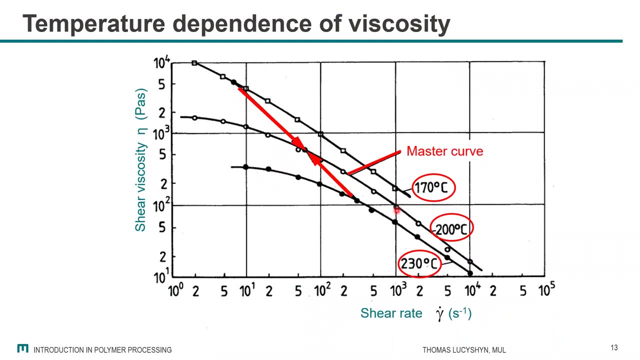 Otherwise, with this very high flow resistance, we could never fill very small gaps. So this helps us in doing fast processes in very thin channels. So this is the predominant behavior of polymer melts. It was also mentioned in the previous lecture that the viscosity depends strongly on temperature. 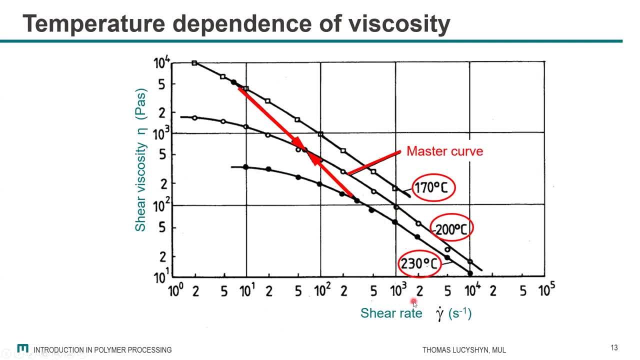 So this is just a graph Once again, the shear viscosity drawn against the shear rate. You see this typical shear thinning behavior again. at lower shear rates we have higher viscosities and it goes down to lower values at higher shear rates. 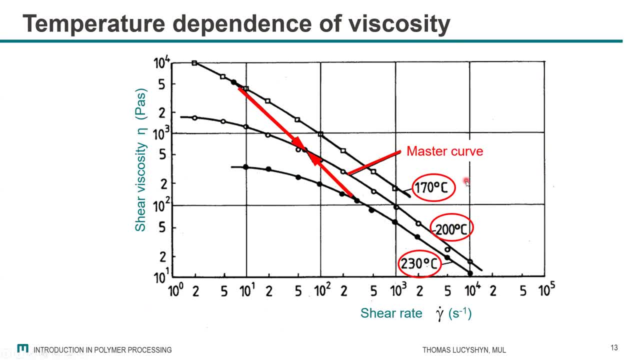 And additionally see the influence of the viscosity of the temperature. So we have measured this material at three temperatures: 170 degrees, 200 and 230.. And that's also quite logical: with increasing temperature the viscosity goes down. It's like 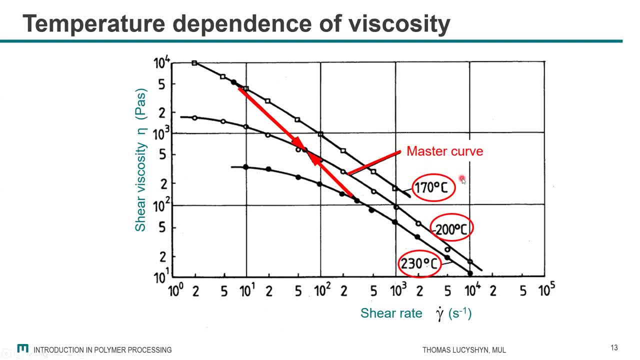 honey. if you put it into the fridge- we are here not at the same temperature, but at low temperature- then it becomes very stiff and viscose. If you heat honey on the oven and it becomes very liquid. The nice thing about this. 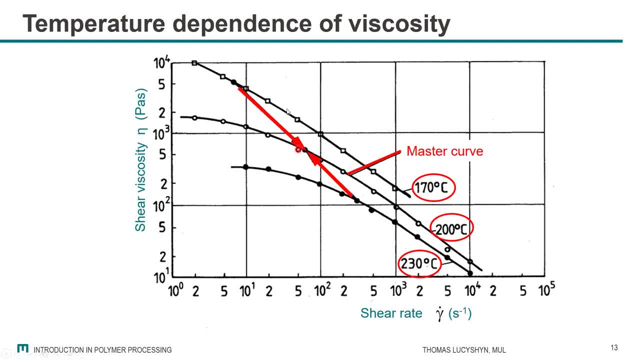 it can be calculated and shifted together to a master curve. So if we measure the viscosity at three different temperatures, we can find equations which can shift them to a master curve. And once we have those coefficients, we can then calculate any viscosity at any other temperature. 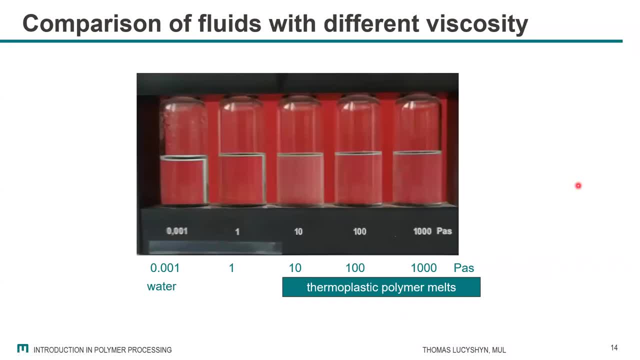 To give you a better impression of what viscosity and what melt behavior means, I'll show you these nice samples in tubes. So here are different liquids with different viscosities, starting here from 0.001 Pascal seconds, which is water. And then these are different silicon oils with different viscosities. 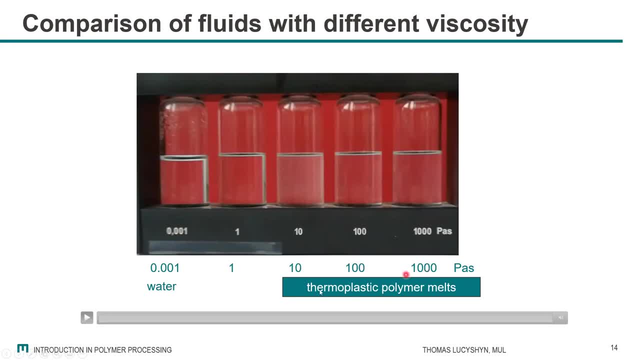 1,, 10,, 100 and 1000. And typically thermoplastic polymer melts are in the range from maybe 10 up to even more than 1000,, 10,000 and so on. What I'm going to do now is to flip this. 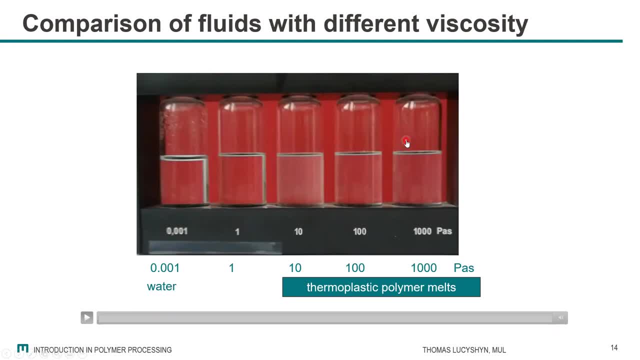 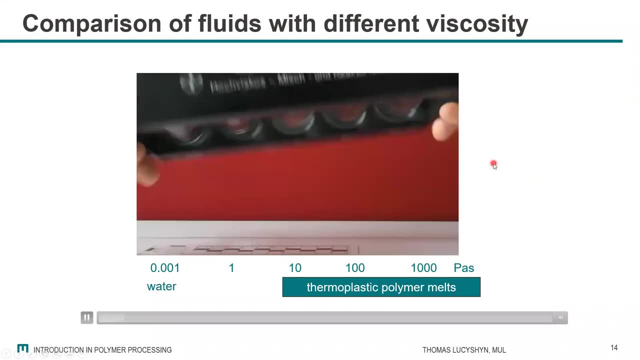 this one. so turn it top down and you see how the materials follow gravity. Oops, sorry, So nothing is happening. Here's the fluid. Now it turns around. Of course, the water follows immediately the gravity. This one with one Pascal second is also already here. 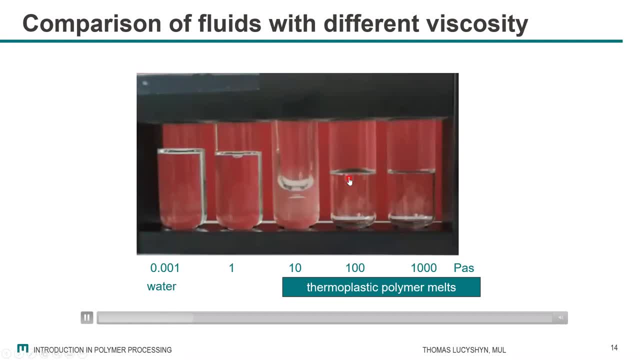 This is still moving. Here you can see that it starts slowly to move. You can also see that it sticks to the wall. And now this, this parabolic shape, starts to develop where the, the melt goes down, And what you can also notice here. 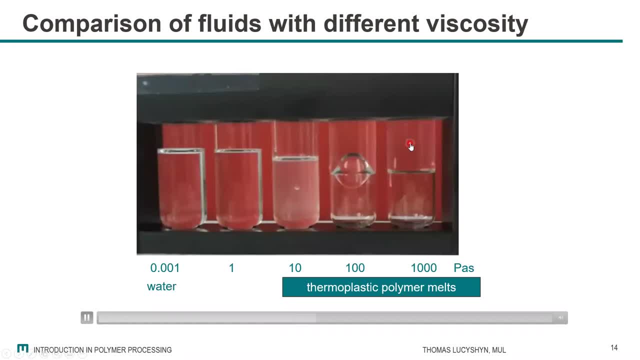 So the liquid is not down here, The liquid is still up here, So that at 1000 Pascal seconds the material doesn't show any motivation to move, just due to gravity. So that means also for our processing you need to apply quite an amount of pressure to really motivate the material to move. 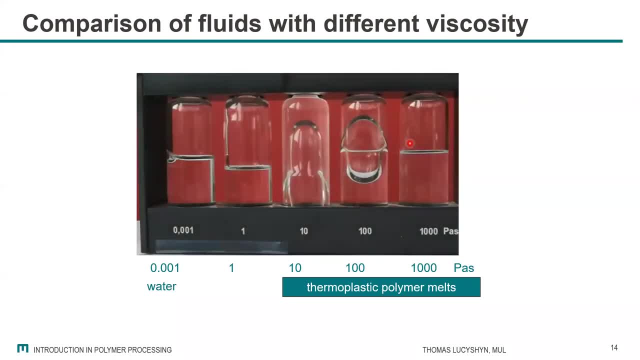 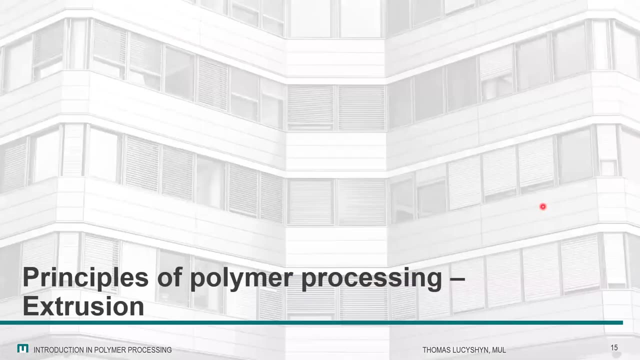 Turn it around again. So just to give you an impression, what do we consider as being melt state? And so not that you think that's like water when you melt ice. So this is really important to understand the basic principles of material flow. 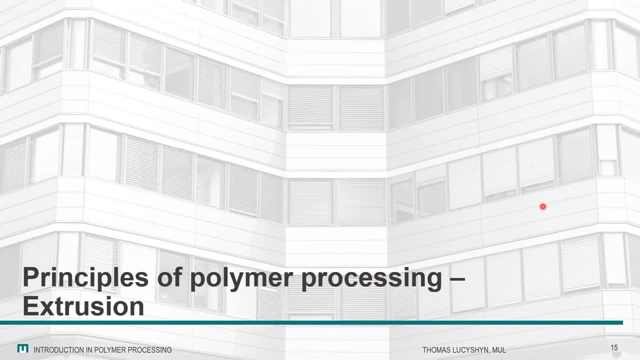 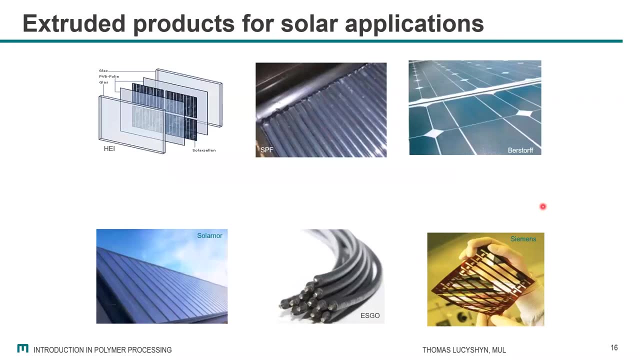 You can, of course, dive much deeper into this topic, But this, I think, should be sufficient to also get a little bit of an understanding what is happening inside a processing machine. Well then, let's go first. The first one is about extrusion. 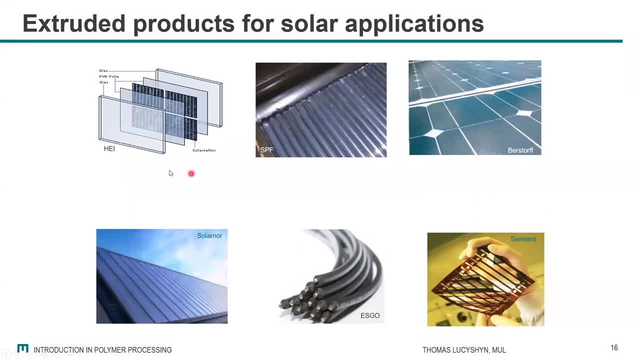 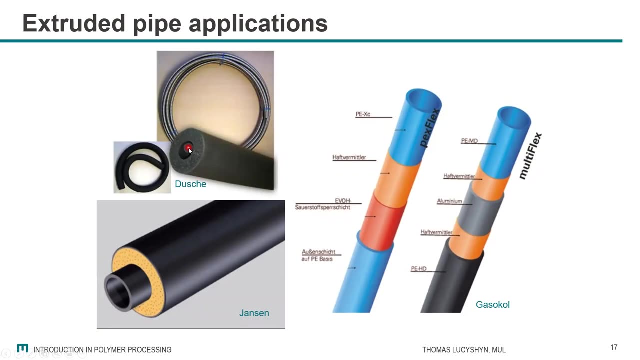 So just show you first some typical extruded products Like could be sheets, plates, uh wires, films for different applications, in that case some applications taken from solar applications. Pipes can be foamed to get some better insulation properties. Here we have some pipes which are 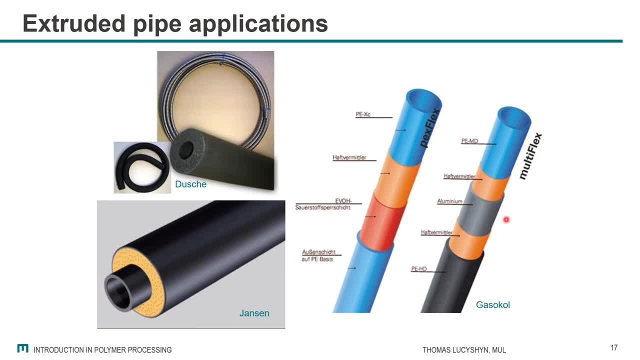 typically multi-layer pipes, which is of course, in terms of property profile for the application, it's necessary to have different materials combined. On the other hand, this of course, from the perspective of recyclers it's a nightmare. so we have to kind of separate this. 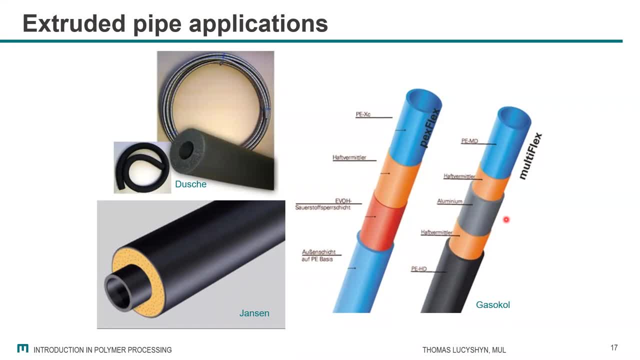 or in the best case, the option would be if we can achieve the same property profile with the same base material, but maybe with different morphologies or different structural differences, but the base polymer chemical structure is the same. But this is really. we are kind of forced to do this in. 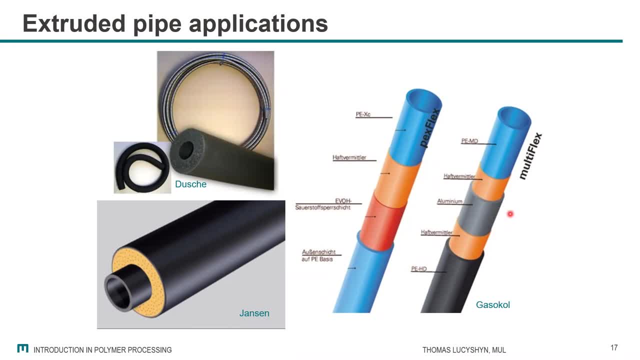 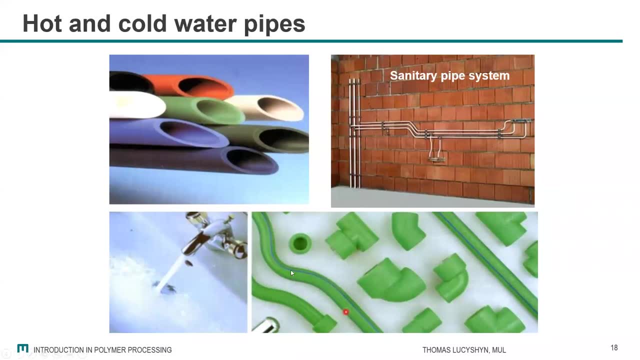 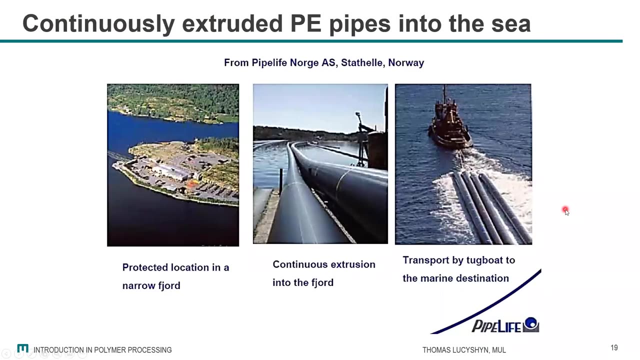 order to achieve a certain property profile. but of course, for recycling this is not a good option. Other examples: for sanitary pipe system in household, these are extruded. these are not extruded, by the way, on this picture they are injection molded. these single parts. Another nice example, an extreme example of 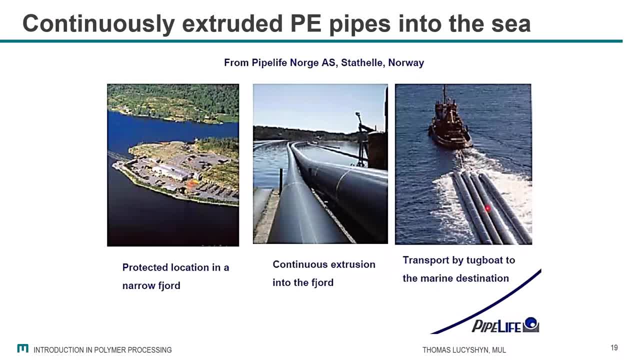 extrusion is like if you want to apply those huge pipes for protection of glass fibers over the ocean from Europe to the US. they have to be transported and put into place and in this case it's not feasible to extrude it in some plant somewhere in the country and then transport the 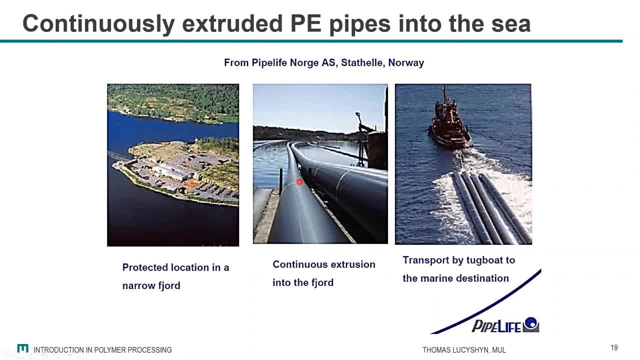 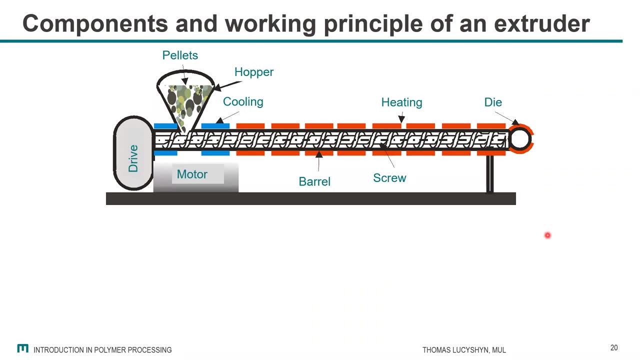 huge pipes to the sea and then transport it. No, they are directly extruded into the sea, cut and then transported by a tugboat to the marine destination. It's quite some nice extreme example of what can be done. I'd now like to explain a little bit the working principle of such an extruder. So basically an. 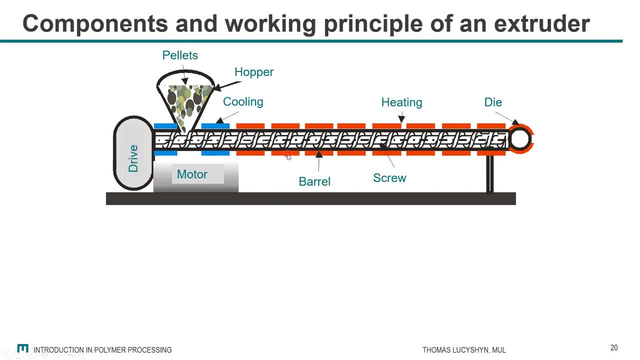 extruder consists of a barrel which is like a metal cylinder, with some heater bands outside so that you're able to heat the material, because we need to heat it for thermoplastic melting- And the core of this extruder is this. This is the element here, And this screw is continuously rotating, and by rotating it, 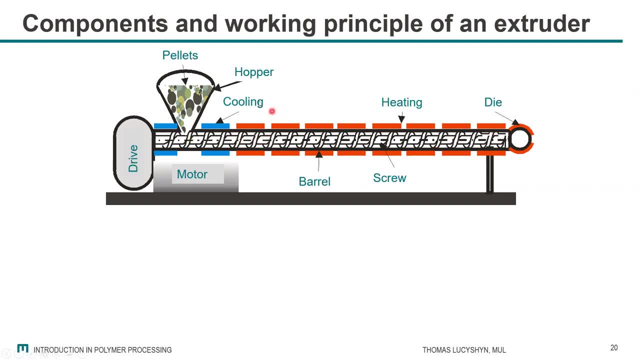 transports the material from here to the front. We have here to enter. to introduce the material. we have a hopper and typically pellets are introduced to this hopper. The entrance section has to be cooled, otherwise the material would already melt here and the pellets would not fall. 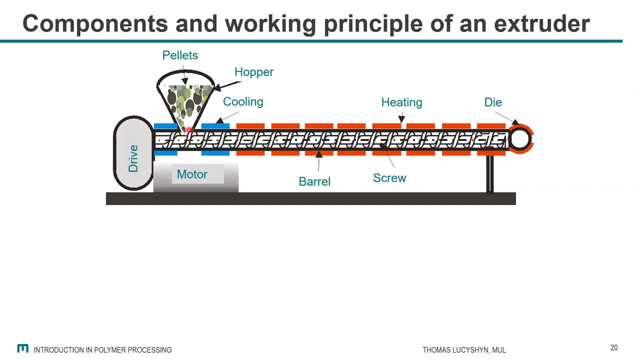 in but make a big, huge bunch of material and cannot. it would block everything. Of course we have a motor in the drive to get this rotational movement of the screw, And in the front of the extruder we have a die which is just a symbol here. The die is basically a metal block with some 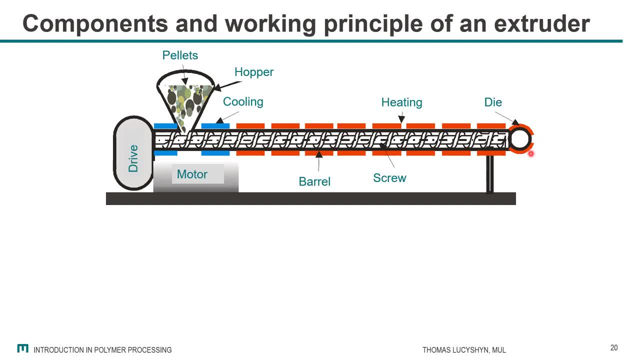 geometry in it, and you pump the material from this die And, depending on the shape of this die, you get a profile, a sheet, a pipe, whatever. So the process is like that. So first you're feeding the pellets into the hopper, can be manually, can also be, of course, automated by some pipes and some. 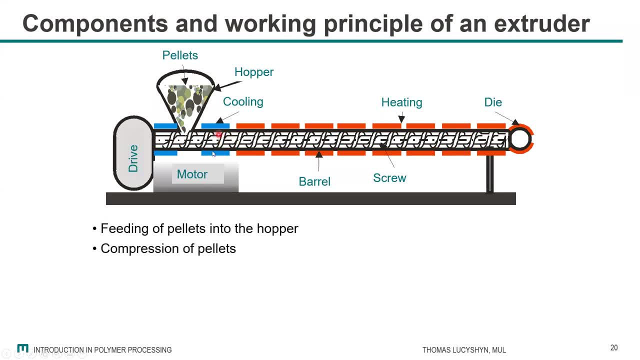 pellets into this hopper, Then in this zone the pellets are compressed and then the melting happens. in this zone, Then, close to the front, there's some kind of homogenization of the melt And then finally the melt is pumped through the die And depending really on which kind of die, 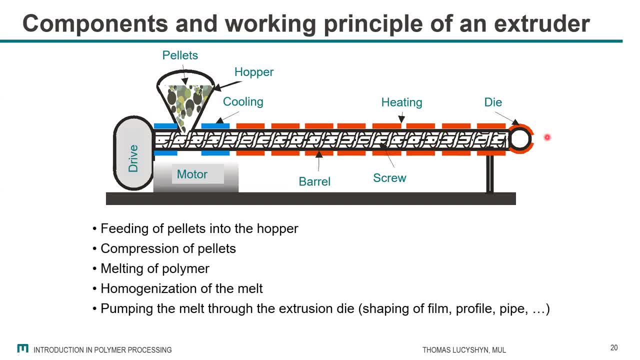 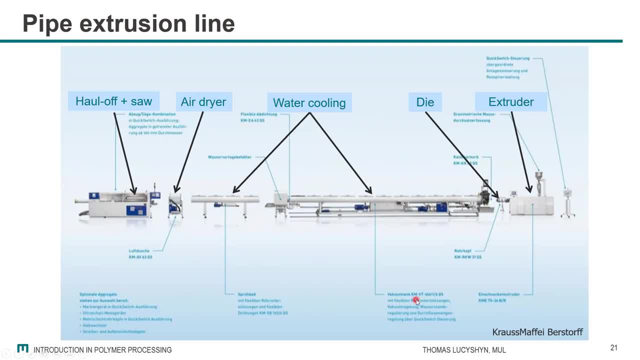 you use. you can shape your film profile by whatever you want. This is a pipe extrusion line. Don't worry about those single descriptions. It's just about the dimensions of the whole line, So it's not only about the extruder. 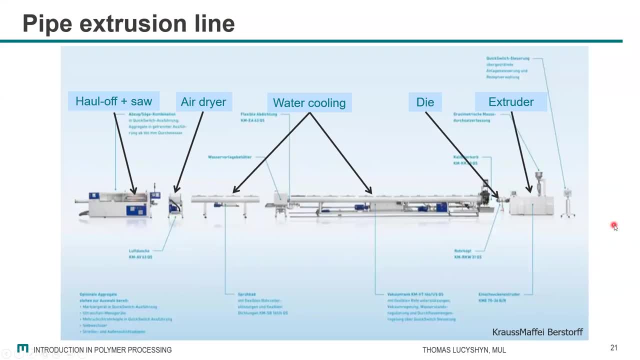 we need some other peripheral devices to get a product out of it. So the whole line consists basically of the extruder. The main function of the extruder is just melting and conveying the material continuously. Then we have the die where the melt is pumped through, And then the material. 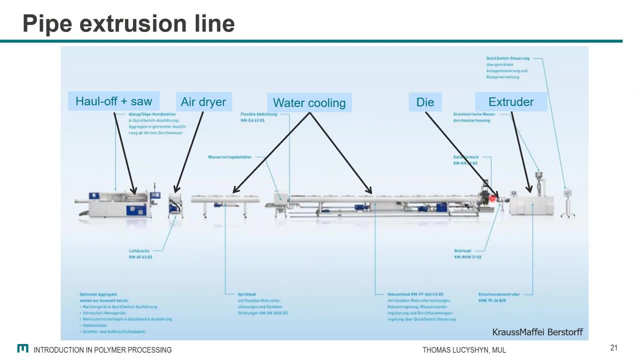 comes out is still soft, So otherwise, if we don't do anything about it, it would just collapse and would not remain a pipe. So we have to guide this pipe through a cooling bath, the water cooling, so that it cools down and it stays rigid and 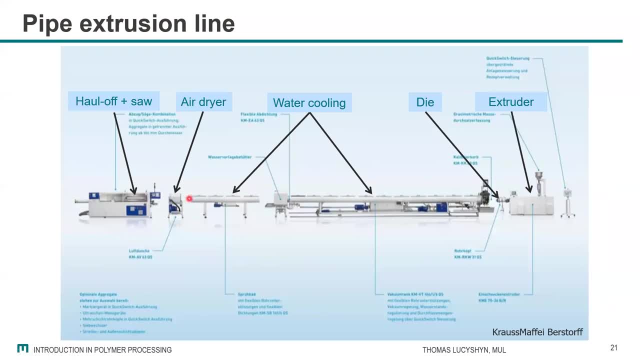 keeps its shape. Then as it comes out here it's still wet from the outside. cooling bath. It has to be dried by an air dryer so that the outside water is removed. And then here is a hole of unit where it takes the pipe and transports it away, And also a saw- otherwise we would. 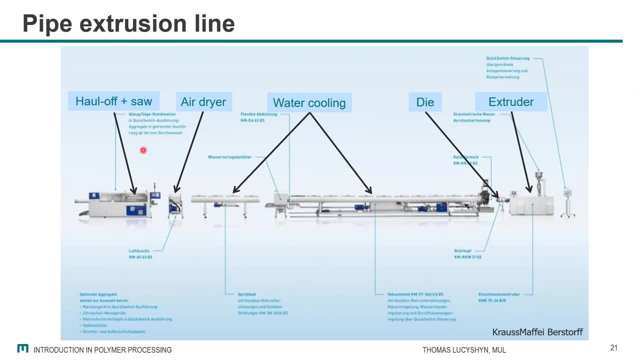 produce an endless pipe which we never can transport anywhere. So we have to cut it to pieces so that we can transport them. That's a huge line, needs a lot of space And, depending on the pipe dimensions, it can be really very long. 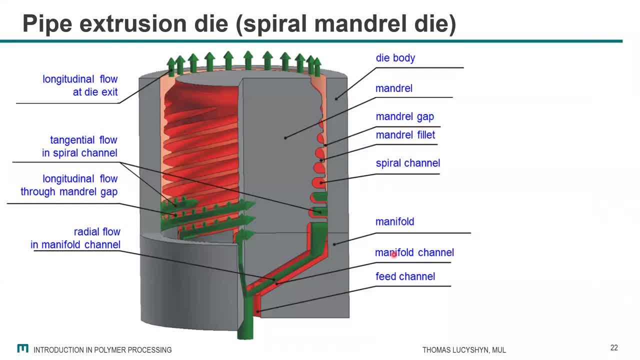 Just some details how it looks like in such a die. The main job of this die is to distribute the melt coming from the extruder, from the bottom. Here is: the extruder provides the melt in a circular cross section, a full cross section, And now we have to distribute this melt to an 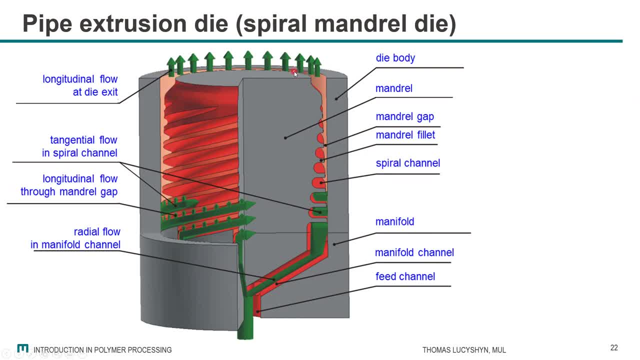 annular slit which forms the pipe, so that it looks like a pipe in the end and not like a bar. So what it does is basically it transports first the. there are channels transporting the melt from the inside to the outside, And then we would have like several channels and just some flow. 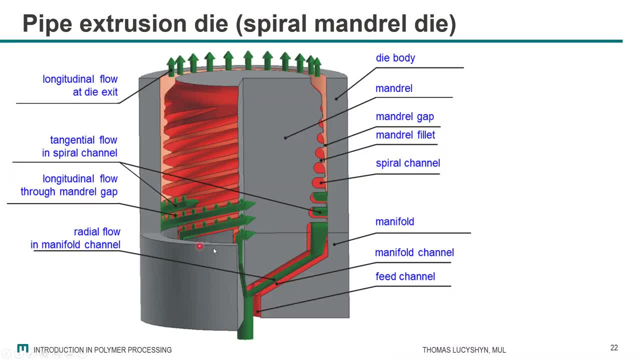 some different flow paths there, So we have to distribute it over the circumferences And this is done via these spiral channels, What you can see here in the cross section at the beginning. those channels are quite deep, So the flow resistance is quite low. 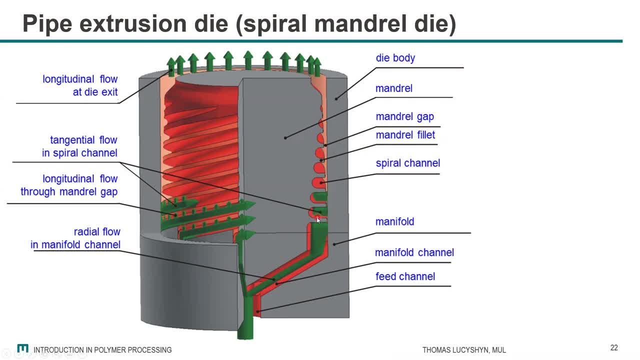 So material likes to go there because there is enough space to go And there is not a chance to get from one channel to the next. As the flow progresses in the actual direction, those channels smaller and smaller, So there is a bigger resistance of flow in here. So the material 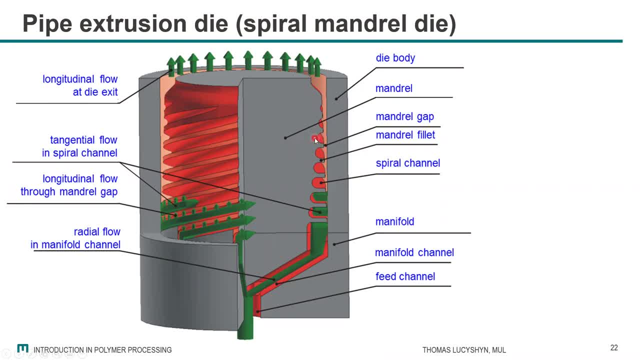 doesn't want to go there anymore because it's a long way around and it's a very small channel. But we open the possibility of the material to change from one channel to the next, So to move more in the actual direction. So not moving in the circumferential direction, but rather in 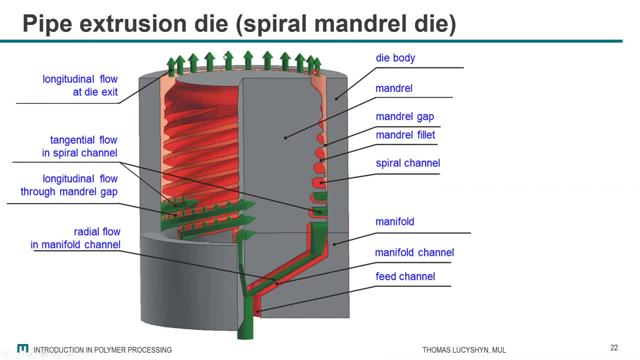 the actual direction And then at the end we achieve what we want. We get the material coming out of this round slit in all the same velocity, all over the circumference and with the same speed. So that's how it looks like in reality. We have those different channels around the 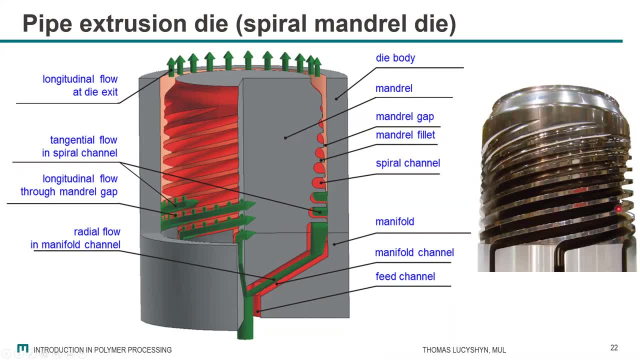 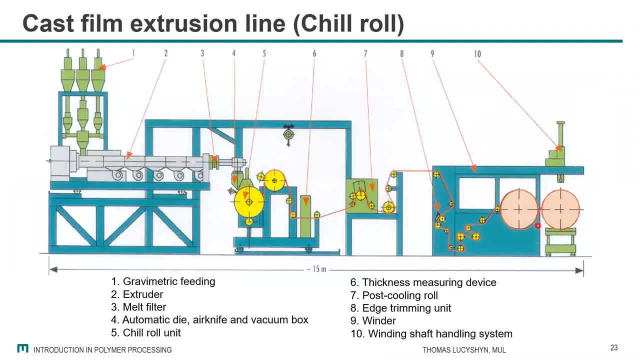 circumference and then those spiral channels distributing the metal over the circumference. Another extrusion type for another product is for films, And there are two types for films. There's cast film and blown film. This one is cast film extrusion line. So once again, 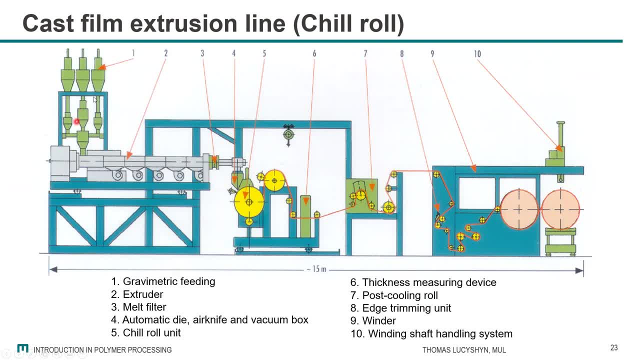 here we start with an extruder. You can add different components to your base material, like fillers, for example, to enhance some properties, And here we have the classical extruder with the screw melting and conveying the material. Then we can also add some melt filters to filter out some contaminants, for example, And then 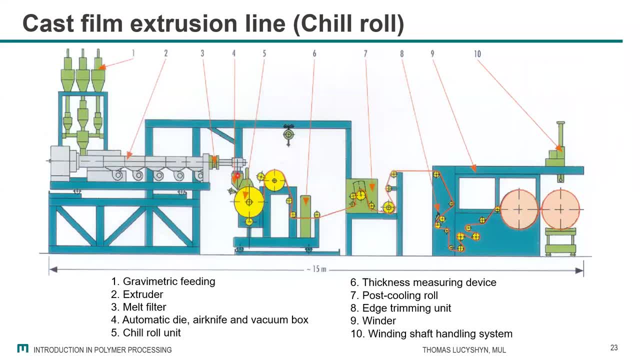 here is the core part of this is the die, which is a slit die. Basically, the slit is a wide, a very wide rectangular slit. So the cross section is a rectangle which is very wide and very thin, So like 50 micrometers thick but maybe one meter wide, And that's basically the shape of a film. 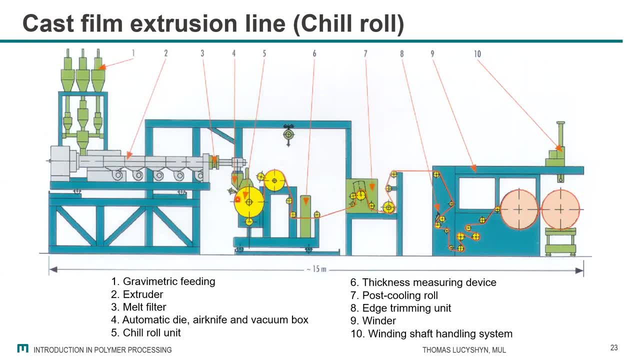 film. And this film comes out in a melt state and immediately after exiting the dye, of course it has to be frozen, otherwise we wouldn't get a defined shape. And then it gets to contact with this huge polished metal rolls which are cooled. Therefore it's called a chill. 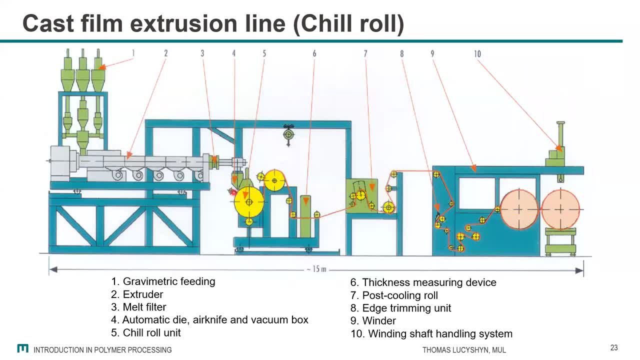 roll. it's chilled And then it freezes immediately upon contact with this roll and stays in its shape. And then there's some additional cooling rolls. You can do some thickness measurement for changing the controlling the whole device. There's some post cooling station. There's. 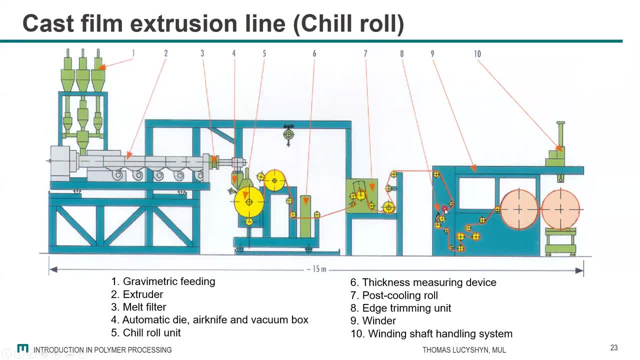 some edge trimming, because the edges are typically don't look very nice, So we have to trim it away. This is also some waste- internal waste, which can rather easily be recycled because it's not contaminated, It's pure material. And then in the end we have some- yeah, some. 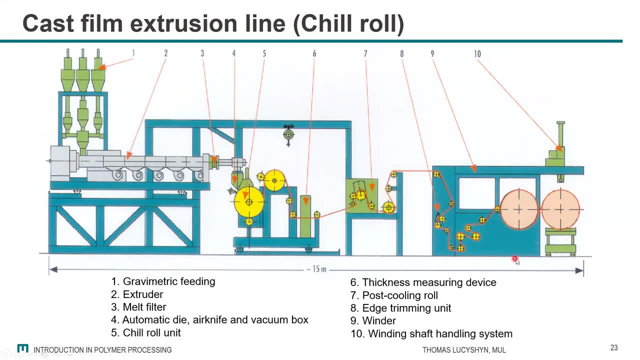 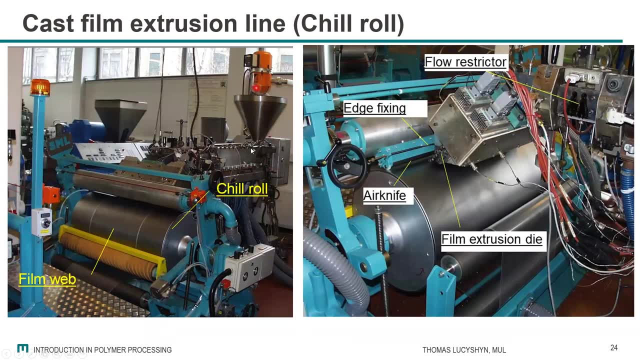 winder. here and there we have the big rolls of the films being ready for shipping. That's how it works. This is how it looks like in reality. So there is the extruder, the hopper and here the extruder and that's the dye. So that's, in this case, like almost a meter wide, And 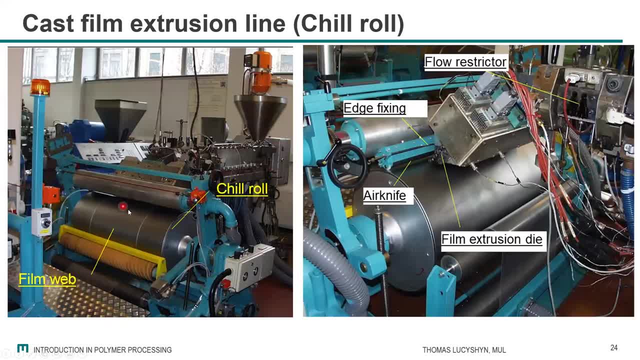 then here the film is coming out. So it's the film which is already cooled down. Here's another perspective from the other direction. So here is the dye and here the melt is coming out directly into contact with the, with the big chill roll, And, yeah, there's some air. 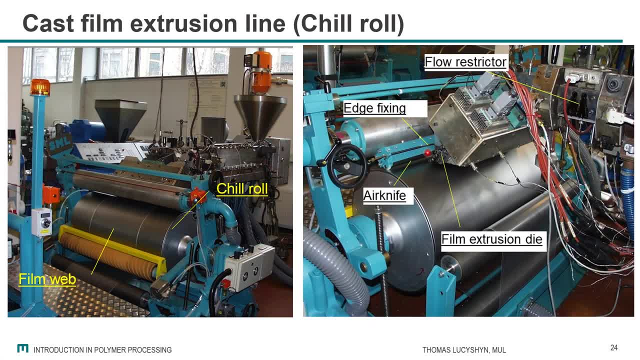 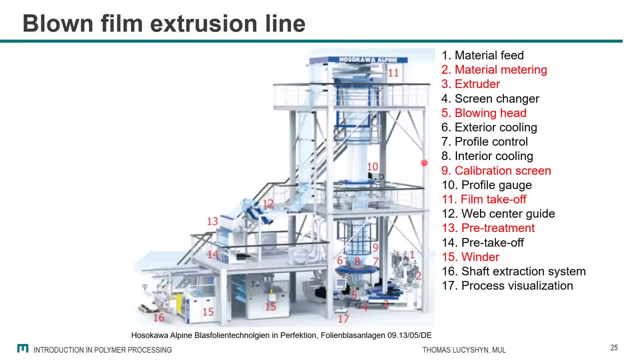 knife with some air blowing onto it so that it makes sure that the film gets into contact with the mold and stays there. It's not going in Any unwanted direction. Another film production line is the so-called blown film for for bags- basically one production. 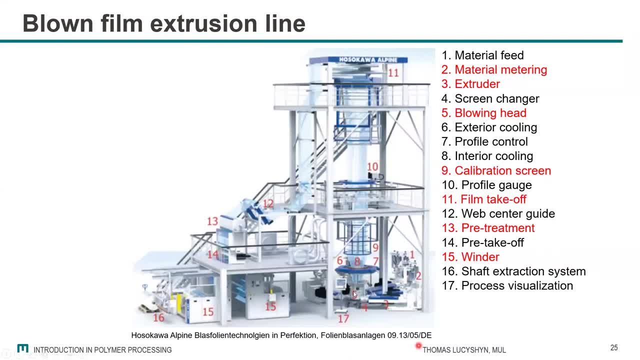 It's. they're huge really, production lines. So this is like if you would see a person standing here. it would be like this size Here's, here are the extruders and it's really can be up to like 10 meters high. It's really huge plants there. 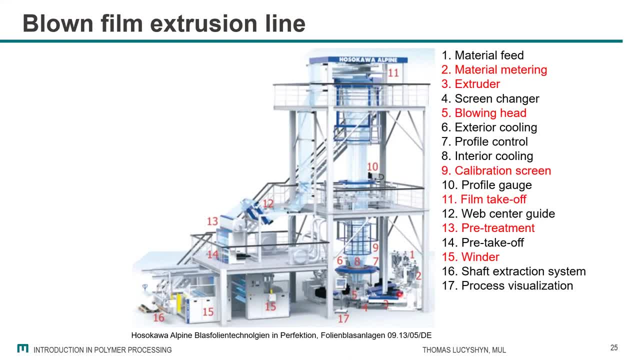 I just want to focus on the most important components of it. So here we have an extruder providing melt. Then we have the the dye. the dye which is extruding a very thin hose of deformable melt which is then blown up by air so that it's expanding. So if you blow, 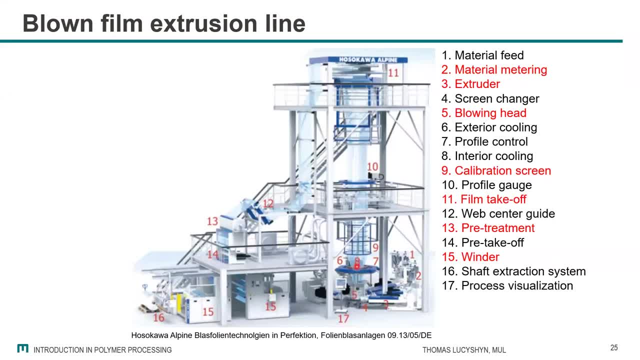 from the inside, like in a balloon. you blow the air inside and it expands. And in order to not to make this expansion uncontrollable, we need this, this calibration screen which is around to limit the expansion of this. Yeah, Yeah. 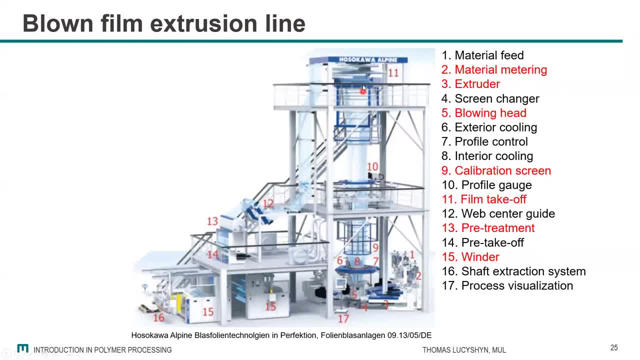 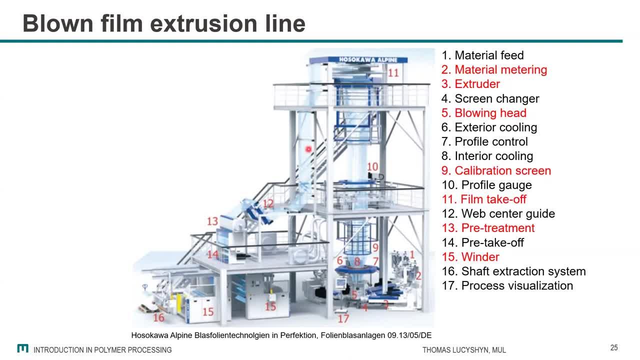 wind up, take off and flattening again And in the end we have a huge winder where you have those film roles but they're kind of close. So before we had like the cross section of this was like a film like this. this would be the thickness in like 50 micrometers and 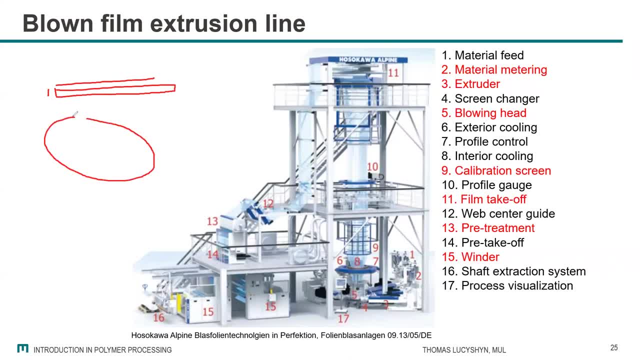 very wide And now we are getting more or less closed films, which you can flatten, of course, But I don't know. but this would be the cross section of this. that would be the result of this film. so it's a round closed bag, whereas this is just one flat film. 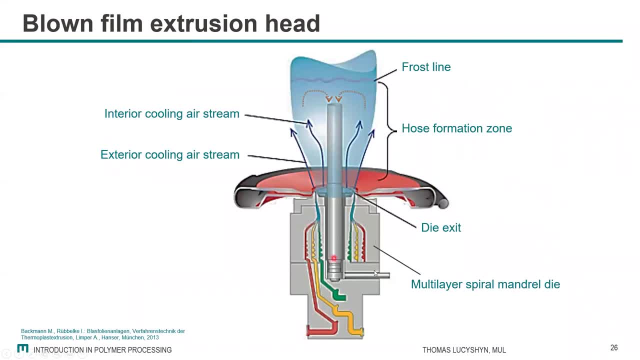 Having a look at the, the die. so once again we have this, this multi-layer spiral mineral there, as I showed you before, but now for more materials. so typically, films are not used in one material, but typically have a layer, structures or multi-layer in order to- yeah, to have all the requirements fulfilled. it's not in many cases, not only one polymer is. 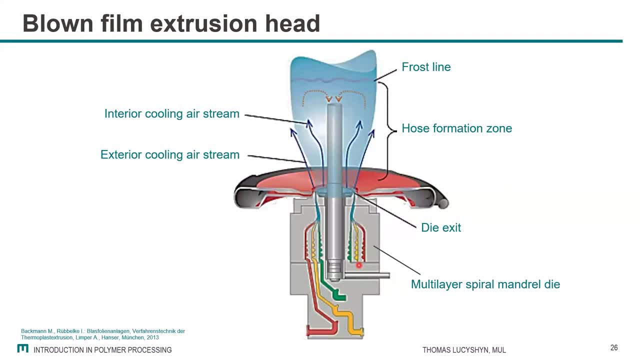 sufficient. we need more layers with different functions, for like barrier functions or mechanical properties and so on. so it's it's not yet easy to achieve a property profile with one single material. So once again here, the metal, the melt, is coming out, and then we have this blowing air where the, the melt is expanded until a 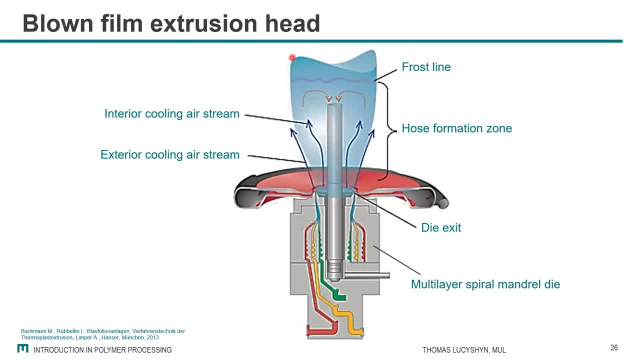 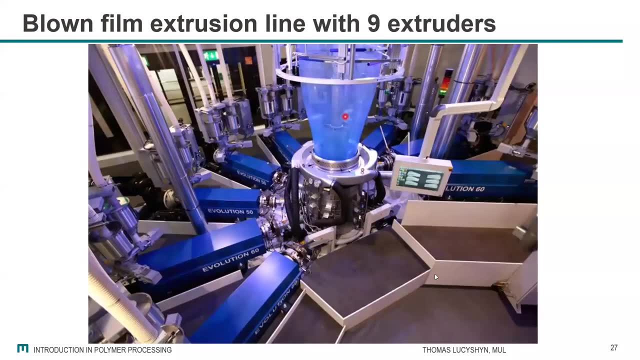 certain point, when it's freezing, so there's a frost line, so there are no further warm. deformation is happening, and this is the working principle of such a blown film line, One example of it. so here, in that case, we are nine extruders providing nine, maybe different. 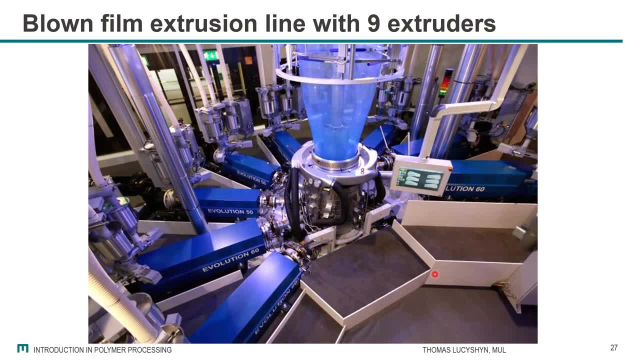 materials, or at least nine different layers for this film. so once again, in the technical point of view, it's very fascinating. what is possible? of course, from the viewpoint of the recycling it's once again a nightmare. So this is really: nine barriers, nine layers of different. 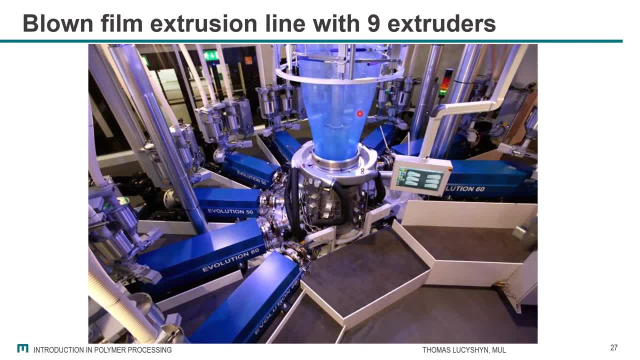 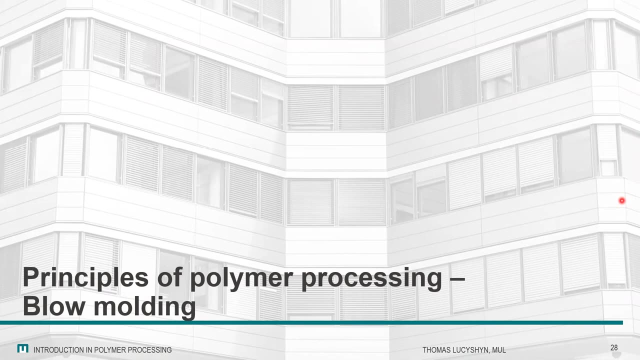 materials combined in one product, basically, which you cannot really separate easily. It's, of course, a big problem and something that has to be addressed, a challenge. All right, then let's go to the next molding principle. It's the principle of blow molding. 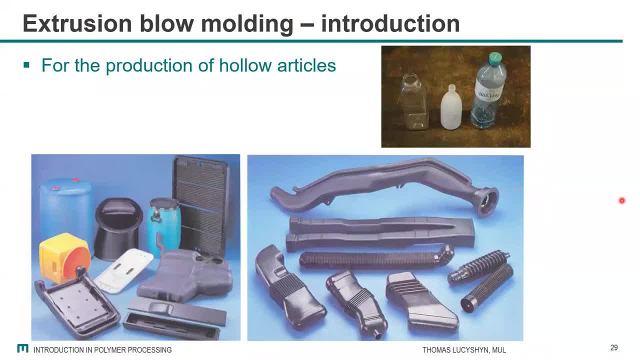 The typical products from blow molding are hollow articles like can be simple bottles, but can also be complex shapes like fuel tanks or parts of that, or like on this side of containers. whatever, And the typical procedure for this method is, you know, two fundamental phases. 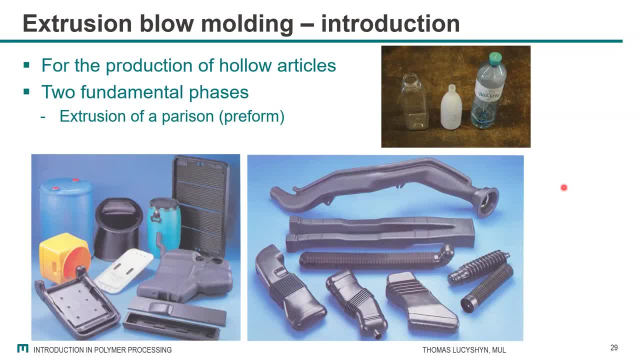 The first one is using an extruder again, and extrusion of a Parisian kind of preform. I'll show you in later slides what it looks like. And then, once again, this Parisian is is blown with with- uh, it's blown fast with air and then gets its final shape. 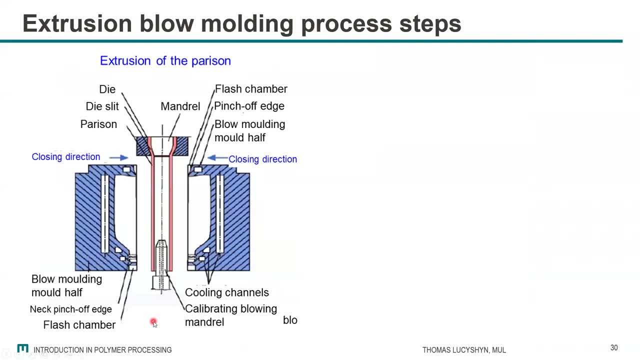 So how does it look? So this is a cross section of this. We have a mold consisting of two mold halves and inside you can see here the shape of the final geometry which will be a bottle once it's connected. And the first step is the mold is open, So both mold halves are on the side And then the 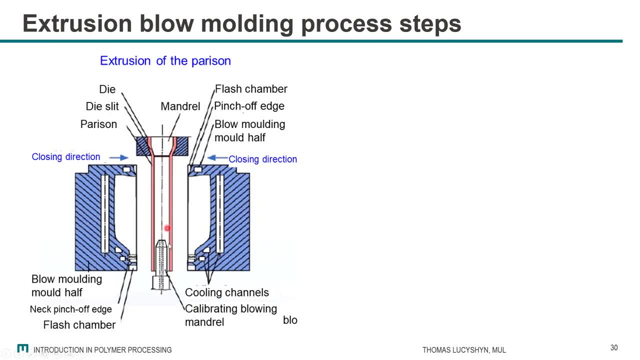 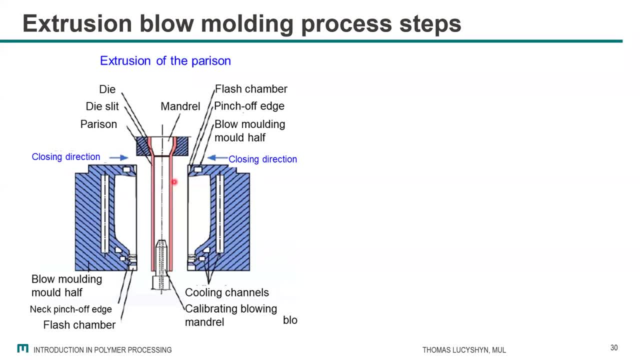 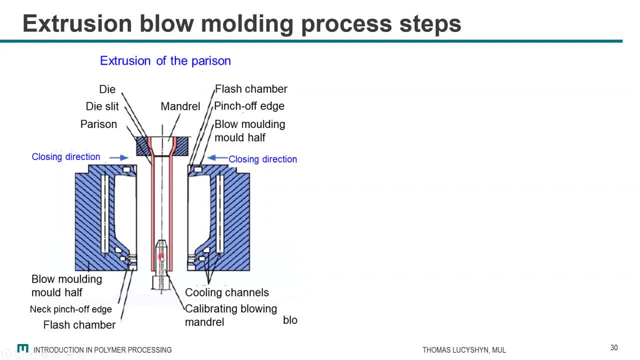 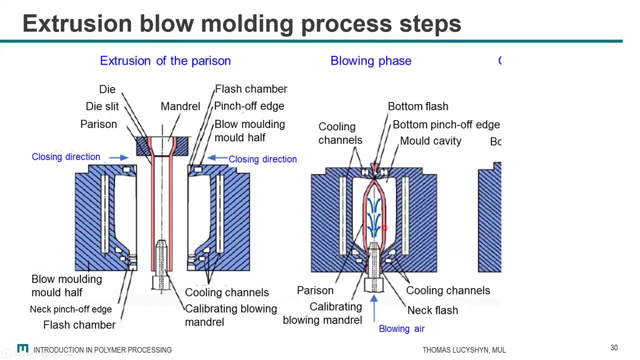 Then from the bottom, this calibrating, blowing mentalists is entering here, and then on the top and on the bottom, in the next step it's closed. So the mode is closing, and then it's closed here, It's closed here. So basically, this hosts is air tight. And now, with this blowing air, with this, 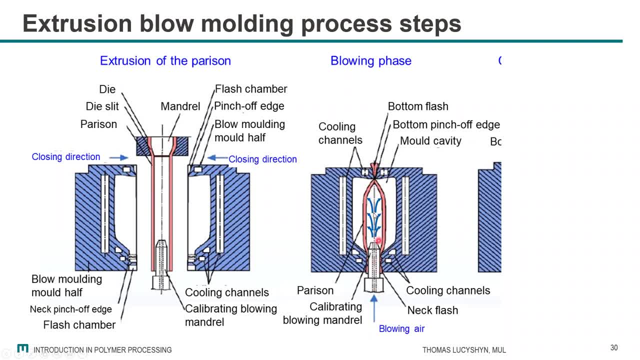 mandrel air is blown into this um, into this parison, and inflates it and, by applying this air pressure, then inflates it and expands the material to the shape of the final bottle. so it comes into contact with the, with the melt, with the, with the mold, with the tool. 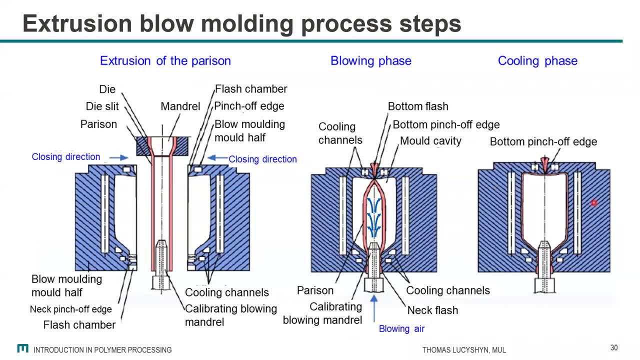 with the steel it cools down, and after it has sufficiently cooled down so that this stiff again, stiff enough for deformation, for demolding, then the mold opens again and then the part can be taken out. so if you're having a look at hollow bodies, you will most probably see some some parting lines where the two melt. 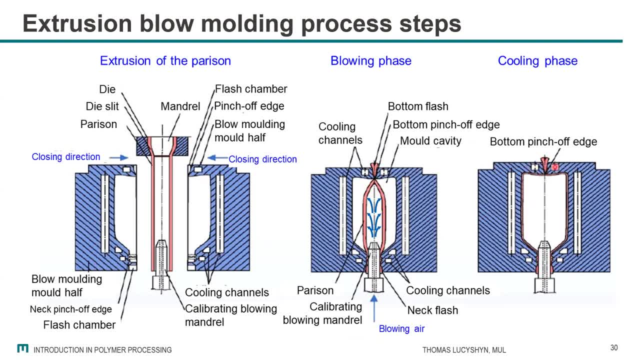 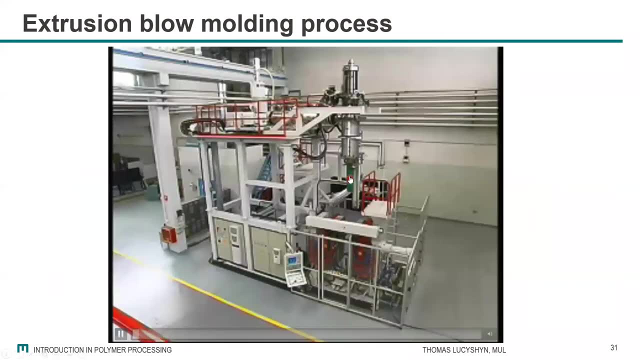 to the mold halves are meeting, so you can find this on typical, if you have like containers for i don't know, for bathing or so, you will very often find this, this, this line on the sides coming from this process, there is a movie showing you how it works. it's a bigger container, so now, 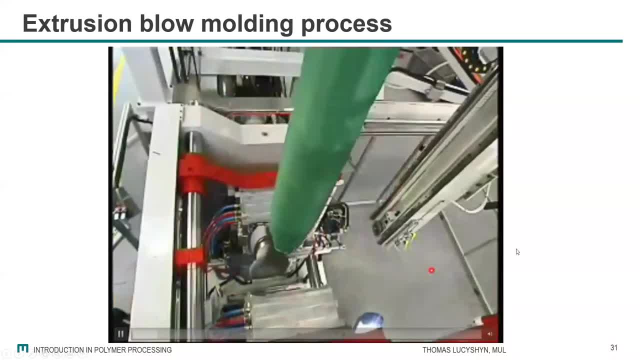 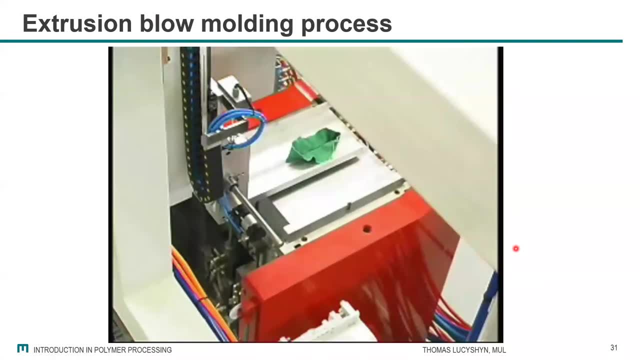 the from vertically the parison is extruded down to the mold which is open at the moment. it comes down, then it's closed. it's blown already. it's very fast, so the blowing stage stage is very fast, then it cools. we have to wait until it's. 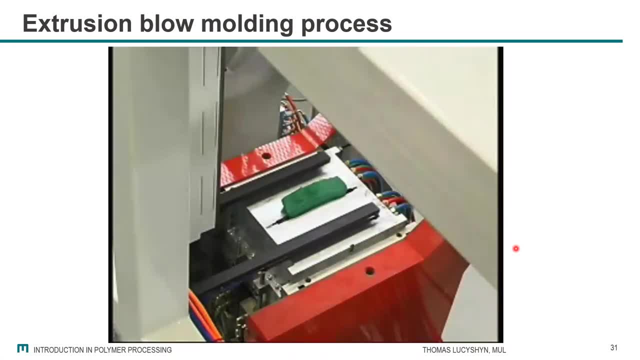 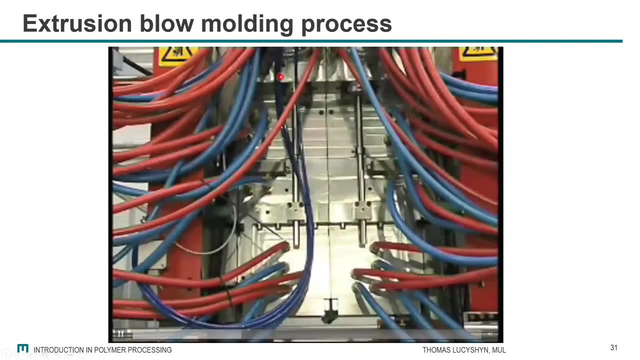 sufficiently cold and sufficiently rigid, and then this is taken again with the robot and the mold is opening in the meanwhile you see that the next person is already coming, because we have to combine here a continuous process of extrusion and a discontinuous process of molding, so it has to be synchronized in some. 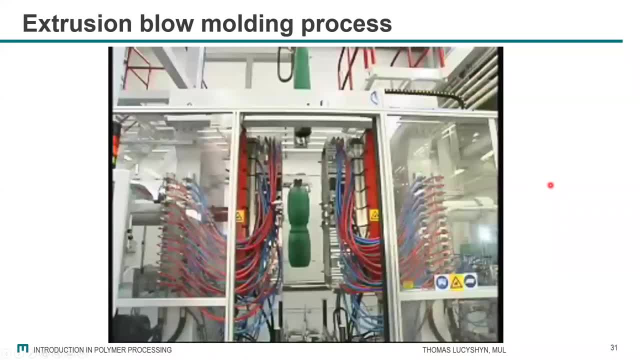 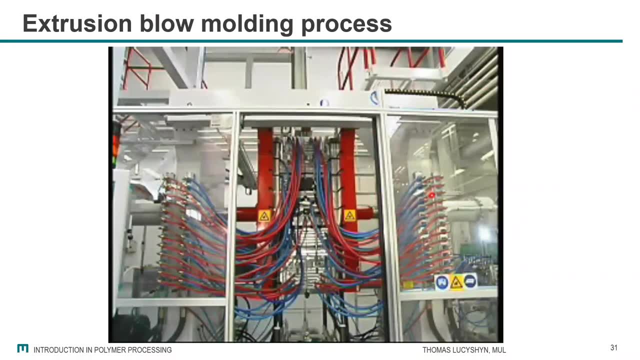 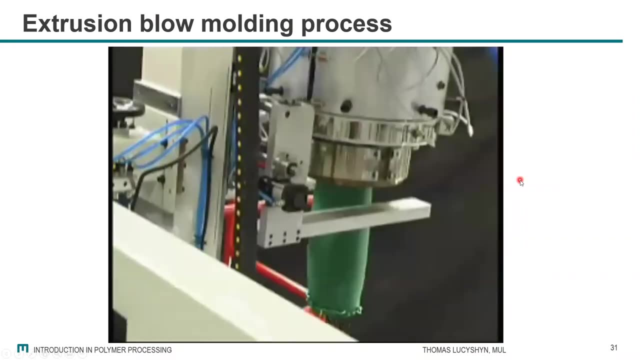 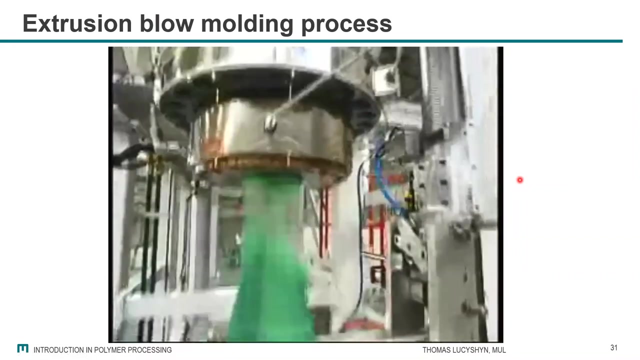 way, so where, while the one is produced, the next one is already extruded and once again the next shaping has happened, takes some cooling time, then it's opened again. once again, you see how it's extruded, and so in general it's, although the product itself is a discontinuous. 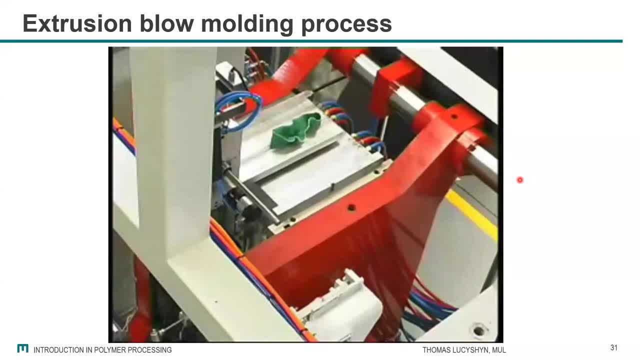 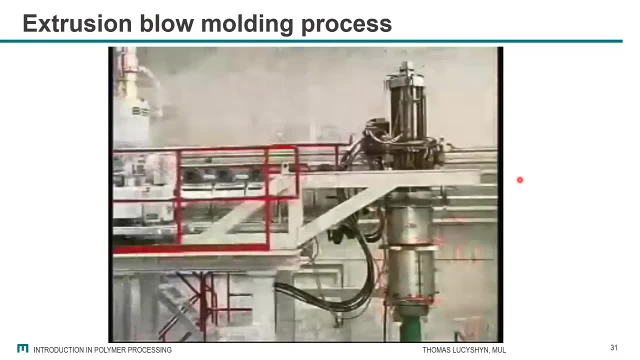 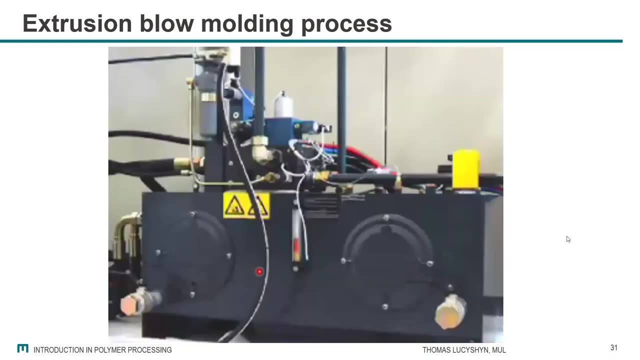 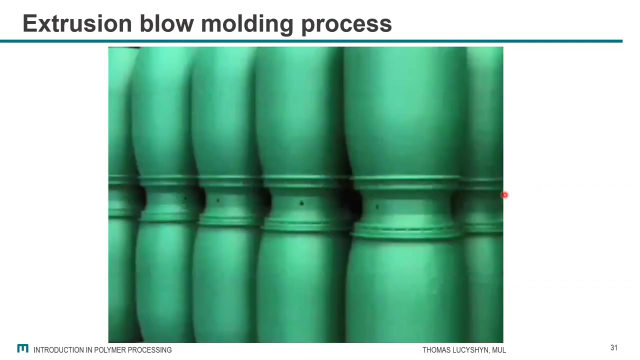 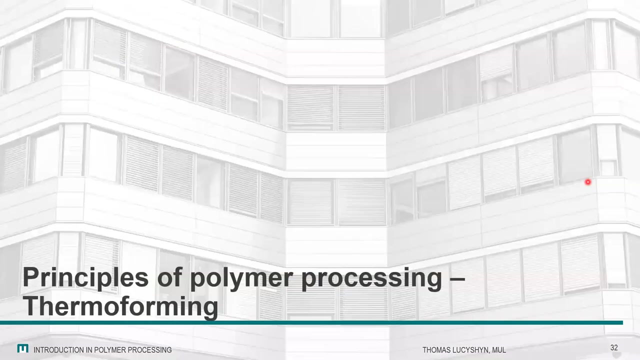 product, but still the extruder works in a continuous way. voila- okay, that's showing the extruder here, the hopper, the barrel with the cylinders in the drive and that's the part. so really huge containers produced in one process step. okay, the next process step, kind of like an. 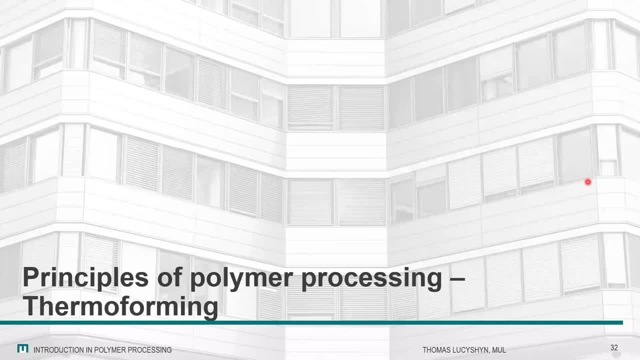 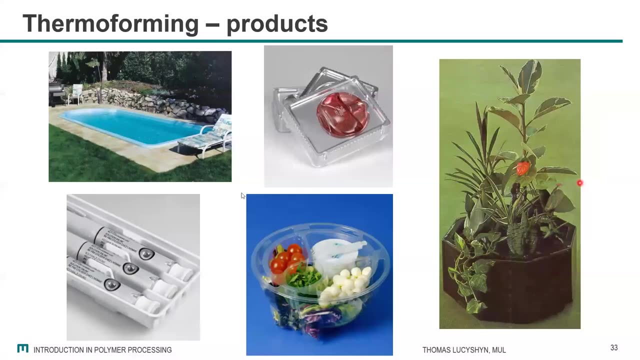 last one that I would like to cover is thermoforming. So typical thermoforming products are rather simple products and are typically for packaging. So packaging of, yeah, of this thing, of food, of course, can also be used for plants And also, in the larger version, also for a whole pool that. 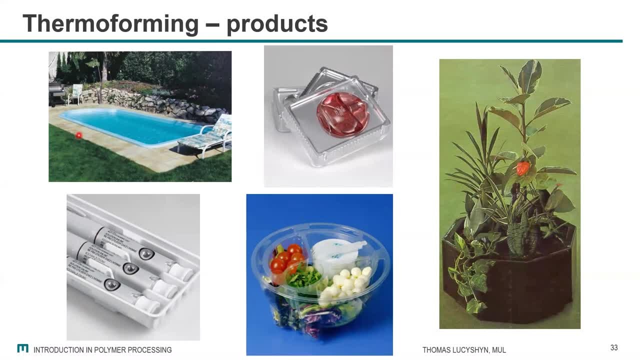 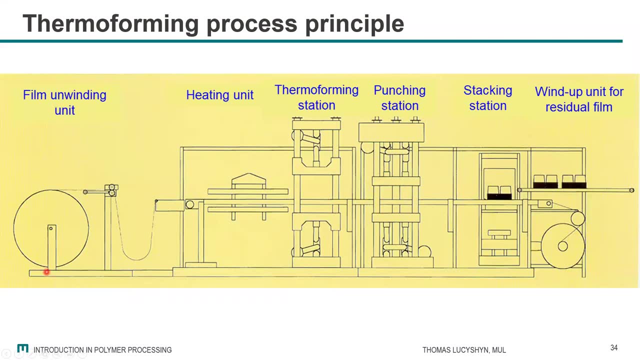 is thermoformed, starting from a sheet, and then it gets the final shape of this. How is the working principle of this process? For thermoforming, you typically need already a first step, like you're extruding a sheet or film, So you need a pre-product which you can then further. 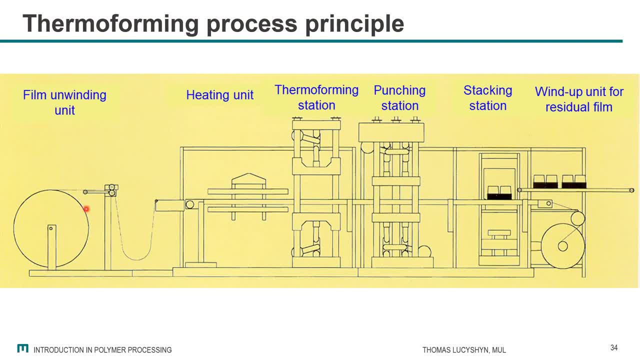 transform into a thermoformed product. So what you have? either you have already produced your film on this big roll, and then this film is taken from the roll, put into a heating unit. So if you want to shape it once again, you have to heat it so that it becomes soft and deformable. 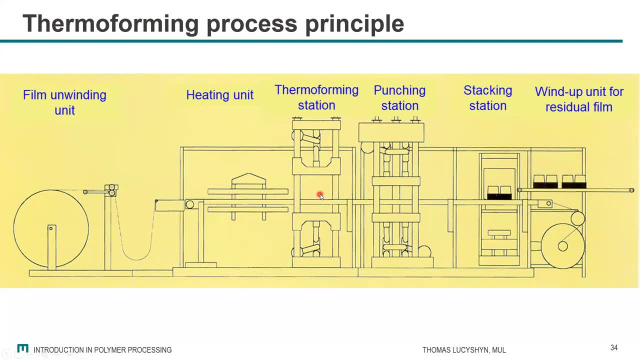 So there is heated And then here is the thermoforming step. So this is the thermoforming station, which I will show you in the next slide in more detail, But basically here the shaping is happening. So the material from this film, from this continuous 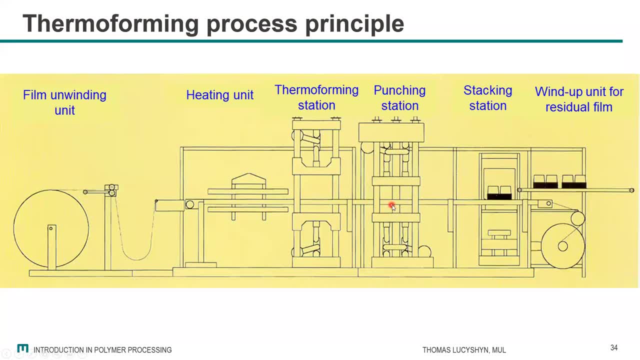 film. a part of the film is deformed And here there's a punching station, So the part itself is punched from the rest of the film And then the parts are stacked here and also the residual unit of the residual film. So the rest which is remaining is taking on here. So just to show you. 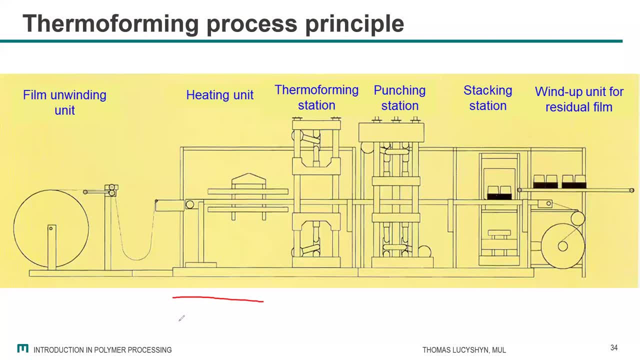 it in the other direction. if the film comes along from this direction, then we might form a cup which has this shape. So here it is shaped. That means that we're getting holes in this film, and this rest of the film is then transported here to this. 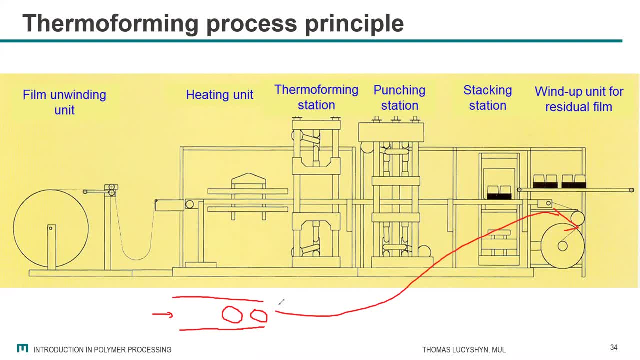 winding unit, And this is the residual material, which is the rest of the material, which can of course also be recycled internally, because it's a pure material. We don't have to separate it from anything else. That's the easier part of internal recycling. 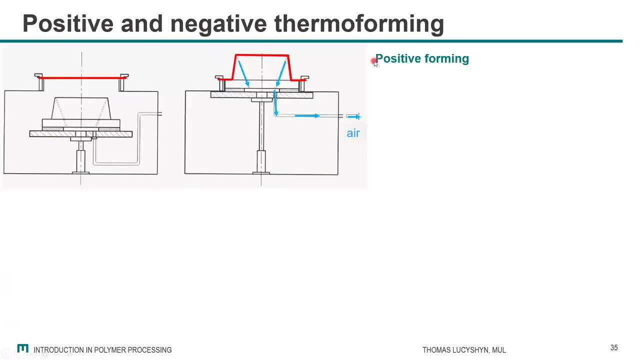 In the thermoform we can distinguish between so-called positive or negative thermoforming, depending on the shape on which side you're forming it, because the thermoform is a one-sided forming, So on one side the shape is quite defined and on the other 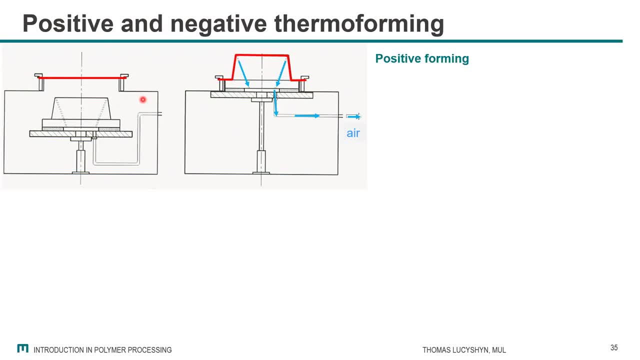 side it comes out how it looks like because there is no active possibility to influence the shape. How does it look? So, in principle, you have the film here in a frame, fixed into a frame, and then this is the finished picture. 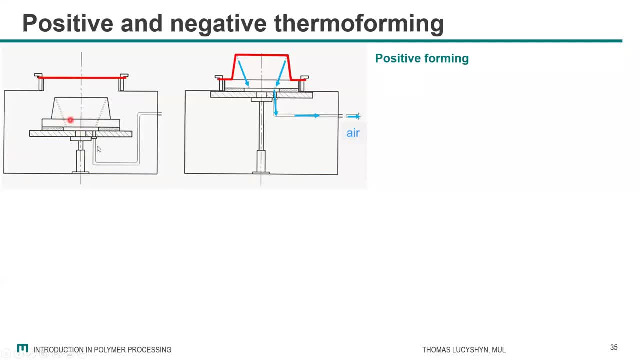 forming the mold, which is typically quite a simple mold. Then this mold is moving upwards, getting into contact with the film And then you can see here there are holes in this mold, small thin holes or channels by which you can suck the air out of it. So basically, you form a vacuum. 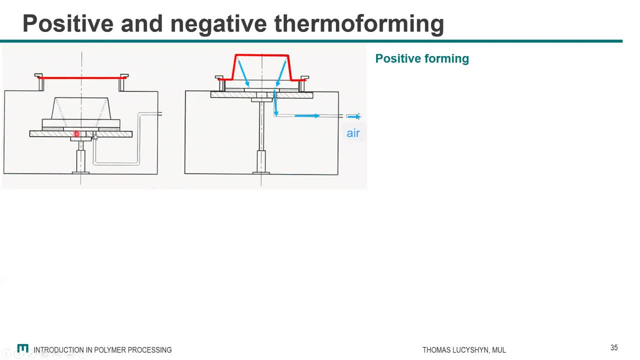 So if, once it gets into contact, there is some air and you suck the air into here by these channels And by sucking the air in, you produce a vacuum which sucks basically the film over this shape, So it really suck it over the shape. And now this is positive forming because the shape 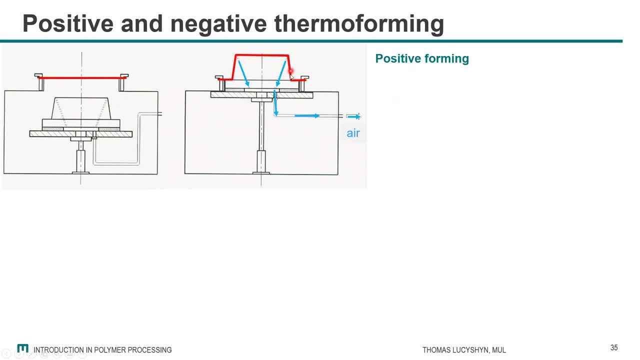 protrudes out of the surface and it's pulled over it And that means that the inside of the part, as you can see here, the inside of the part is in contact with the mold, which has a very defined shape. So if you want to have a very defined shape of your dimensions in the inside of your product, 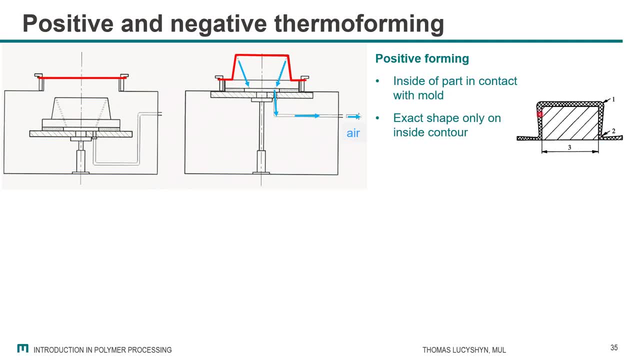 then you need to use positive forming. Whereas the outside has some kind of undefined shape, because it's really. you have not a big influence on what is happening on the outside, But on the inside you have a very exact shape of your mold And also the thickness distribution is different. So what comes into 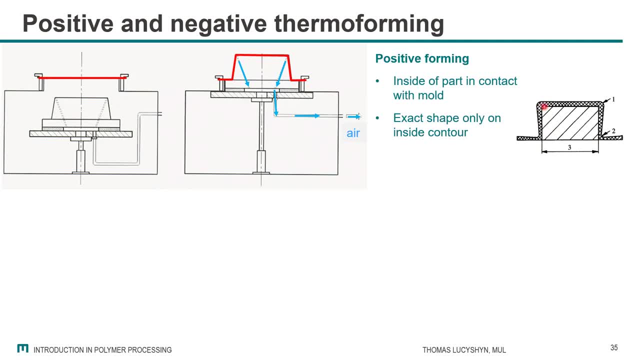 contact with the mold in the first step will freeze and then cannot be deformed so much And then it becomes thicker And that would be the part that would be stretched last. So just imagine you're starting to stretch the material over this mold. Then this part would. 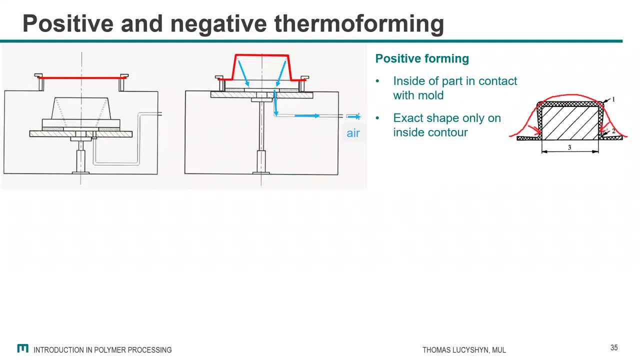 be the last- which is deformed and has quite a large deformation And then therefore it's stretched a lot and therefore the material becomes thinner in these regions. If you want to have the outside shape in a quite defined shape, then you need to go to 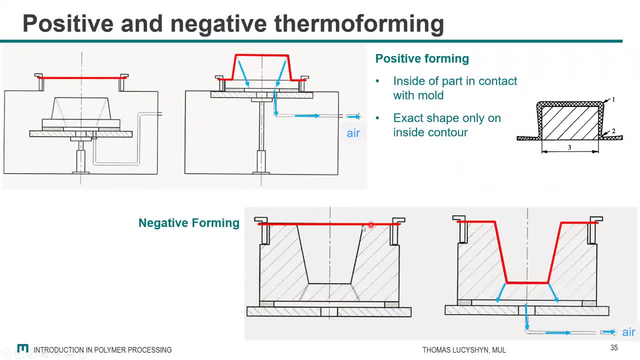 negative forming. It's just the opposite. Once again, you have the fixed sheet and you have the shape inside and you suck the not over a protruding shape but to the inside. So the polymer is sucked here by vacuum. So if you apply vacuum here by taking out the air here, 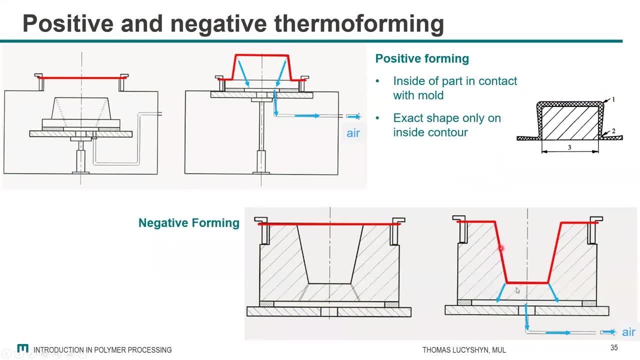 then the polymer film. the soft polymer film is now sucked into the shape of the mold and forms the part. So the characteristic of negative forming is that in this case the outside of the product, so this would be our product, like a cup, then the outside of the product would have contact with the 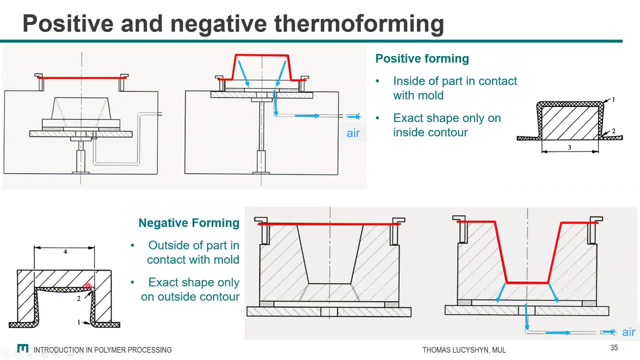 mold And then you would have an exact representation of the shape of the mold on the outside And on the inside of the product. you would have some kind of undefined shape And once again we have a different thickness distribution. If you compare it like here: 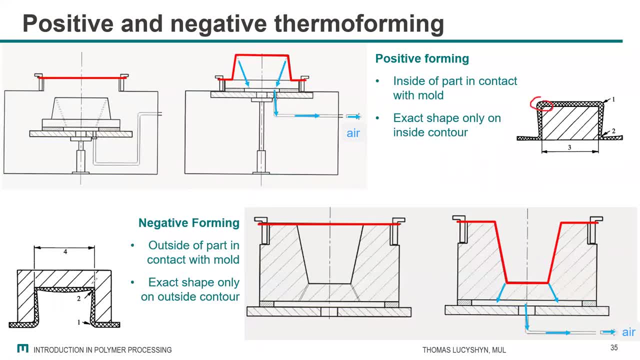 here we have, on this corner, we have the thickest region And here, for this part, in this corner, we have the thinnest region. So it's the same position of the product, but that depends on the production method. So here we have, you can imagine, here is the. 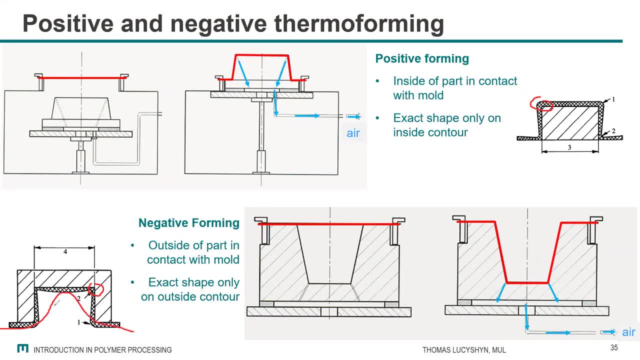 stretching going on Like here, you suck it in, and then this would be the part that is pulled here by vacuum at last, So that one will be stretched most. And then stretching most means that it's also stretched in this direction: it becomes thinner. So this: 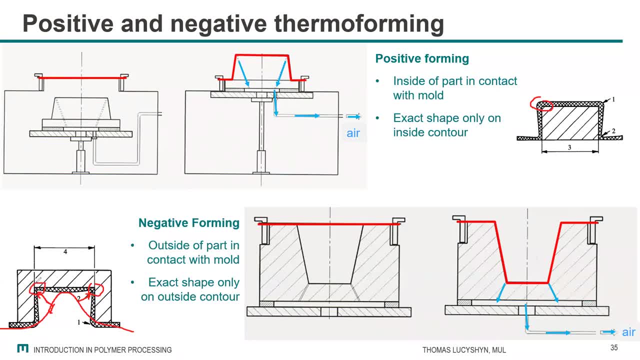 part would be the most stretched part of the product And therefore you get the thinner regions there. So once you want to produce a part, you need to know where you need your exact dimensions And based on this you can decide if you go for positive or negative forming. 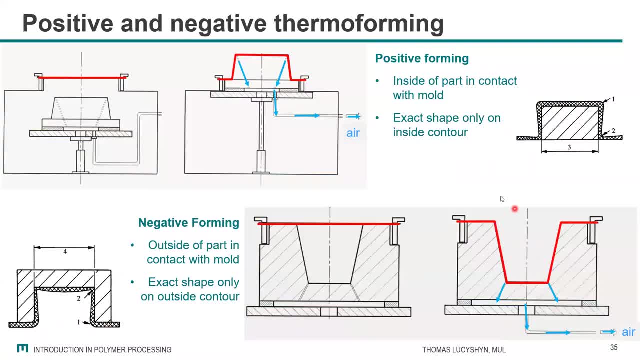 All right, then let's go. So, basically, this is also the geometry. as I said, the geometry on the outside is not very much defined. So if you need really very precise parts on all sides of your product, then you really have to go for injection molding, which is a lot more complicated. 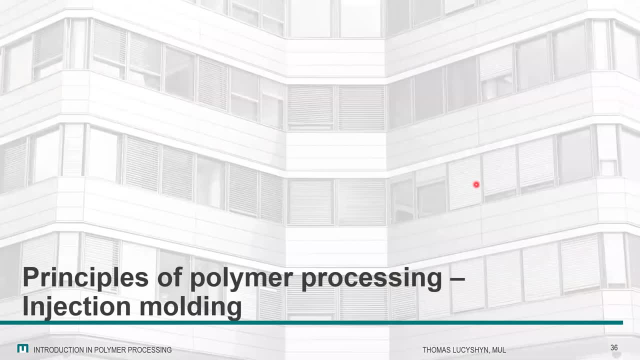 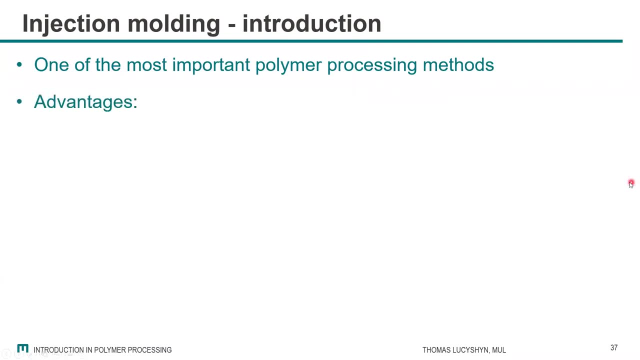 and also more expensive. regarding the molds, more complex. Injection molding in general is one of the most important polymer processing methods. The advantages are quite obvious. It's a very direct path from the raw material to the final part, So you have one process step. 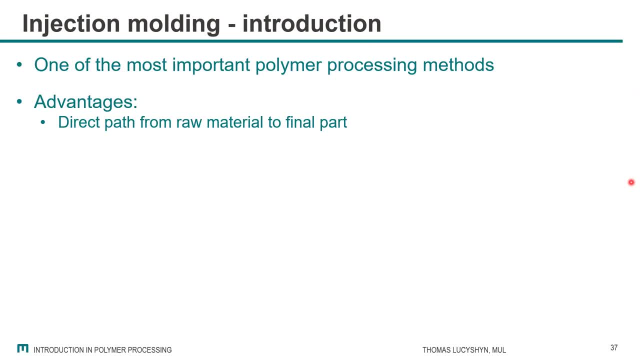 you put in the pellets and at the end you get a part which you can basically sell. Normally you have little or even no further treatment of the parts, So the part falls out of the machine ready to use And it's also possible to use really fully. 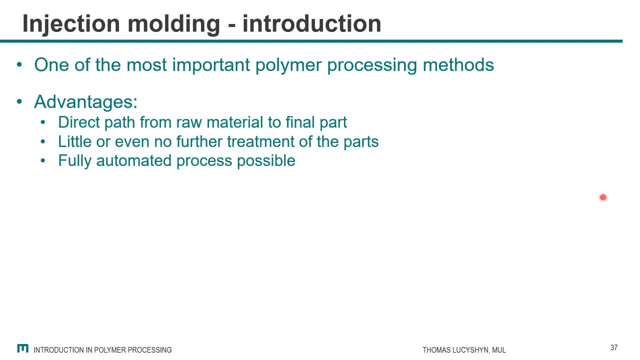 automated process. That's why, also in Europe, we have quite a lot of injection molding happening still, because there's not too many persons involved And also what's really good is you have a very high reproducibility of the process, even at very large numbers. So it's 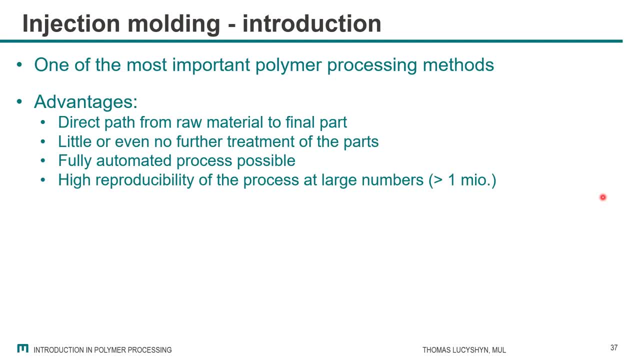 a process which is intended to be used for mass production, not for 10% parts. Injection molding would be way too expensive. The part range is very wide, so it can range from very tiny gears in the range of one milligram, like this small gear in. 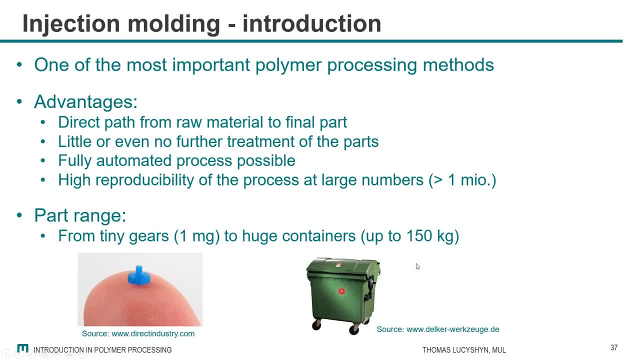 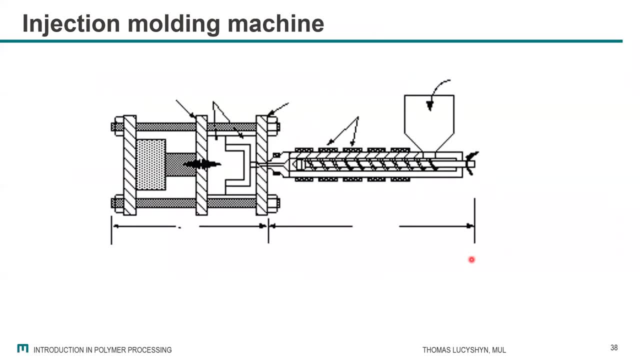 comparison to a thumb, up to huge containers, up to 150 kilograms, And of course the size of the machines is of course then very different. I would like to show you the principle of injection molding. So that's a principle sketch for such a machine. So on the one hand we have the silk. 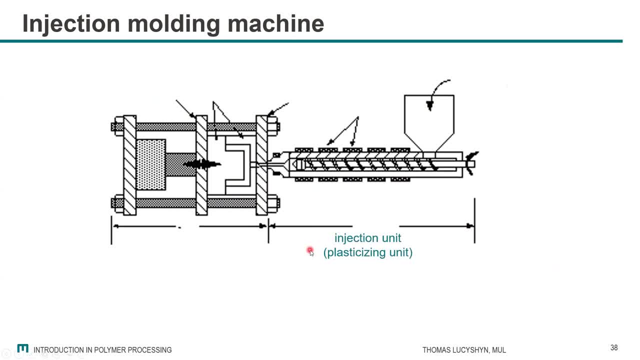 called injection unit or plasticizing unit, And on the other hand, we have the so-called clamping unit and they have different functions. in the process, Starting with the injection unit, we have again a barrel. So it's quite basically it's an extruder on this side with a barrel. 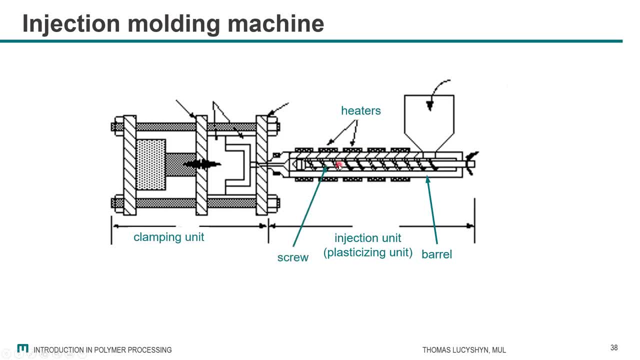 some heaters outside- and the screw. The difference between extrusion and injection molding is that in extrusion we have a continuous rotation of the screw and then conveying continuously the material out. In injection molding the screw is not continuously rotating, but it's also actually. 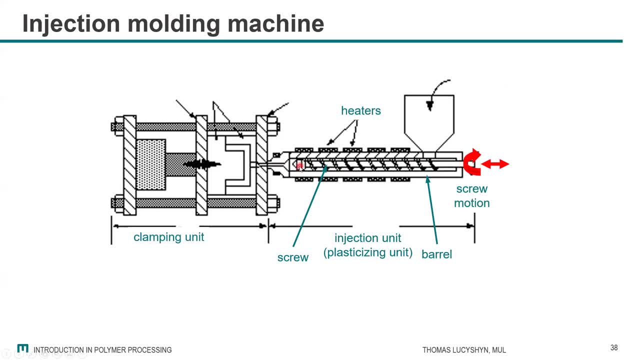 moving. So typically, before a new part is produced, the screw is moving backward, collecting material in front of the screw And then in the next step, the screw is acting like a syringe and pushes the material through the nozzle into the mold. That's why it's also called injection molding. 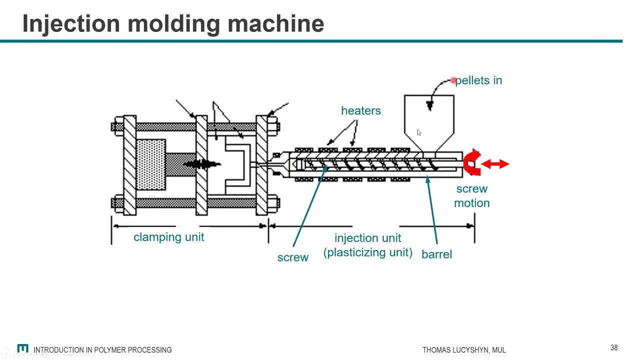 machine, The pellets. here's the hopper again. Here the pellets are coming in. Here they are coming in. They are melted and in the front we have homogeneous melt which is then further processed into the mold, The clamping unit. we have typically one fixed platen and one moving platen, And attached to 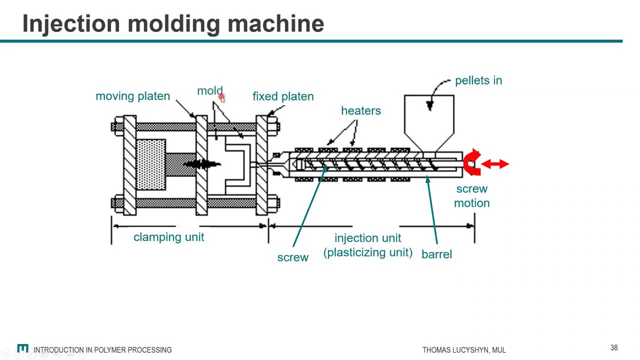 these two plates. we have the two mold halves, So a mold consisting of two mold halves forming the cavity. So these two halves are forming the shape of the final product. And then the moving mold half is opening and closing. So this one is moving back so that you can demold the part. 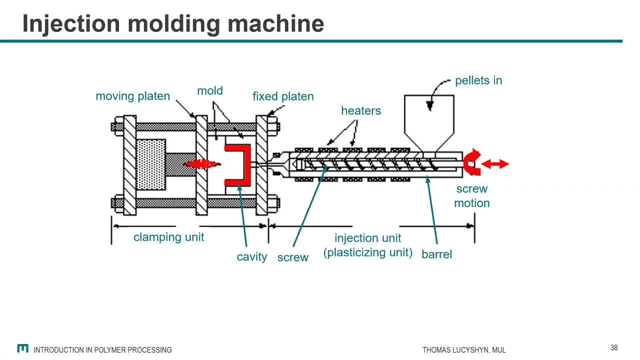 And then it closes again, so that it's a closed volume which is then filled with the melt. Additionally, we need to temperature control the mold. So, depending on the material which we are processing, we need a defined temperature If the mold is too cold. 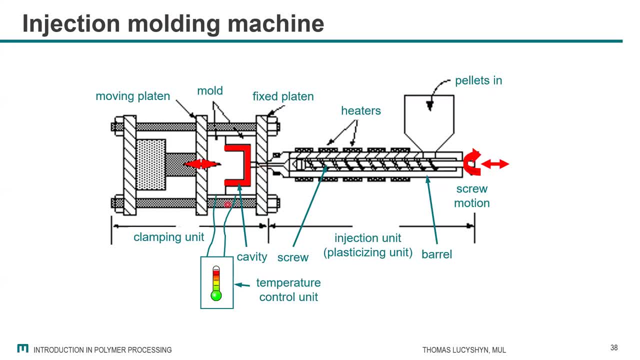 the material would freeze too early and we could not fill it. If the mold is too hot, then the cycle time is too long, the productivity is bad and also the surface quality would maybe not be the best. So we have to find a good compromise between quality and productivity. So this is how such a 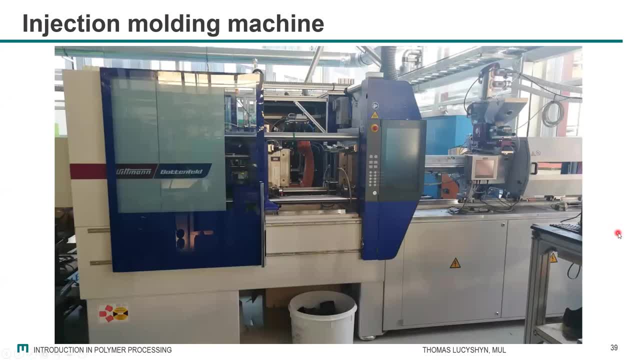 machine looks like in reality. So this is an injection molding machine in our labs, very modern one from Wittmann-Buttenfeld. You see, here, that's the barrel with the screw inside which you don't see. basically, here There is the hopper. In that case we have an automated conveying of pellets into the hopper. 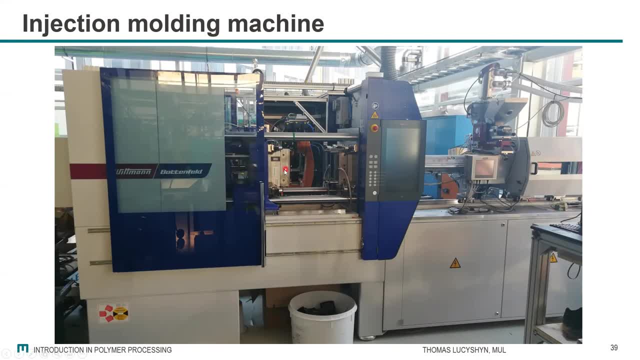 with a gravimetric feeding. And then here we have the two mold halves. So there's one mold half, there's the other half now in the open stage, And that's how it looks like. To give you an impression of the size of the machine, I added the size of a person here, So that's typically the size. 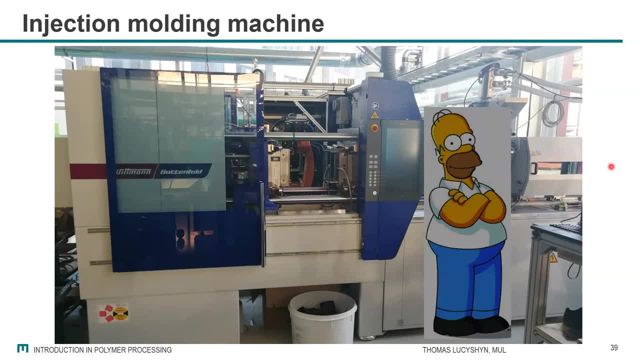 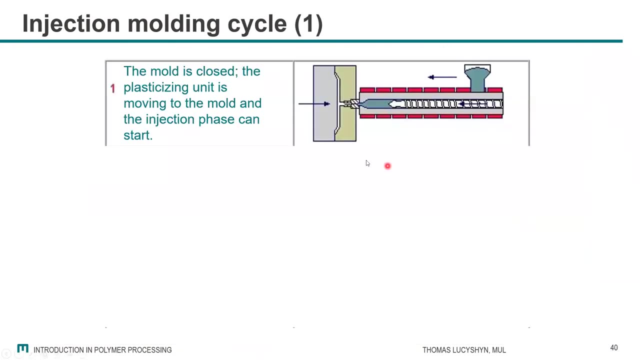 of this machine, And this is for a range of, I think, 1,100 kilonewton or 110 tons machine, So it's an intermediate machine size. How is the cycle running? So what's the typical cycle of injection molding? So 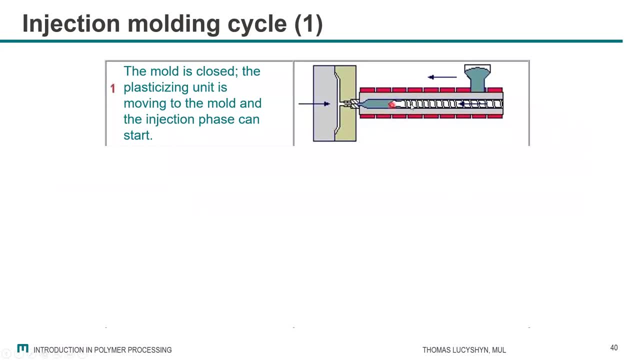 the starting point is like the screw is typically in the back position, So in front of the screw we have already collected melt for the next product. Then the mold is closing, The whole injection unit is moving to the mold and getting into contact to have a tight contact. 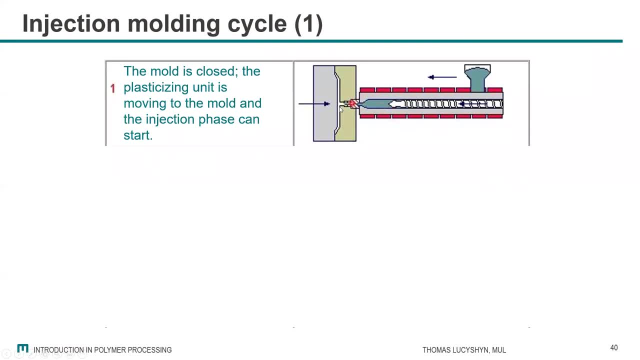 With the mold And there is a channel from the injection unit into the mold And then the injection phase can start by moving forward of the screw. So the screw moves forward, acting like a syringe, pushing the material through the channel into the cavity until it's completely filled And 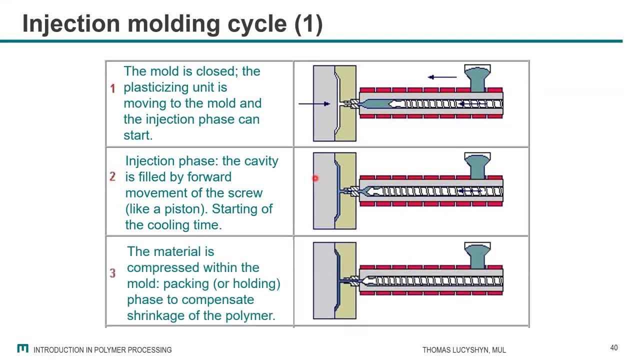 now we have to add another step, because polymers have the property that they're shrinking quite significantly when they're cooling. So typical shrinkage ranges are linear shrinkage of like up to two and a half percent. That means, you know, two and a half percent of the material is 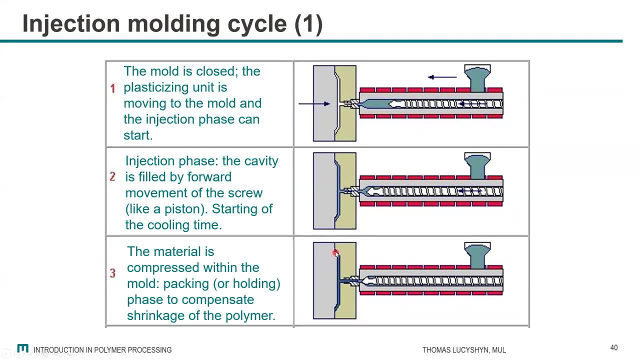 shrinkage. That means if the mold has a dimension of 100 millimeters and you put the hot melt into it, once it cools down to room temperature, the final product will not have 100 millimeters but maybe only 98 millimeters. So you have to consider that in your mold construction. 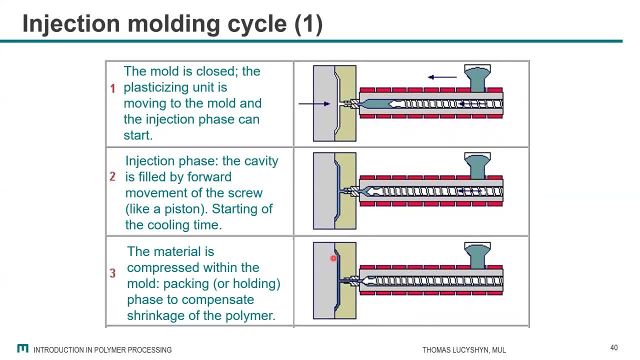 That means you have to basically increase the size of your cavity in order to achieve a final desired shape of your part And in order to compensate this shrinkage which is happening, what you can do is you can press some additional material during the shrinkage. 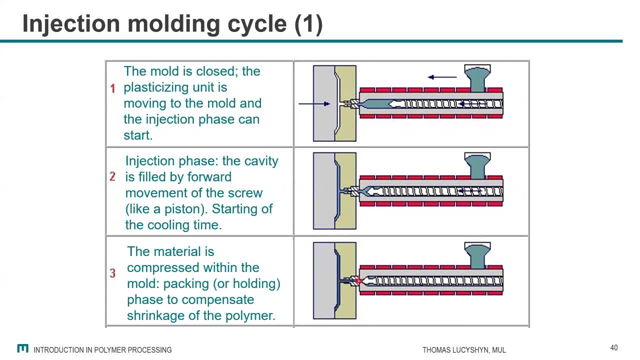 during this cooling phase as long as the material is not frozen yet. So if this channel is still open, you can still push more material in, which means the density increases, the shrinkage will be compensated and you will not get so much shrinkage. But once there will be a point where 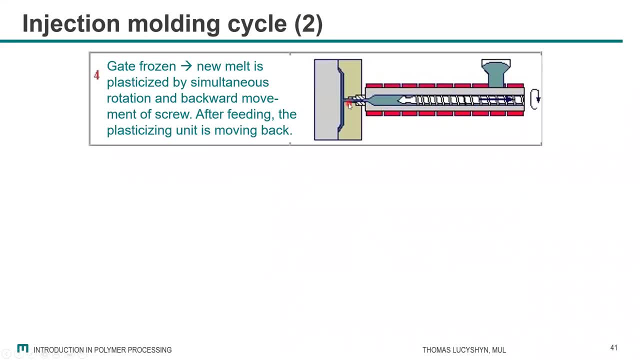 the gate, the channel will be frozen, So material cannot flow anymore. You cannot push any more material into the cavity. And that's the point when you start to feed again, to move the screw backwards by rotating it and conveying more material. And that's the point when you start 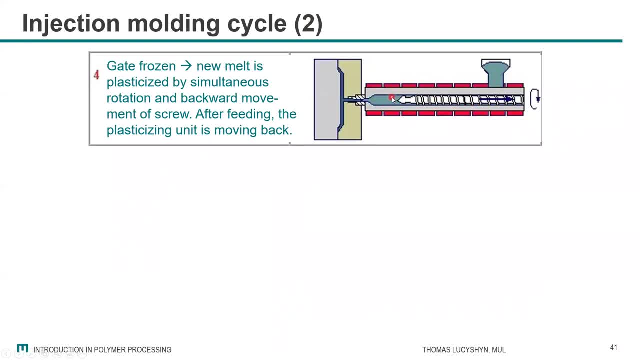 melting material and conveying it to the front so that you're prepared for the next shot. Then you typically need some more time for the part inside to be cooled down sufficiently so that it's rigid enough that it can be safely demolded. Then the mold opens, the part is demolded, can be. 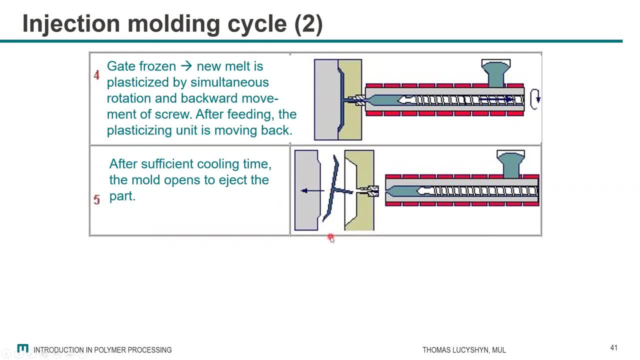 taken by a robot can just fall down, taken out manually, whatever, And then the cycle starts again. So mold closes again. injection unit moves forward, injection unit, the screw, moves forward and injects the part. So this is running in cycles, It's a discontinuous process. Regarding cycle times: typical cycle. 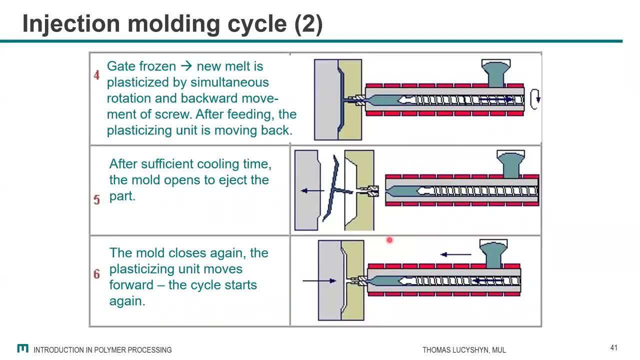 times range from very fast processes of small closure- caps of bottles, for example- we are in the range of a few seconds, two or three seconds per cycle, And we have multi-cavity molds. So in one mold with not only one cavity, like up to 128 parts can be simultaneously molded in one step. 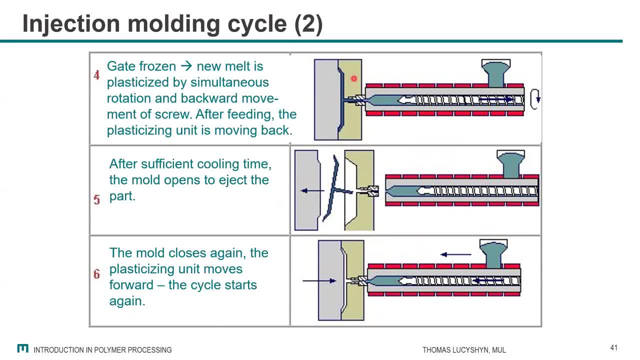 And this every three seconds. the mold opens and throws out 128 parts, So it's a huge number of parts that can be produced within basically one day. This is a short animation how it looks like. So the mold is closing injection. 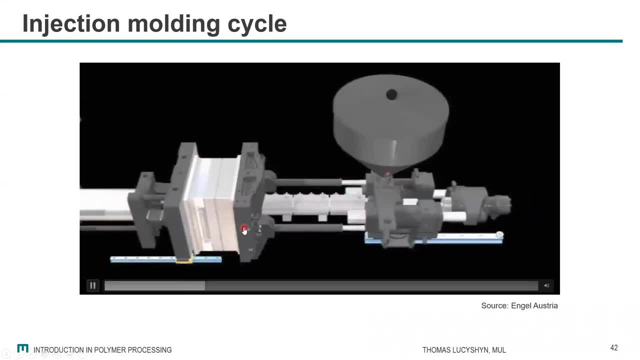 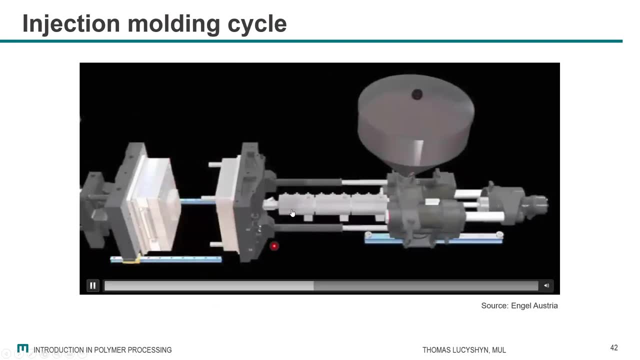 unit gets in contact with the mold, Then the injection happens, cooling, feeding, moving back. mold is opening, the part is ejected And now we are looking into the injection unit. So the mold is closing again. The injection unit is in contact with the mold. 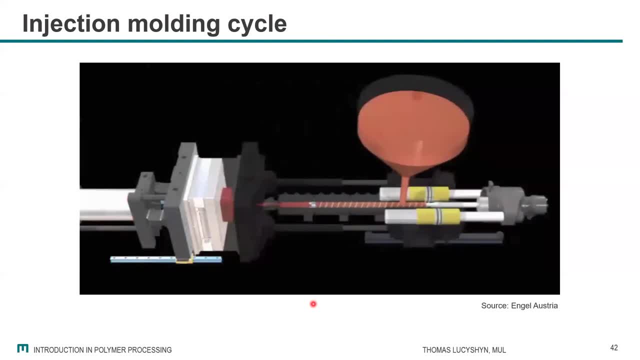 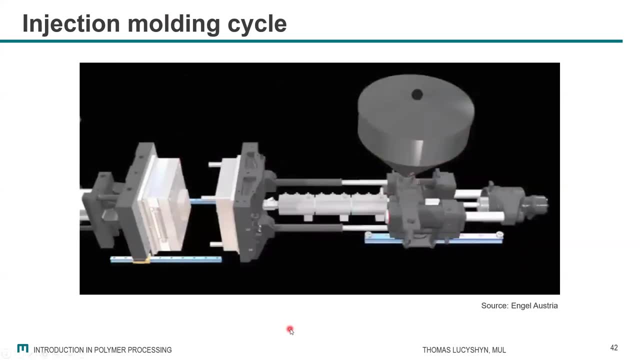 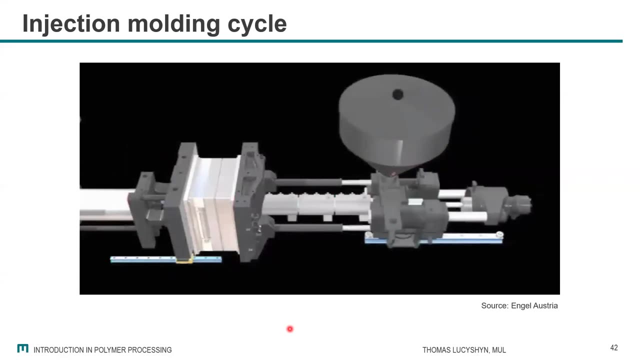 Injection phase. packing is quickly feeding, going back, opening, demolding, So packing phase is here very short. You don't see them very much in the packing phase, So maybe repeat again. So mold closing, moving forward of the injection unit, injection packing, feeding, cooling, opening. 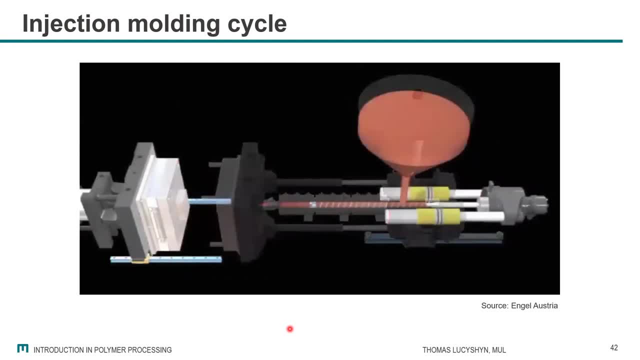 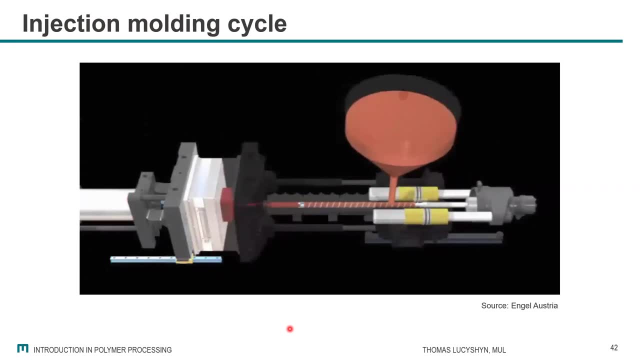 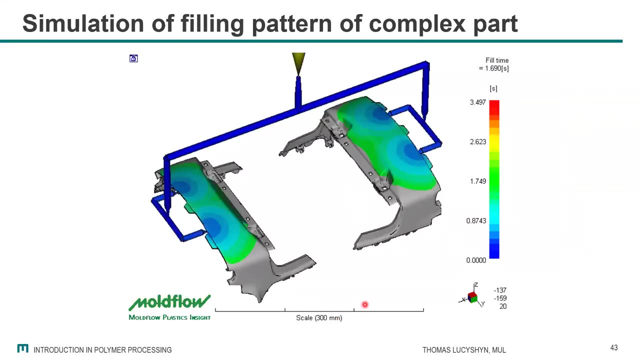 demolding And once again look looking inside: closing injection, packing very short feeding, moving back and so on. This is one possibility to look inside the cavity. What is happening there is. we're doing a lot of simulations So it's possible to simulate the filling phase, having a look at the temperature. 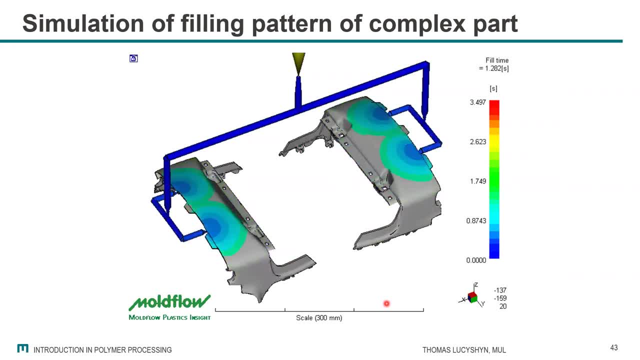 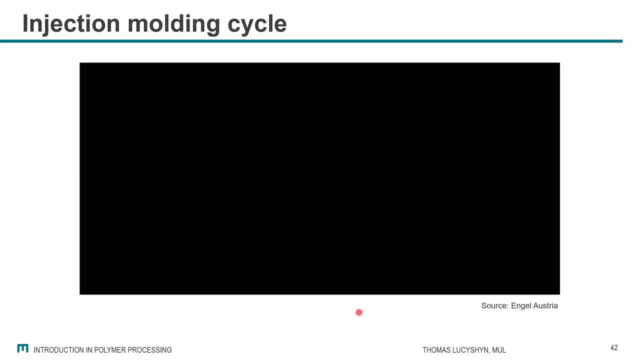 conditions, also a shrinkage and warpage, And this is a nice possibility to do some front loading. Otherwise such a mold for a machine can be quite expensive, can even be more expensive than the machine around. So if you produce a mold which does not work then you're going to have to do a 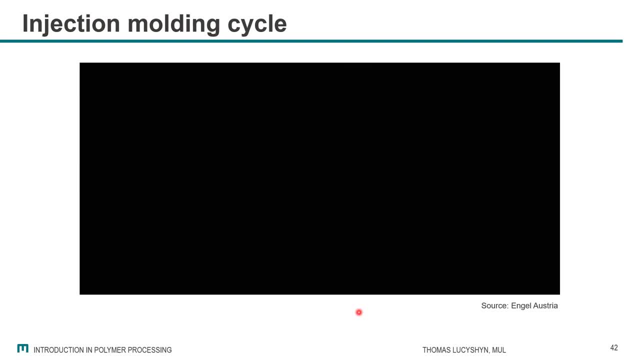 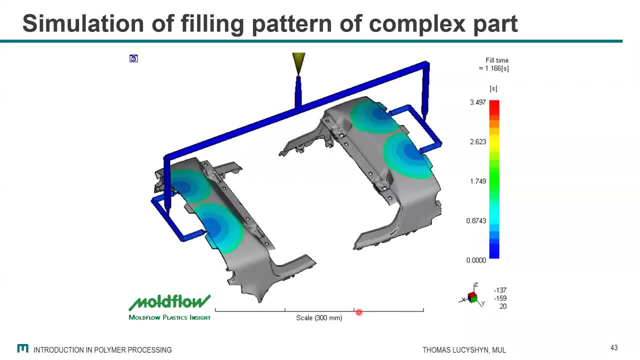 simulation, It's quite a lot of time and money wasted. So if you can use simulation in advance to recognize potential errors, you can optimize your process and your product before you build a real physical metal mold. Okay, the last process I would like to show you. it's really gaining. 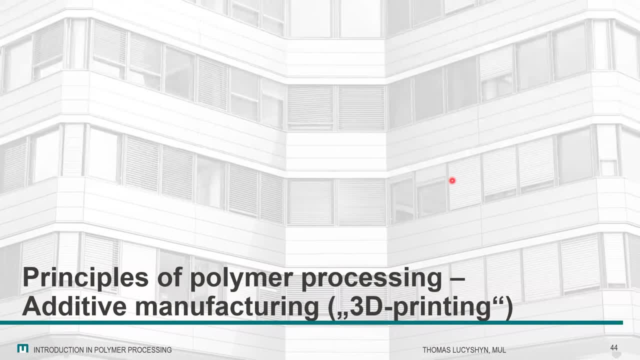 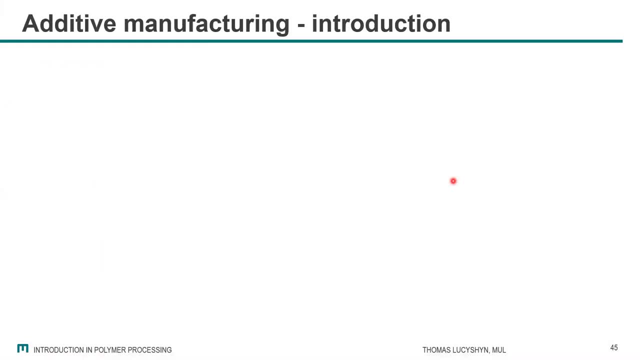 increasingly more importance. It's the so-called additive manufacturing, also known as 3D printing, although this is one term for many processes. Some introduction: So why would you want to use additive manufacturing compared to other conventional processes? It's, of course. 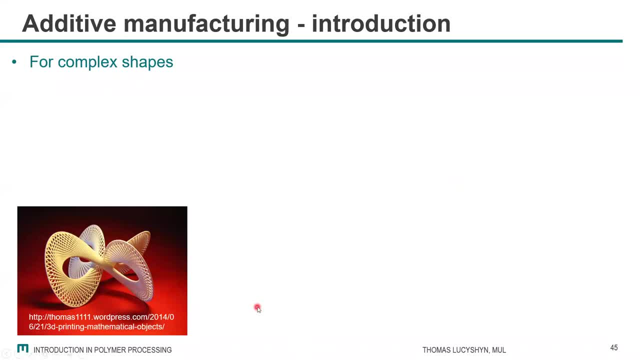 really enabling us to produce very complex shapes which you cannot ever produce with conventional methods. It's also about individualization of single products, So if you want to have this helmet produced, this one in this shape and color configuration and the next one in the other color- 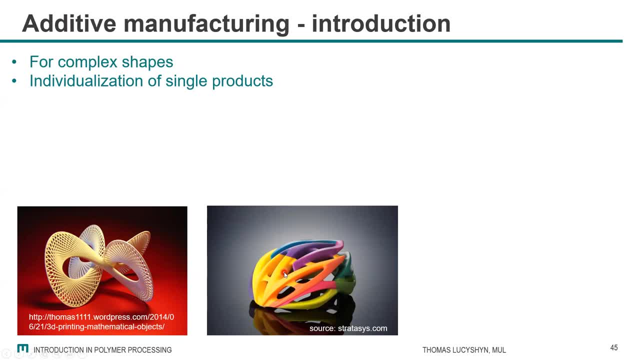 configuration, then you cannot do it in injection molding. So injection molding is really you produce one mold and then you produce one million parts of the same size and shape. You can do the same thing with the color, but not in that way, And it's about a fast realization from the project. 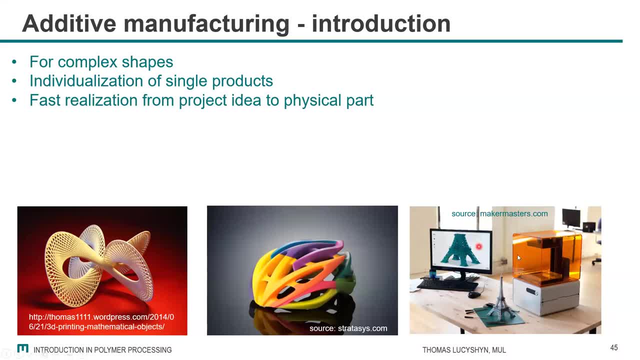 idea to the physical part. You have some CAD drawing, some idea, and then immediately go to the printer and immediately, a few hours later, you have your part. Mind you, fast means only from the realization, from the project idea to the physical part. The production process itself is quite slow. 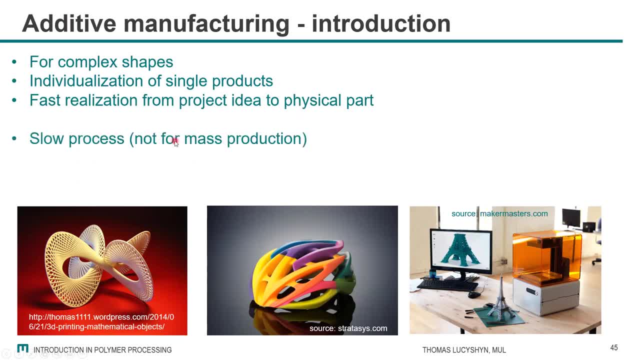 so it's not intended to be used for mass production. I told you, for injection molding we are ranging from like two or three seconds per second cycle up to like in the range of minutes for very big parts, And here we are talking about hours for. 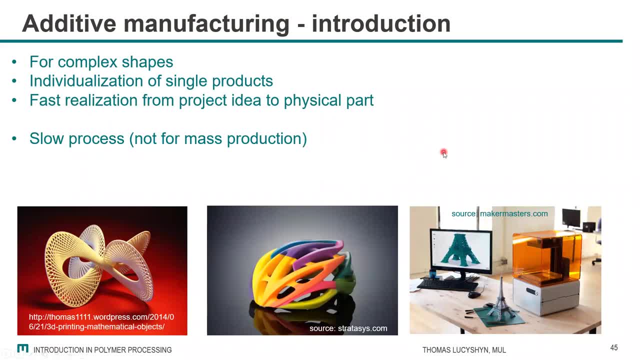 a single part. So that means if you intend to produce one million of parts, maybe 3D printing is not the right choice, So you would go for injection molding. But if you want to have a first physical part, you can have this very quickly. Compared to injection molding you have. 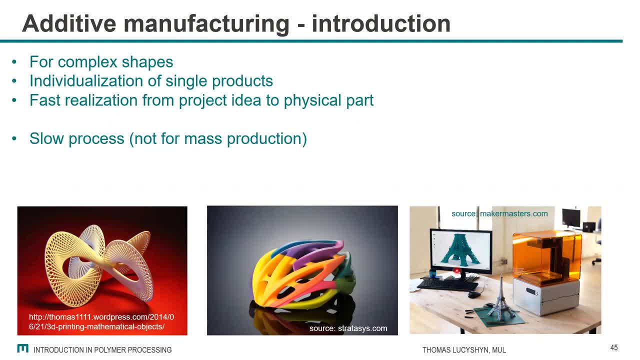 to first design your mold, build your mold, do your first injection molding trials. It can be weeks and months before you get your first part. So that's the big difference and big advantage of additive manufacturing. Currently there is still a limited number of materials, so you cannot use all the materials. 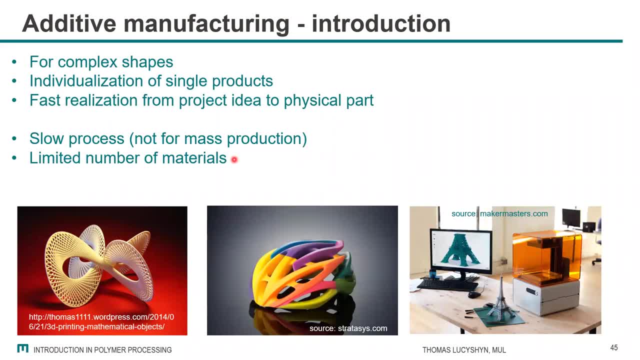 which are used in conventional processes, So, for example, highly filled materials, glass fiber, reinforced materials. it's quite limited to use them And also in general the quality is not comparable with conventional processing. It means that the surface quality is not the same and also the mechanical properties are typically not the same. 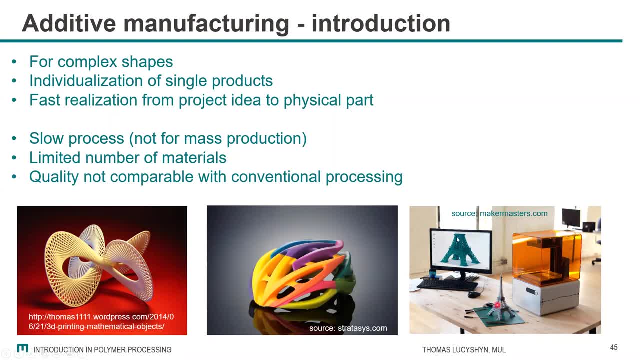 So it's more like for having a prototype seeing how it looks like, also maybe for repairing something. it would be a nice hybrid approach to produce something in injection molding and then doing some additional additive manufacturing onto it. It's a very nice and interesting method and process, but still there is a lot of development to be going on. 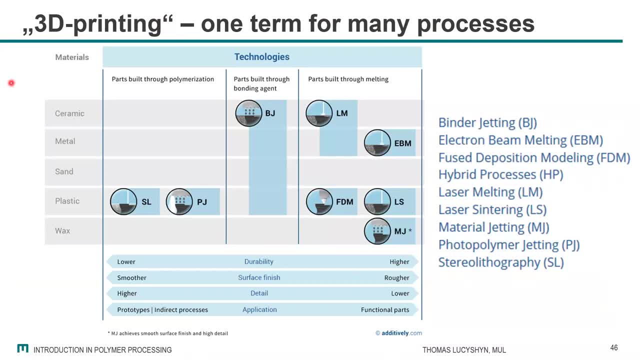 3D printing is not 3D printing. So there are a lot of technologies in this term 3D printing. I would like to just give you a brief overview so you can first distinguish between different materials: Ceramic, metal, sand, plastic, wax and also different technologies. I would like to focus 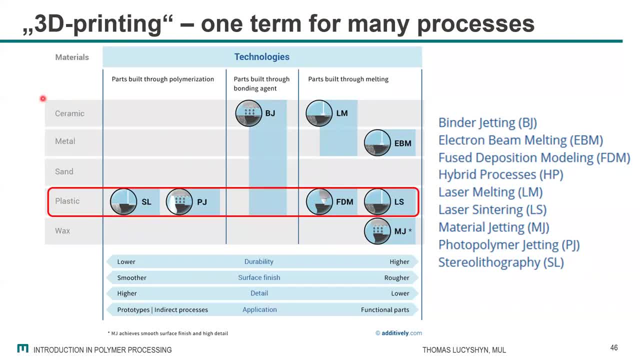 today, basically on plastic, of course, because that's what we were talking about in the whole project, And there we have four major processing methods with two principles. The one is parts being built through polymerization, So this one basically resin based, And then on the thermoplastic. 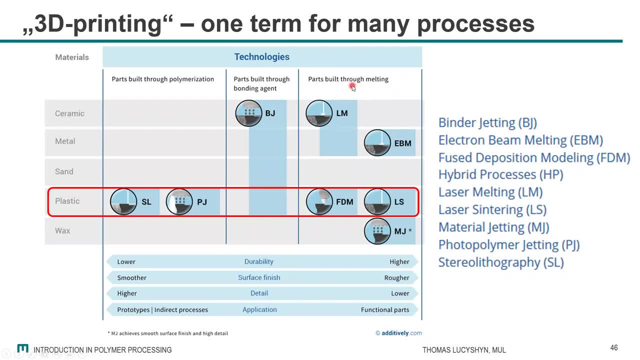 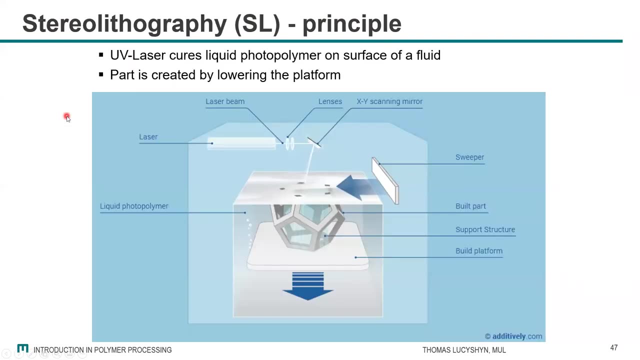 side, we have parts being built by melting. So that's the thermoplastic side, And there are also some effects on the properties. So I'll focus on these four methods here, listed here in the red bar. First of all, the stereolithography principle. Basically, you have a liquid, a resin, 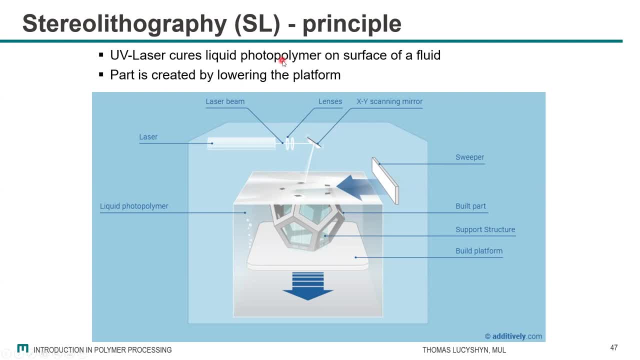 which is a photopolymer which can be cured by applying laser. So what you're doing here is you have a platform, You start your platform here, Then you have a liquid on it which can be cured by using a laser. So at those positions where the laser contacts the liquid- here the material- 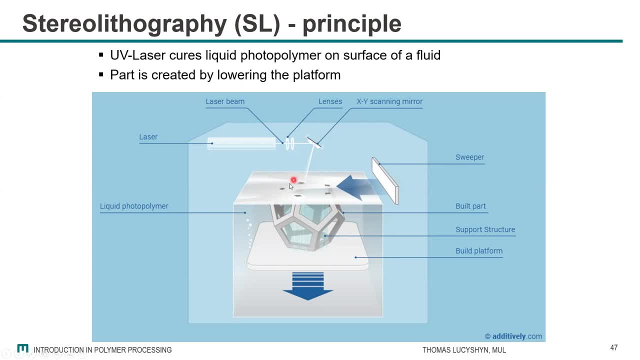 cures and becomes a solid And the rest of the material stays liquid, So only on those local positions where the laser is acting. there we have some transformation of the liquid into a solid And then, step by step, the platform is moving downwards And the next layer 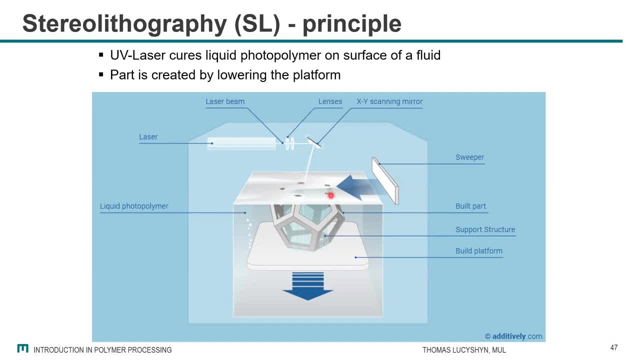 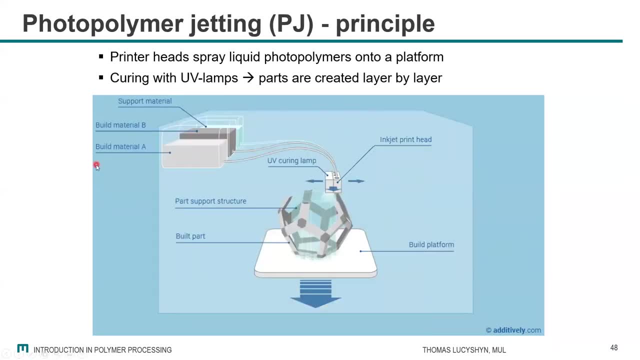 some certain positions are cured And in the end you can kind of create and grow such complex geometries. Another similar project or similar processing method is the photopolymer jetting. It uses basically the same principle of curing a material by using light, in that case UV light. 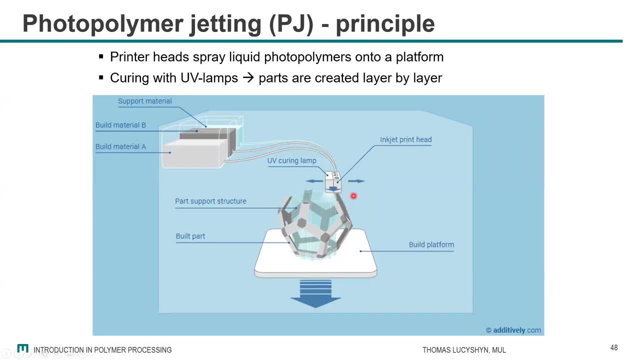 The advantage of this one is in the first one you had a container with one single liquid, So it's one material you can use. In this case, you are spraying this liquid onto a certain surface And then, locally, on these positions where you spray it onto, you cure it by using UV light. 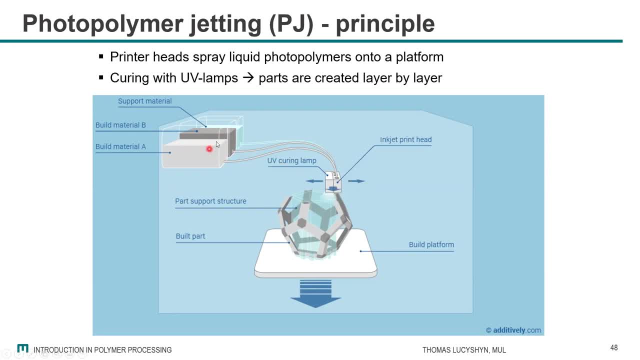 The big advantage is you can use multiple containers of different liquids, Of different materials, different nozzles spraying different materials onto each other. So, basically, you can create materials, multi-material products. The disadvantage of this is it's based on thermosets, So it's in resins which are curing. So, once again, in terms of 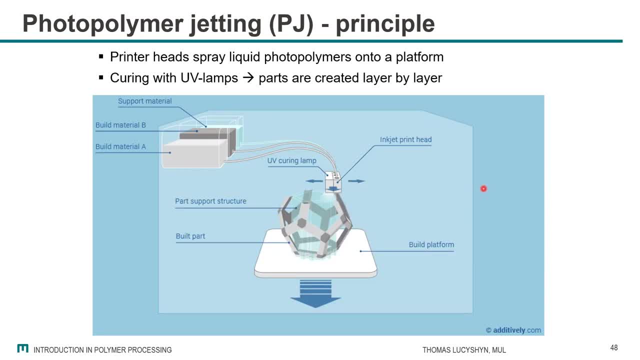 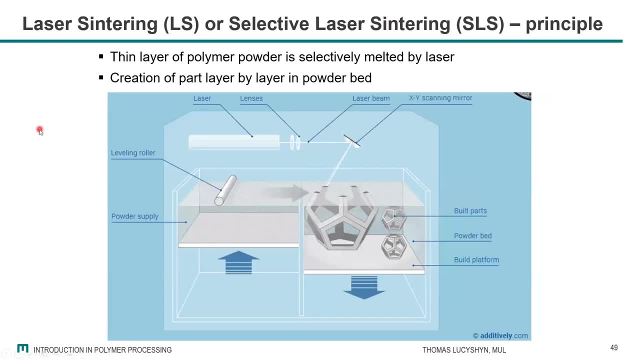 recycling. once they are cured, these chemical bonds are established. You cannot remelt them and reshape them. Now we come to the thermoplastic part of it. So that's the one is the so-called laser sintering, or selective laser sintering, And that's the one that's called the laser sintering. 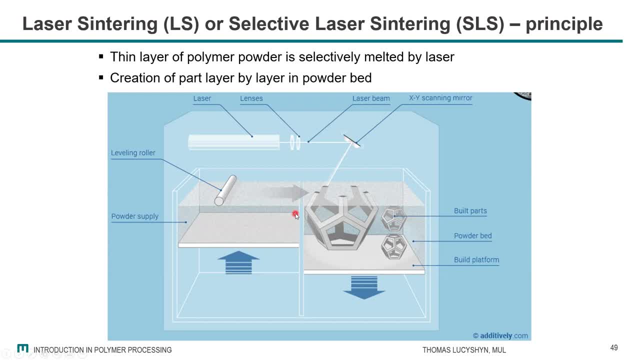 In this case, the base material which you are using, raw material, is powder, a very fine powder, fine-grained powder, in a container. So this is the powder supply And then we have a platform. Then a very thin layer of powder is shifted to this platform And then locally, the powder is. 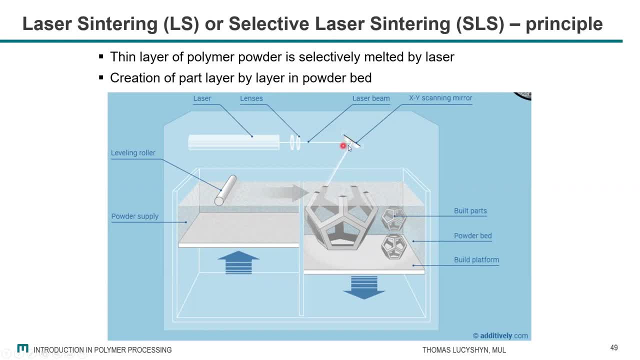 melted or fused by some laser. So here you introduce the laser power And then locally the powder is melted together to a solid material, And then this platform moves down a little bit And the next layer of powder is pulled here, And then locally once again. 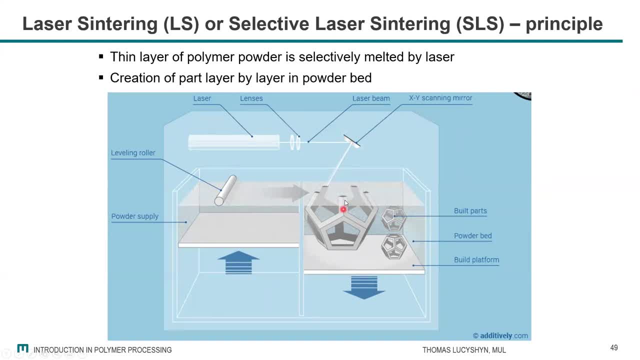 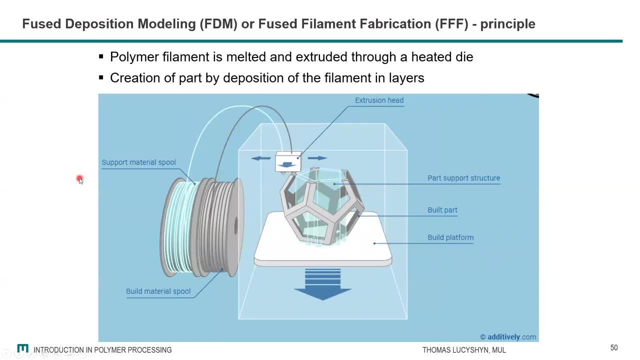 on different positions. you can melt it, the material, and then you get this final shape, And then, finally, we come to the method which we are also mainly applying in our institute. It's this fused deposition modeling, which is basically a brand name, or fused filament fabrication, which is the more general name of this principle. 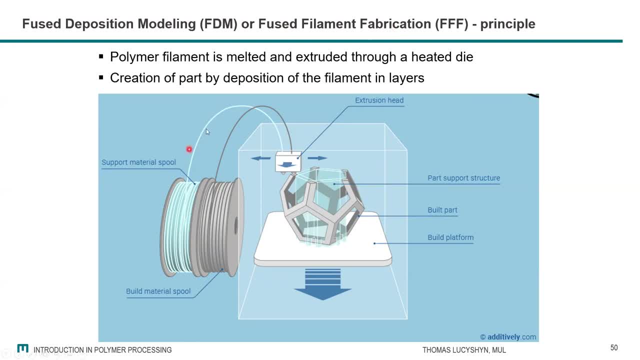 For that purpose, you first need to produce a filament with very tight tolerance of the filaments with in terms of roundness and dimensions, and then this film is on those spools, and then you pull these filaments into an extruder which is heated, so you melt, basically melt this. 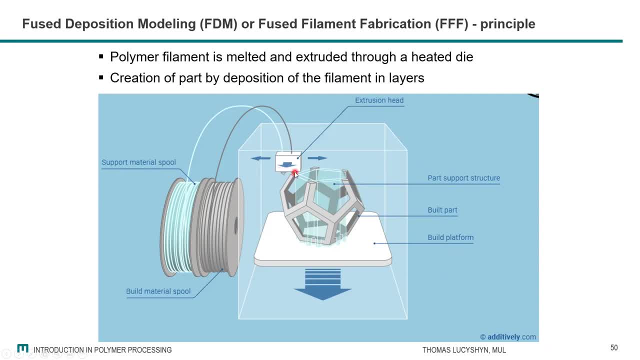 filament in this extrusion head and then you, by layer by layer, you deposit this molten film onto this platform and then by that layer by layer, you can create or produce your part. so the layer, the platform, is going one step below. then the next layer of those filaments is put somewhere where. 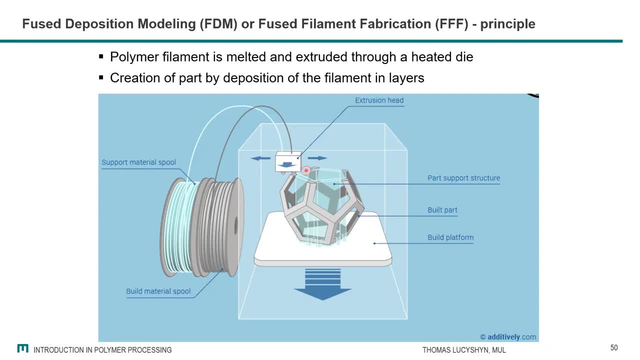 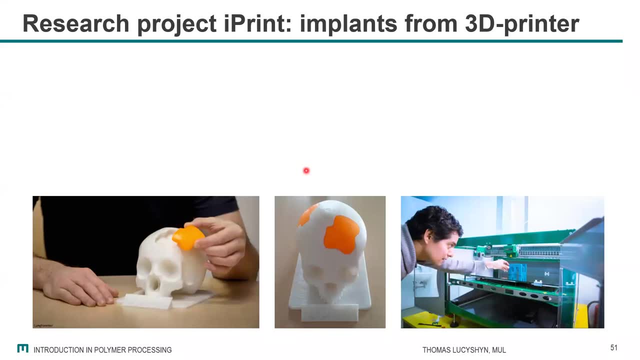 you want to have it and then it's going on like that. i want to show you just one example of a project that we did for this. 3d printing was a nice application for it. the project was called iPrint, for implants from 3d printer. it was used for, like for replacement of bones of a skull, which 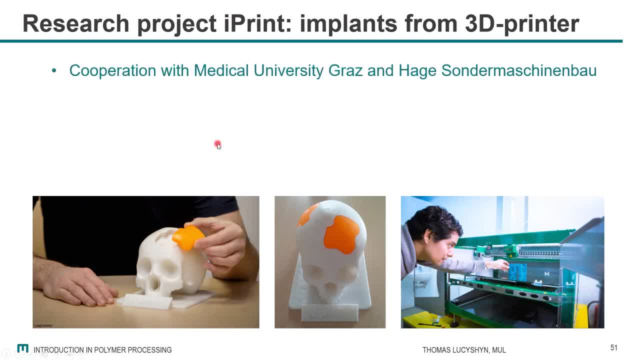 were damaged by an accident, for example, and it was a cooperation with the medical university in Graz and Hage Sondermaschinenbau who produced the printers. so basically the idea was to use to produce the polymer implants during the surgery. so the head is opened and then is. 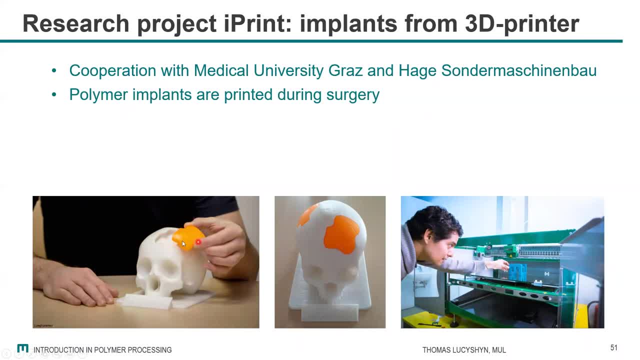 measured and then in the next room the printer works and starts to produce the spare part, if you want so, and this could save a second surgery, because the normal procedure would be: there is a big operation on the head, taking like the geometry. then this geometry is transferred to an external. 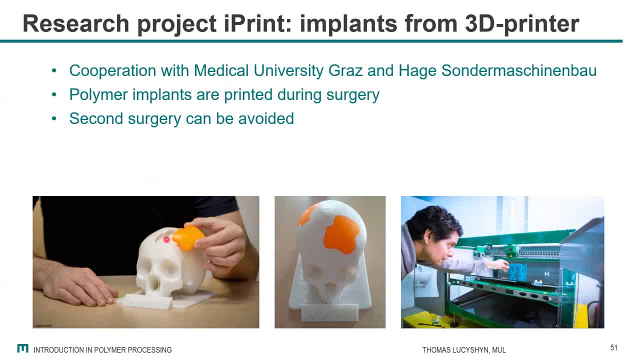 company producing the spare part, which might take one or two days or so, and then the head is something that means, in the meanwhile, the the patient is closed again and there is a second surgery for for implementing the part. it can be tailor-made for each patient, of course, so depending 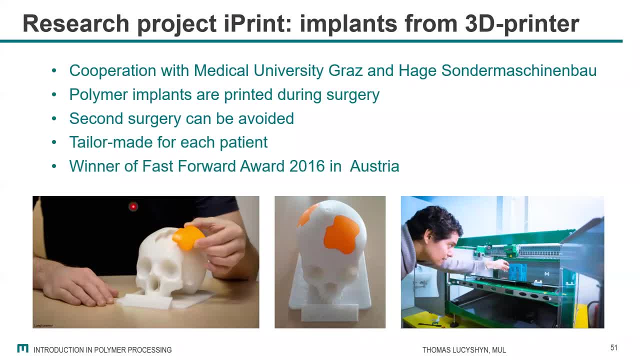 on the geometry. it can be used and you know it was nice. we got also an award for this, for this project and this. this activities are going on. now we are transferring this knowledge to other parts of the body, because the requirements for a bone on the skull is much different from a bone. 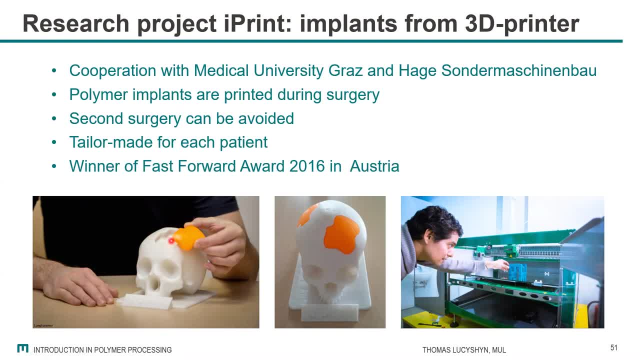 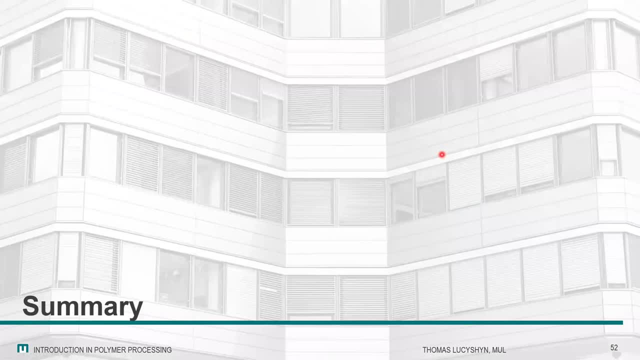 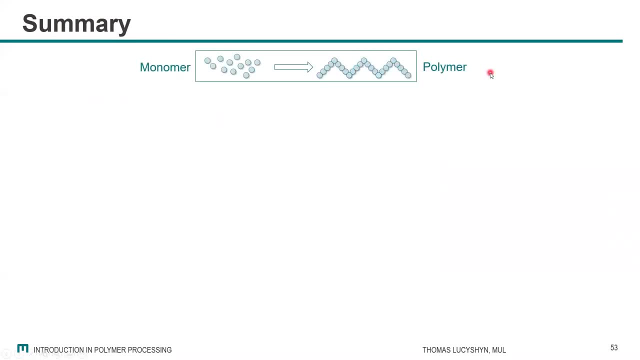 on the rib. so we have different material property requirements and it's quite challenging. okay, this brings me to the end, so I just tried to show you an overview of different processing methods and trying to summarize this. so once again, we start with our polymers. you need to know this chain structure which has some effect. 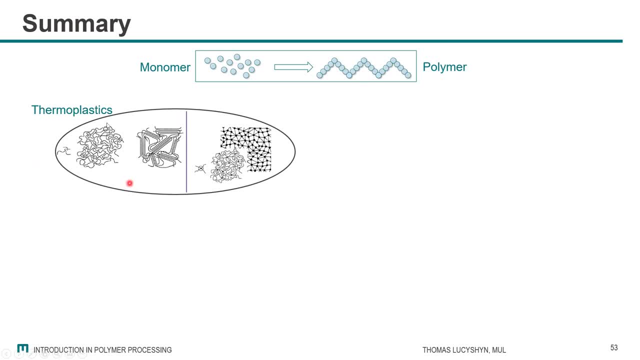 on the morphology. so we have the distinction between thermoplastics, which can be further distinguished between. and then what sets thermoplastics? once again, we have no chemical bonds between the single molecular chain and thermosets. we have those chemical bonds which are irreversible in the thermoplastics. we can 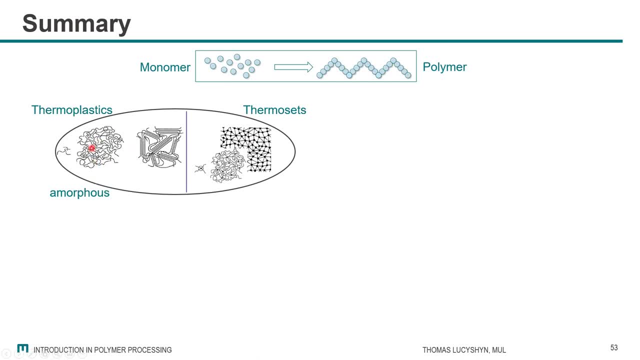 distinguish between amorphous materials, which are very unstructured, and the semi crystalline, where parts of the material are structured in a crystalline way, and for thermosets. if we have very tight network, we are getting durameres, very rigid materials, and if we have very few contact, 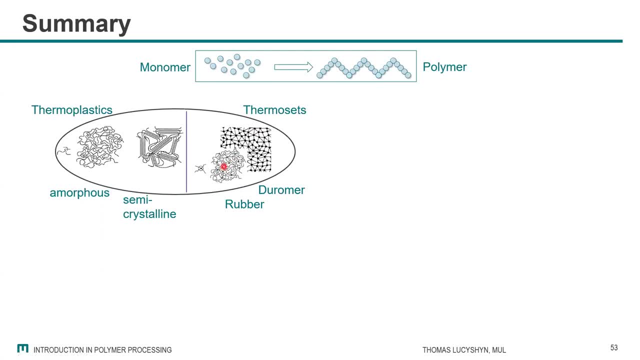 points. we are getting rubber and this has an influence also on the processing methods. I showed you a little bit of different flowcharts. and I showed you a little bit of different flowcharts. so the shear viscosity is a function of shear rate and for polymers, typically we have this shear. 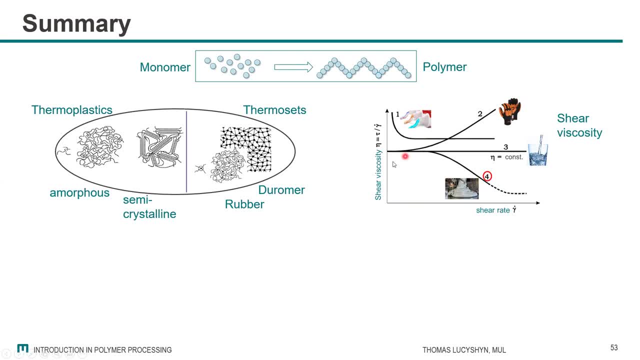 thinning behavior which enables us to basically do injection loading, so that if we're doing a very fast process, the viscosity goes down and therefore we can have a low viscosity which is enabling us to fill small gaps. I showed you the principle of an extruder with the screw inside, heating it melting. 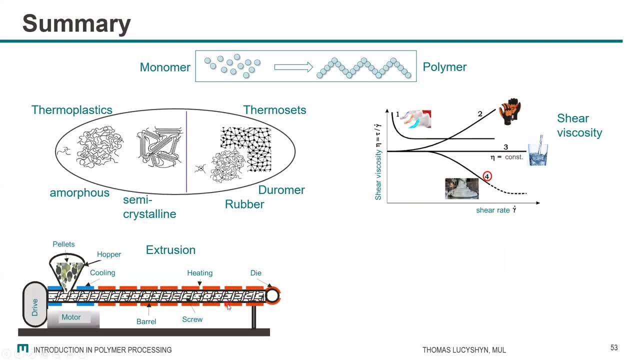 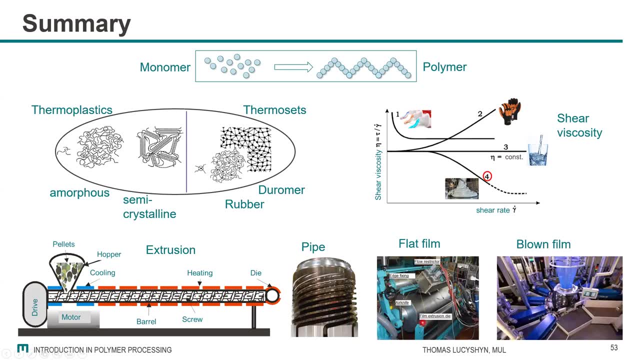 it and squeezing it through a die and depending on the die, you will get different products. either you can produce pipes, you can produce flat film, we can produce blown film, depending on the die and the follow-up periphery you use. I showed you the principle of blow molding. you have an extruder. 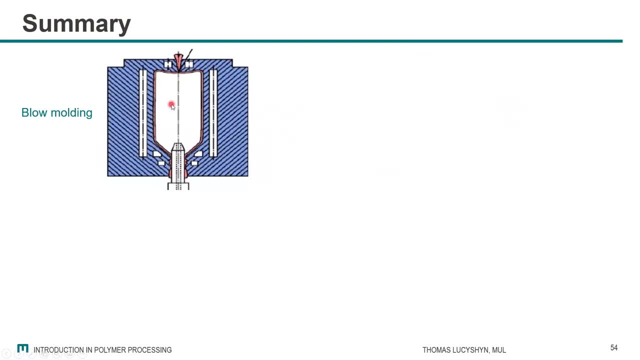 extruding a Spirit, which is then blown up and cooled down for a hollow body. I showed you the principle of thermoforming. you first need to produce a sheet or film of which is extruded, and then this film is further deformed in this thermoforming process. I showed you injection. molding for multi, for for mass prostu orders. I show you the principle of弧 etap木ang. I showed you injection molding for, not the, for much to make by floating. as I showed you injection molding for undergoing a sheet of " as well as amortization. 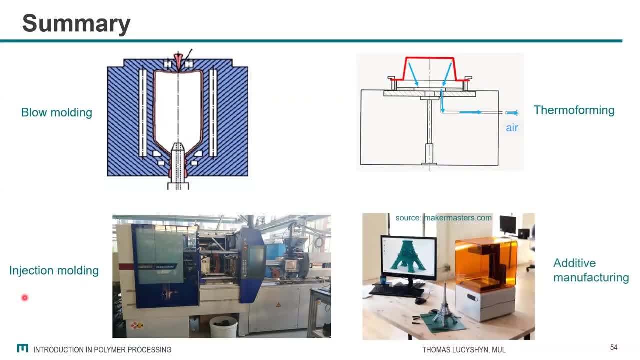 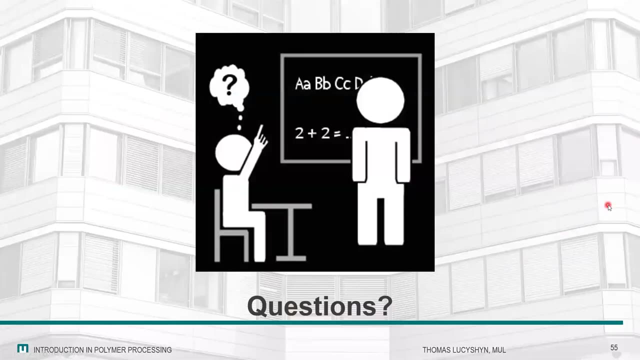 production of complex shaped single parts and also showed you the potential of additive manufacturing for individualized products and also fast development of products to get products very quickly from the process. So I want to thank you for your attention and I'm open for any questions from your side. 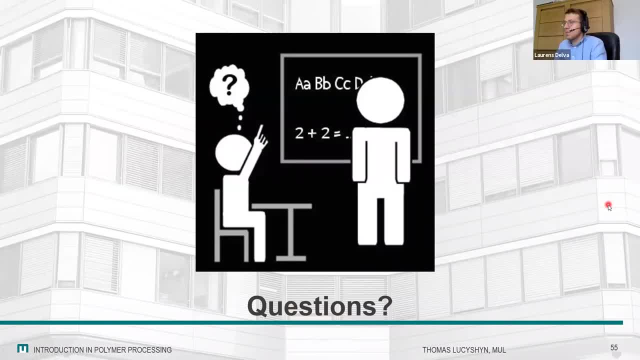 of course. Thanks a lot, Professor Luciccin. thank you for your very interesting presentation. just extremely clear and very comprehensive. I see one question in the chat from Alejandro who wants to know at which point in the polymer processing chain that typically additives are incorporated, so additives such as flame. 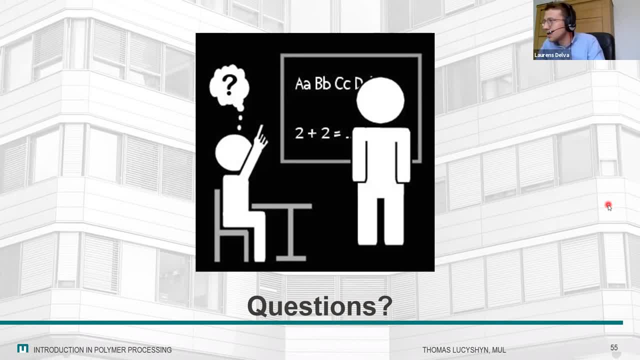 retardants and how these affect the process or even the properties of the material, And he also imagined that there are differences between thermoplastics and thermosets. So could you elaborate on that question? Yes, of course I'm sorry. I really basically I forgot in this processing stuff to really 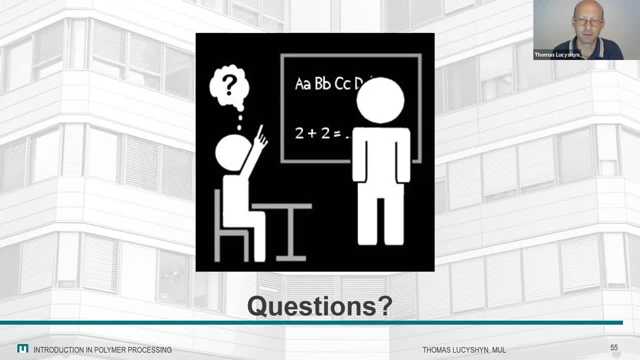 go about compounding. So I was rather focusing on those processing methods which are really resulting in a final product. but basically all this adding different fillers is happening in a different processing step which is before the real processing step. So this is called compounding. it's basically a mixing. 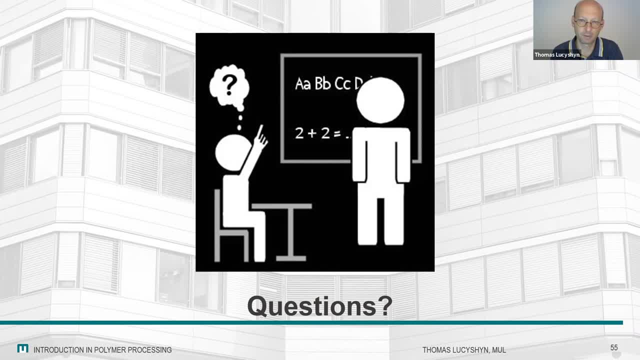 So we have an extruder with typical twin screws, so two screws inside the extruder, which are which have a very good mixing effect, And there we are adding different additives to the polymer and then in the end, the product of this process is basically pellets. 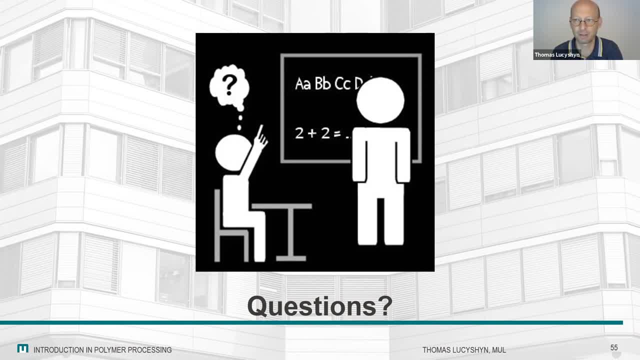 And these pellets are then used in conventional processes to produce the real product, And there we can add different additives: can be solid additives or particles, can be liquid additives and like flame retardants, so this can be added there. There is also an option to do it on a production machine. 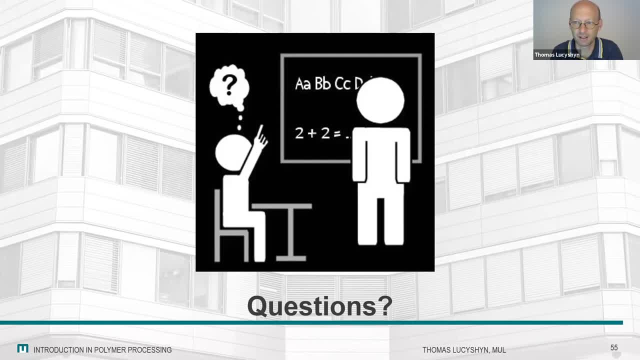 So you have kind of sort of master batches, as they are called. There have been compounded first into these master batches and then you can add those pellets to the other pellets You have. you can kind of dry mix them and put it into injection. injection warning machine. 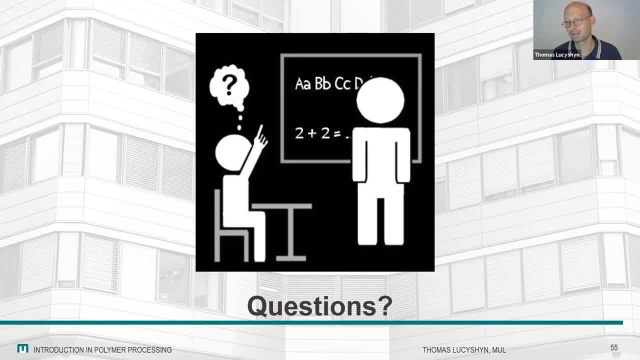 or extruder and then it will be kind of mixed together in this machine again. But still the the primarily process of primary process of mixing happens in a compounder which is a twin screw extruder, So two screws which have a very good mixing effect but are not intended to be used for. 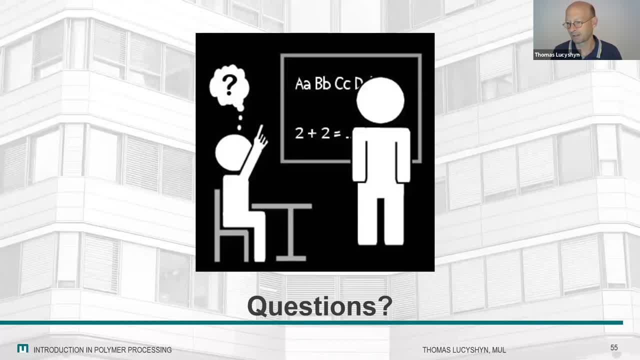 a production of films or whatever. And the effect of fillers is, of course, it changes the flow behavior. So if you add liquid fillers it might reduce the viscosity. If you add particles it might increase the viscosity. It all has an influence on the flow behavior. 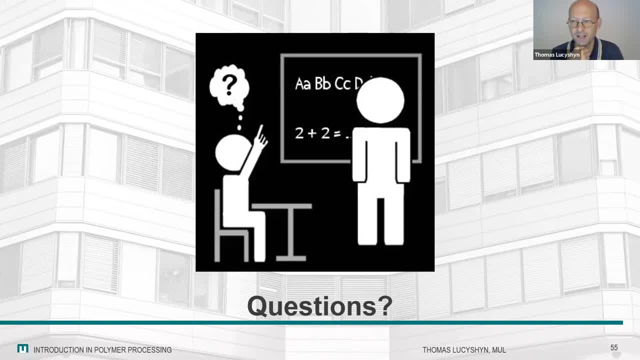 And in terms of the viewpoint of the processor, the best you would get is a material with very, very constant flow properties. That's also the challenge regarding recycling. As soon as we're getting mixtures of different materials- different materials, different flow behaviors- our machines are really optimized for good for, for homogeneous materials. 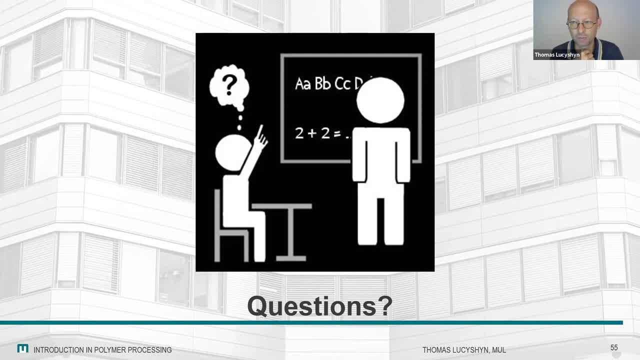 As soon as the material starts to be inhomogeneous, our processes will not run in the intended way. And there are two options: either you- you tailor your material, you optimize your material so that it remains constant, but that's very difficult for recycling materials- or the other. 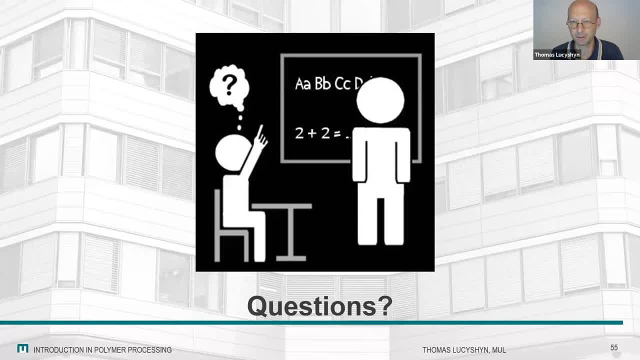 way would be: try to come to a flexible production method to to react onto the polymer properties, to react, to adapt Your process to the properties of the material. that would be the more intelligent way and something we're working on. also Is this question asked by that? 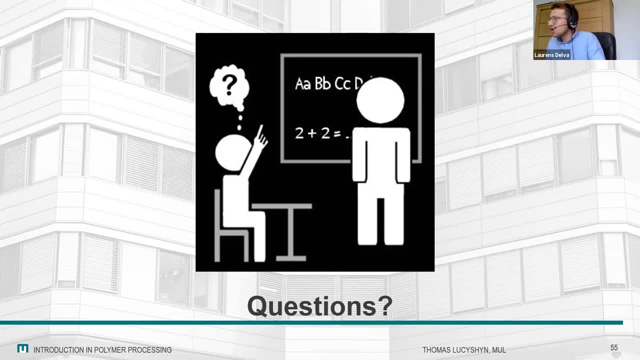 I believe so, Thank you. We also have a second question from Anton Cetus. She says that in the beginning you made the distinction between elastomers and thermoplastics. What about the reprocessing on the recycling of these, of thermoplastic elastomers? 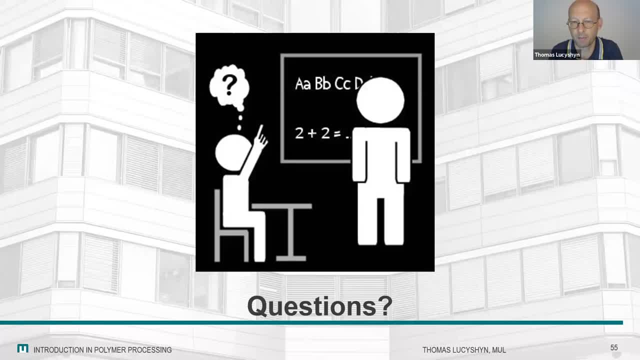 So, which is a special question, Yeah, Yeah, I would say thermoplastic elastomers. they are basically copolymers, So part of the chain are thermoplastic and parts are elastomer, And this can be I'm not sure. I'm not an expert, I must admit. so I'm not not focusing. 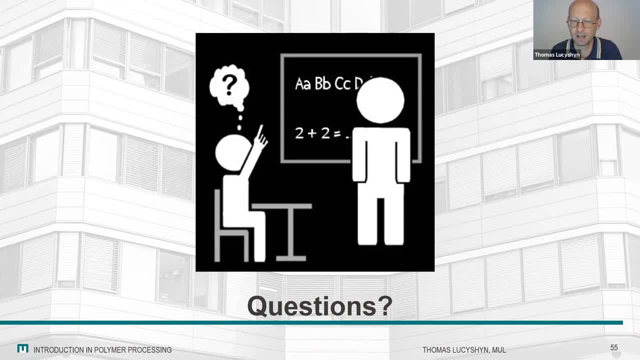 on this thermoplastic. You have not much experience on recycling of this, but I would say it should be possible to remelt them again, because the thermoplastic phase of this material is still able to remelt And so it should be shapeable again. 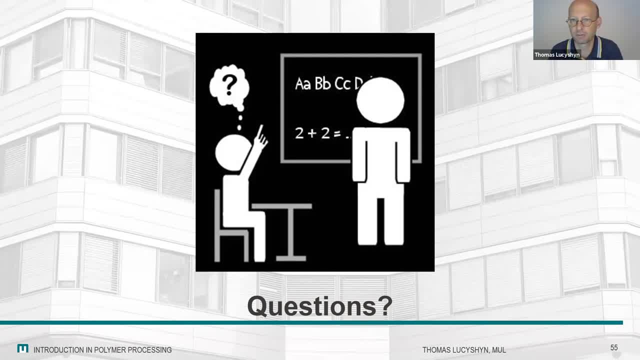 So I would expect that this should be possible to to react So to to conventionally do mechanical recycling. that Okay, Thank you. I see next question popping up from from someone in the audience who is wondering if the additives, if they are mixed with a polymer material not to be used like coating outside. 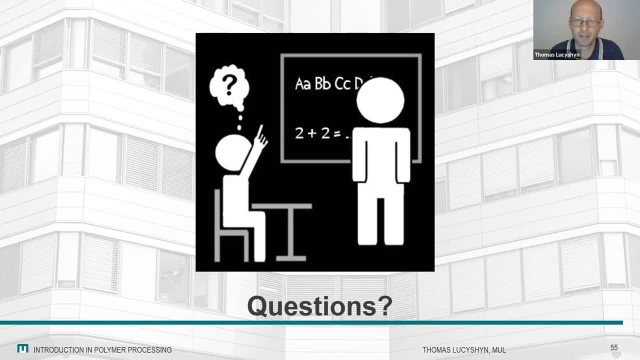 Normally not, So you normally put the additives into the bulk material and then it's extruded, So it's almost like coating. Yeah, Yeah, So it's not a homogeneous distribution of this additives all everywhere in the material, So it's not like a coating. 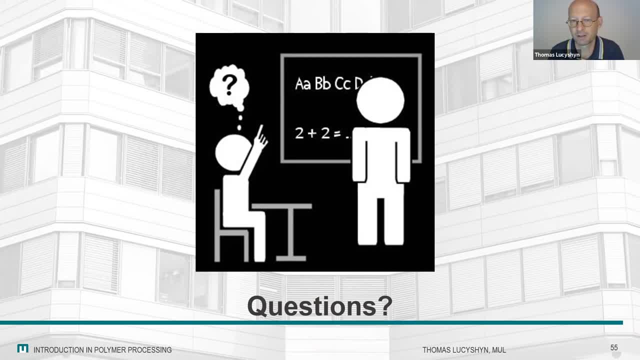 It can happen, though, that during processing or also in the use, that they're diffusing to the surface and then form some layers which you don't want, or you want them to have some protective effects. So it depends on your application, but typically they're distributed all over the material. 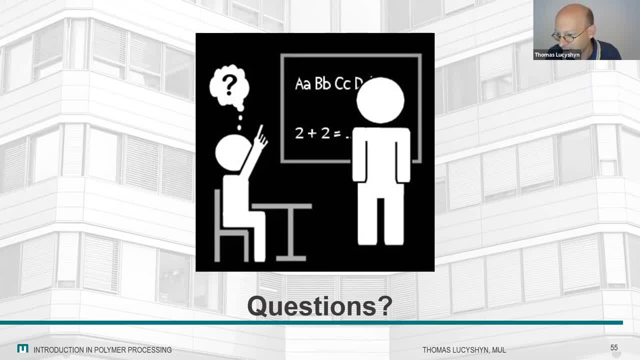 in the extrusion process. Thank you, And next question from Tiago. So he points out that VOCs or other compounds are mainly formed during the extrusion process at the at high temperatures, And he wonders during recycling processes, if, for example, washing procedures can be. 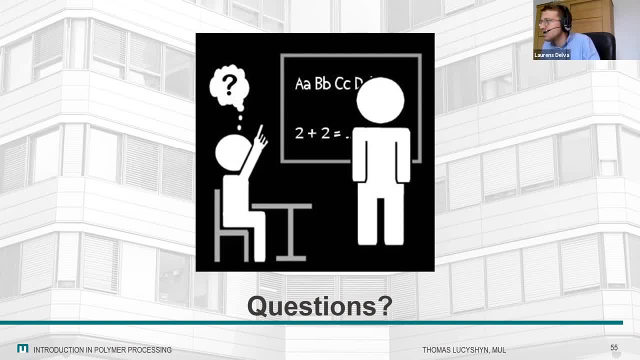 applied in order to diminish that. So is it possible to use washing, cleaning up processes after extrusion? I would say, if you, if you have a look at the final product, so if you're extruding a film again, or or. 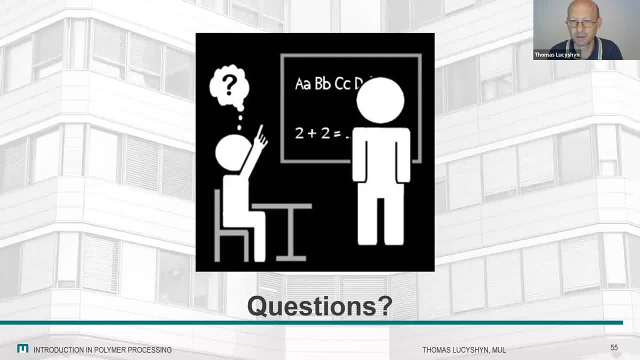 Or a pipe. the problem is that there there's the relation between surface and volume is not the best, So you only have, you have a material, a product, you with the washing process, you cannot reach into the product itself. So I'm not sure if the effectiveness is so high. 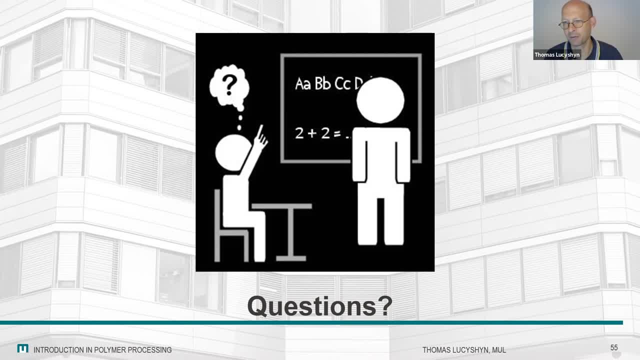 So if you applying washing in the pellet state, you have a better ratio of surface to volume and therefore maybe you can easier extract some, some orders or something. But in the final product, if it's a very compact part for injection molding for example, there 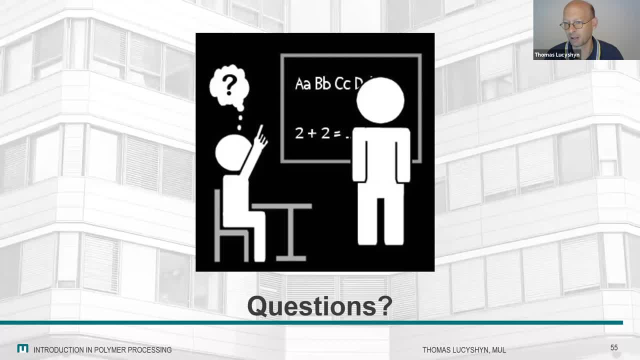 will not be too much surface, But you can extract something from it. So I would say it's more in the- maybe in the stage after compounding and you have pellets before you go for the real production process. this would be a good point where you could. 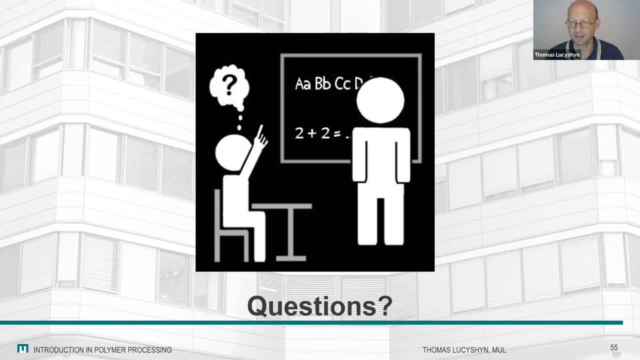 maybe add some washing process, but in the final product I'm afraid it's not so effective to do some washing of the product So typically. if I may add as well on that point that during compounding so they typically will also apply some Vacuum there. 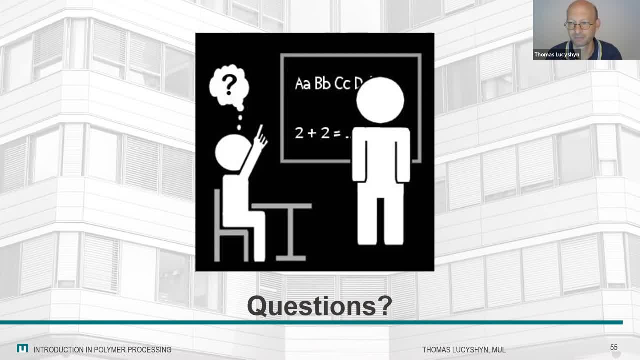 Yeah, Degassing, Degassing indeed, And I think it's something to to try to remove these compounds as much as possible. Okay, Do we have any other question or point of discussion? We still have five minutes before the before the break. 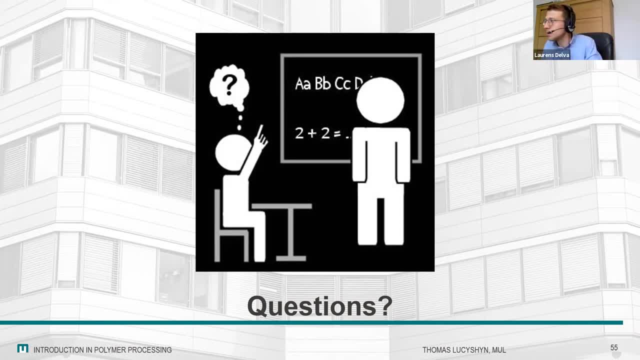 So you could put on your microphone if you would have some. Okay, There's one question regarding degradation. That's the point I mentioned at the beginning. So we have this compromise between: we need a sufficiently high temperature that we are able to melt it and to shape it And, on the other hand, we know exactly that each contact 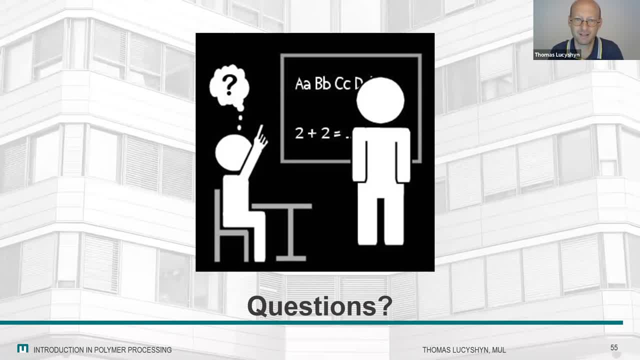 with heat damages the material. So what is basically done is there are additives which are added to the material with the only purpose that it survives processing. So not for application, so that's another topic- but really additives with the only purpose that they survive the 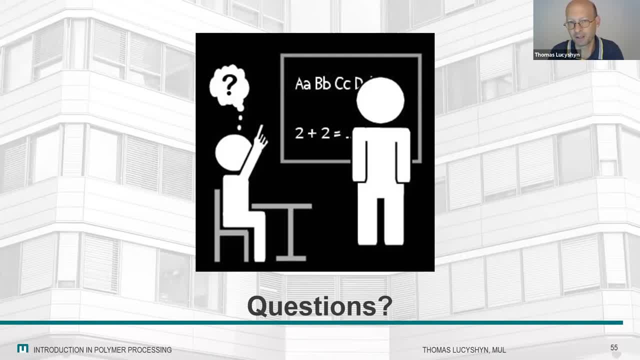 processing step. So this is really a topic. and if you are recycling materials, so each processing step they are running through, they're damaged in a certain amount. So that means we cannot do this, although it sounds like very promising. You have thermoplastics. 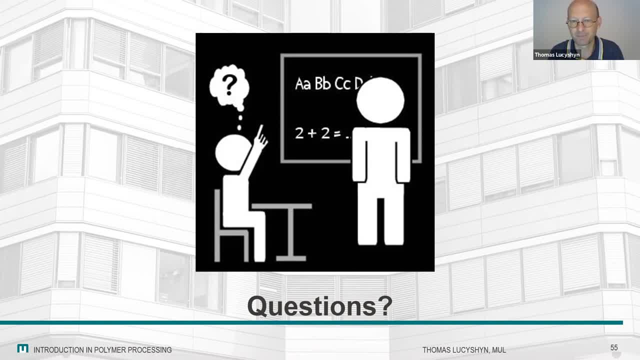 you can always remelt it and reshape it, but this is really limited by the damaging which you're doing to the material. every processing step There will be some damaging, but you in the first process step maybe it doesn't make any difference. all those additives are consumed. 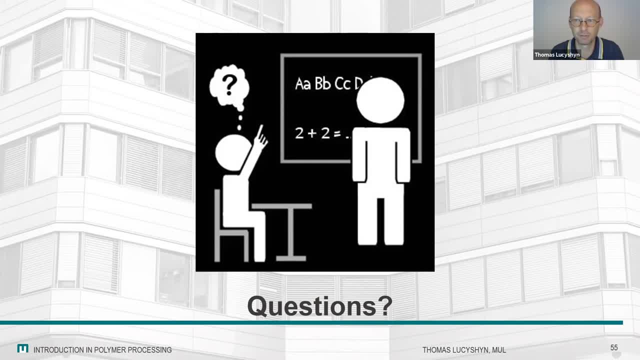 in this step, but then in the next step these additives are consumed, and then that's the problem, where the problem starts. if you add this again to the processing step, there might be more degradation. so what you can basically do is, before you're doing recycling, you get recycling material. 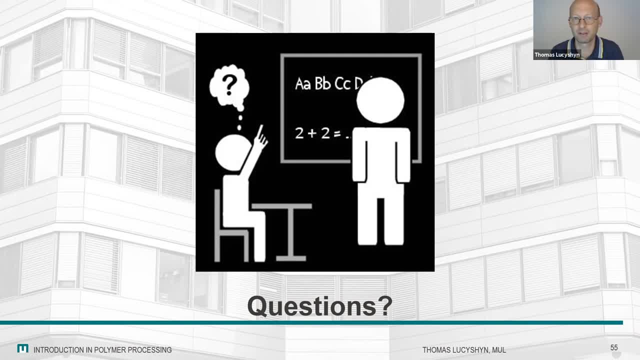 you still have to add another type of, or you have to add additives so that you can really process them again. so it's like upgrading them or this additivation which is necessary to, yeah, to enhance the properties again. yes, that's also a question from namarata. um, so, indeed, she. 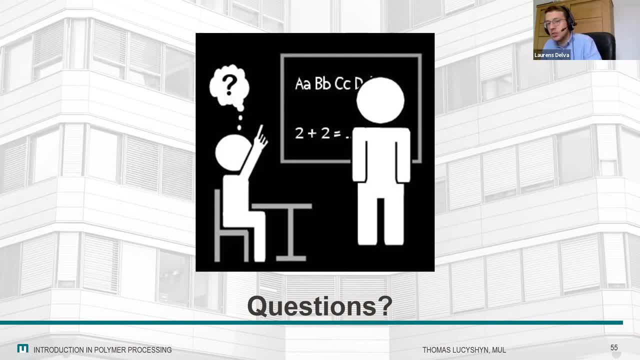 also mentioned that that when you're degrading your polymer change, that you actually are downgrading um, and that she also wonders if you could, in the recycling method, that you could um get these properties back to a certain level? um, and she asked if you could highlight what the 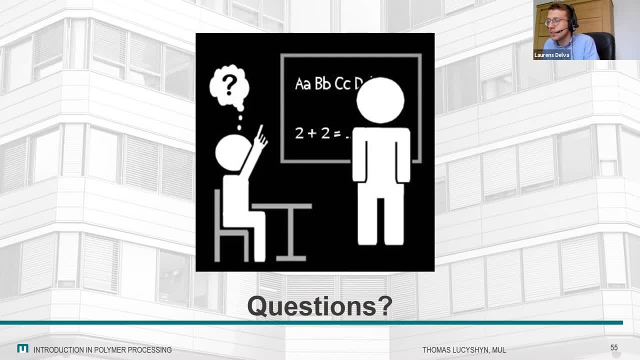 difference between these two methods would be- but i think you you answered that in your in your previous uh question- basically, add additives. i will tell a little bit also in tomorrow's lecture about this, and that's really so. just taking the recycle material and put it into the processing machine. 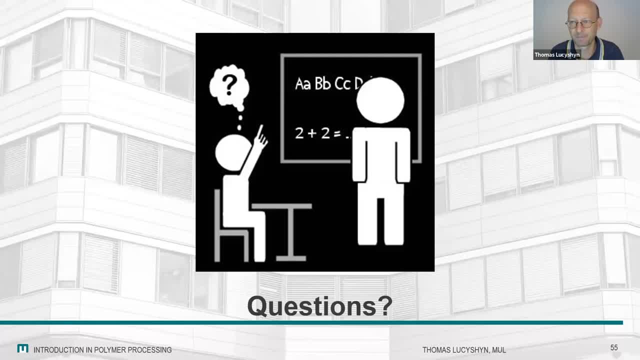 will probably not work quite well. otherwise, you really have this downgrading which you have this, this downcycling which we don't want, we don't. we also did a project where we used polyoxymethylene for a technical product, which is quite challenging and, in the end, by editing some, 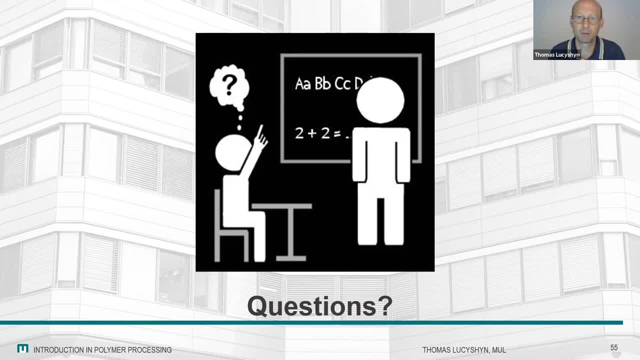 materials, enhancing their thermal resistance and also mechanical properties. we ended up in really producing a product which is of the same quality or sufficient quality for the product, but it's of pure recycling material and this was really a nice, nice result. i will show you this example tomorrow, also in the recycling lecture, perhaps last question, uh, from roberto. why can't thermostats be mechanically recycled? yeah, the problem is that you cannot reshape the, so there, you can grind them. you have some, you can cut it down to small pieces, but you cannot re-melt them. so they are not deformable. and once those bondings are established, especially for 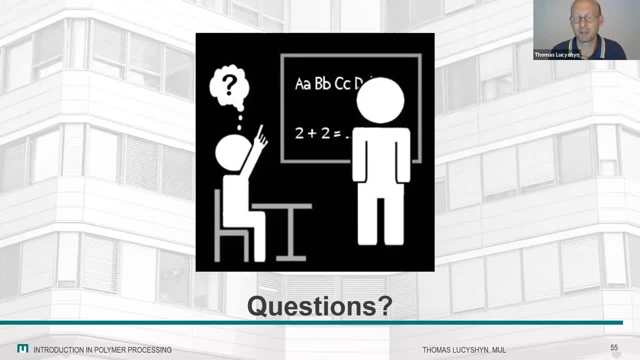 these durameres? uh, they are not reshapable anymore, because that's the principle for thermoplastics: you always have those entangled structures, you melt it and then it becomes movable, flowable, and if you have these fixed bonds, once you have these bonds established, the shape is given and